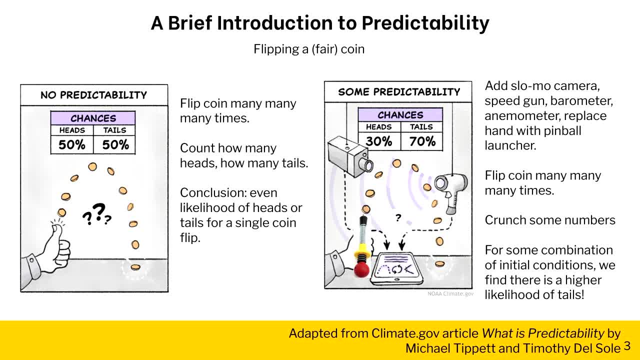 system. what if, I, you know, add a slow motion camera, a speed gun, a barometer, an anemometer? what if, you know, we take this metaphor to the absolute limit and we replace the hand that's flipping the coin with like a pinball launcher, and we 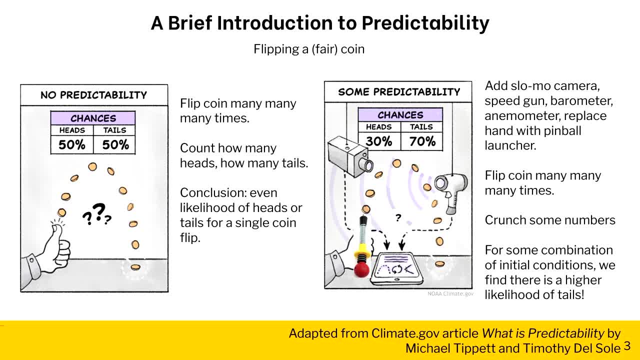 need. so we know exactly how much force we're putting on and we flip our coin again and then we sort of crunch our numbers and we find that for some combinations of initial conditions- so, for example, you know if tails is facing up when we start- if we pull our pinball launcher back an exact one centimeter, we 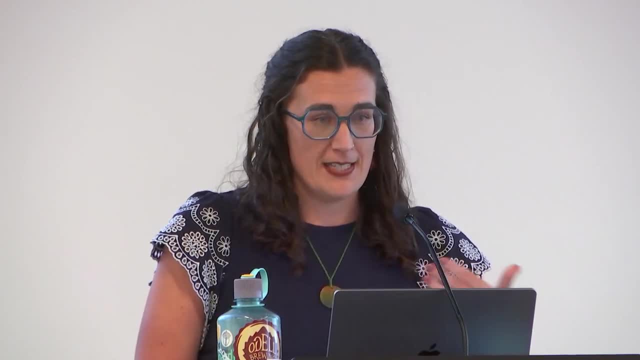 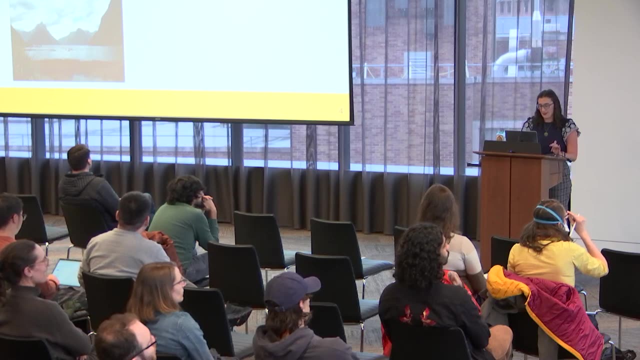 might find that there's a higher likelihood of tails. so we found that we, our system, does have predictability based on the initial conditions. so now I'm going to go through a climate example of this. so you know, I'm wanting to go hiking to my home and I'm going to go to the beach and I'm going to go. 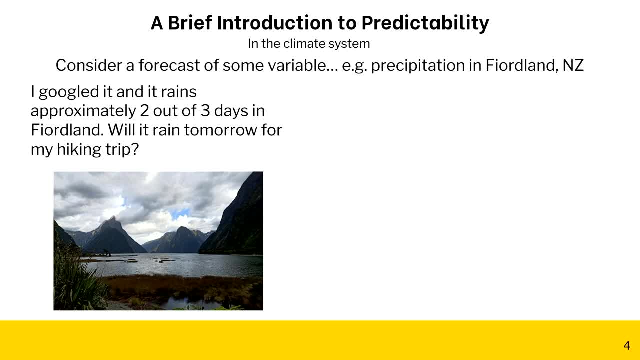 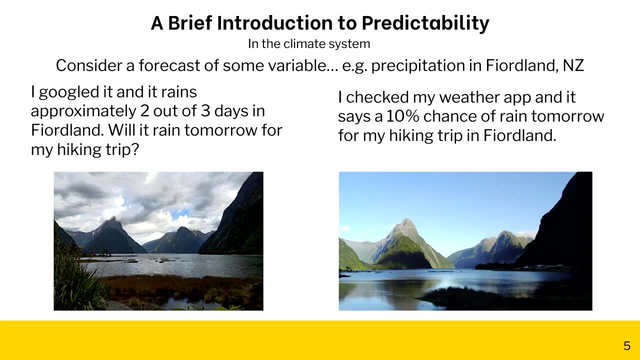 trekking tomorrow in Fiordland in New Zealand. so I googled it and it rains. you know every. you know two out of three days in Fiordland. so you might naively think, oh, there's, like you know, 66% chance of it raining for my hiking trip. 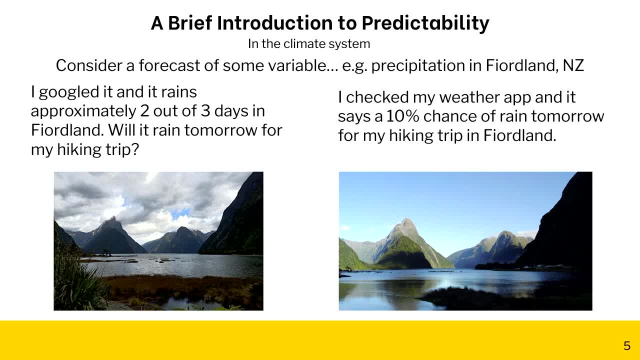 tomorrow. however, I looked at my weather app and it says: actually, there's a 10% chance of it raining for my hiking trip in Fiordland. so what's going on there? well, we have the initial conditions in the system actually allow us to know that there's a 10% chance of rain, so that the evolution of the system only 10%. 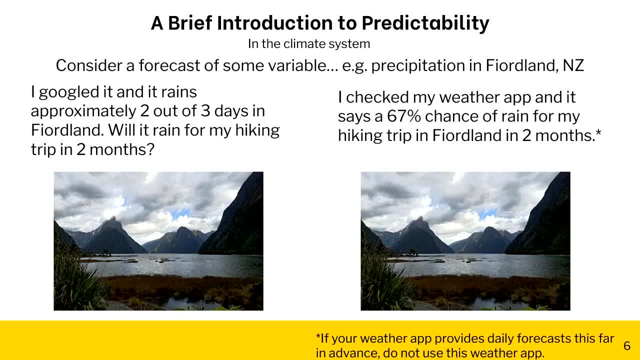 of cases, will it be raining tomorrow? Okay, but what about? I look in my weather app for my hiking trip in two months' time? So now, my weather app now says that there's a 67% chance of rain for my hiking trip. 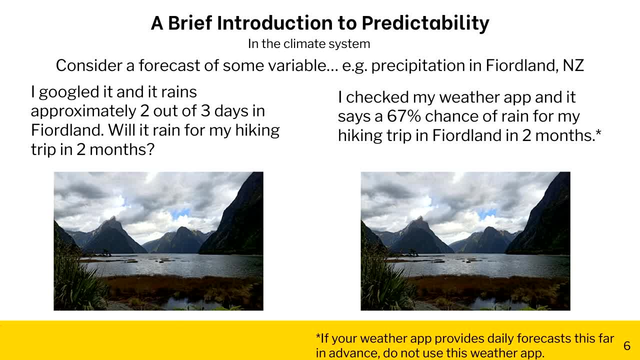 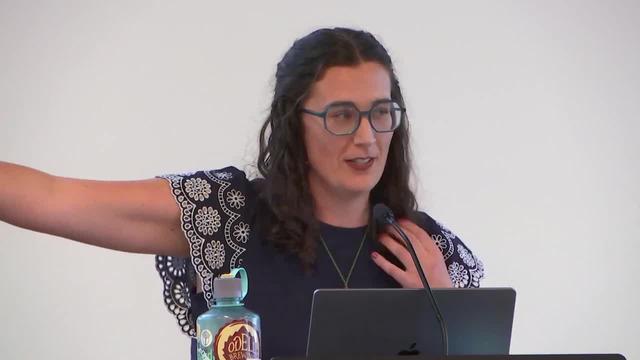 And this is because at this lead time there is no skill from our initial condition, so the memory of the initial conditions in the system is lost. And I've included a little bit of a note about if your weather app is providing daily weather forecasts, in two months' time you probably shouldn't be using this weather app because 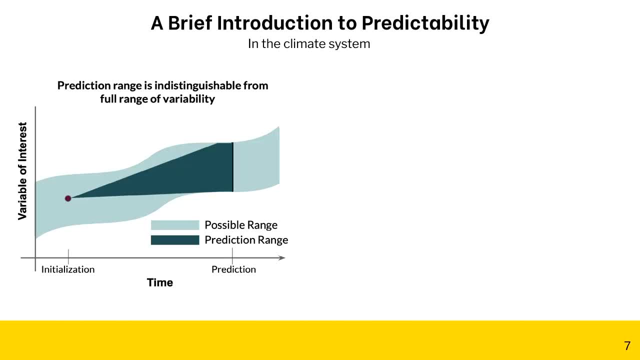 they really can't do much better than climatology anyway. So now I'm going to formalise this in a schematic. So along the x-axis here we have time from the initialisation of some forecast to our prediction time, And on the y-axis is our variable of interest. 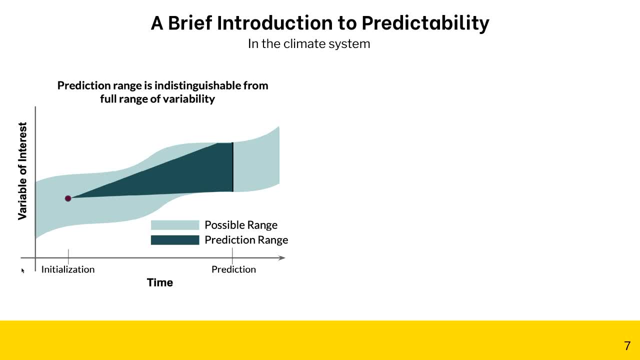 This could be temperature or precipitation And in this example, here we have our initial state and, when we look at our forecast, the possible range. so the prediction range is indistinguishable from this full range, the possible range, what we'll call climatology. 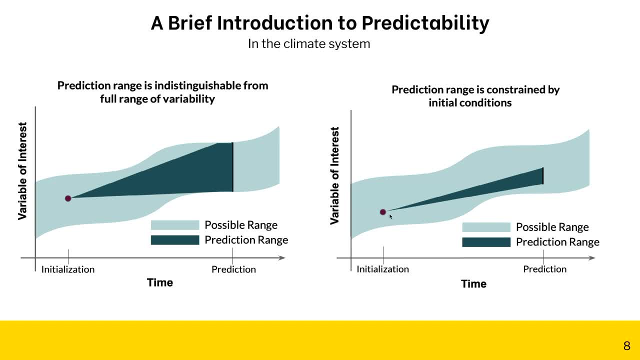 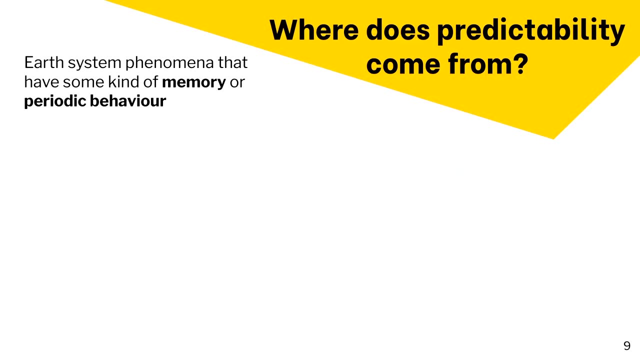 However, we might find for a different initial state, maybe a slightly lower anomaly- that by the time we make our prediction the prediction range is constrained by the initial condition. So we have a smaller outcome range than the full possible range. So this initial condition provides us some predictability of the system. 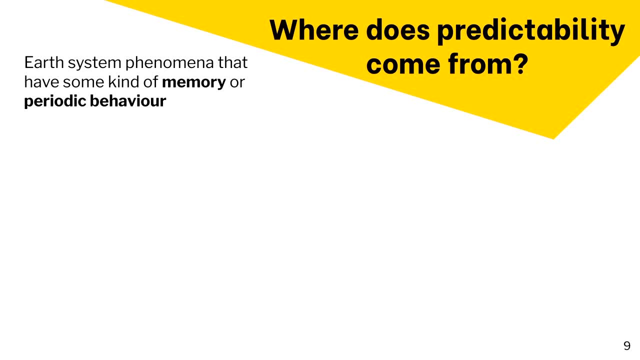 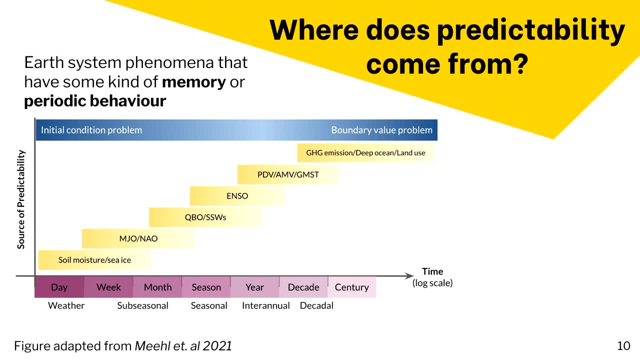 So where does predictability of this kind come from? So I'm going to make a statement that it comes from a phenomena that have some kind of memory or periodic behaviour, and this is a figure from a study that sort of looked at predictability across timescales. 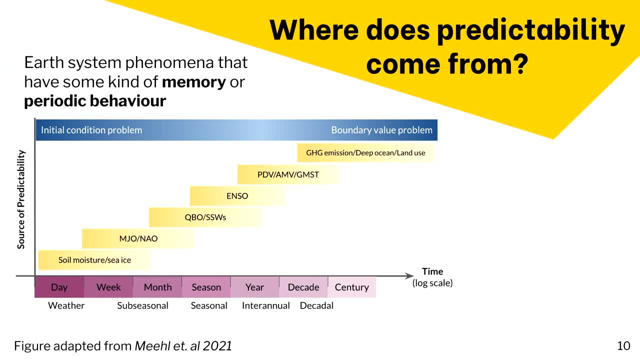 And on the x-axis we're looking at the timescale from weather, so the very short timescales out to sort of century timescales, And then we're sort of going up and listing all our sources of predictability from the initial condition problem, so making sure we get our initial conditions correct to 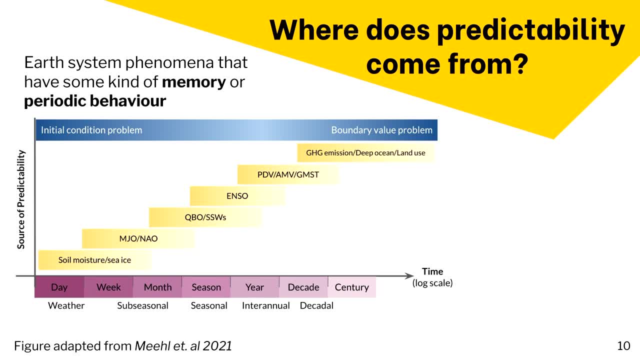 the boundary value problem, where it's really important that we're getting the forcings in the system. And I'm really interested on this timescale here, this sort of inter-annual to decadal timescale where we're pushing the limit over our initial condition predictability. 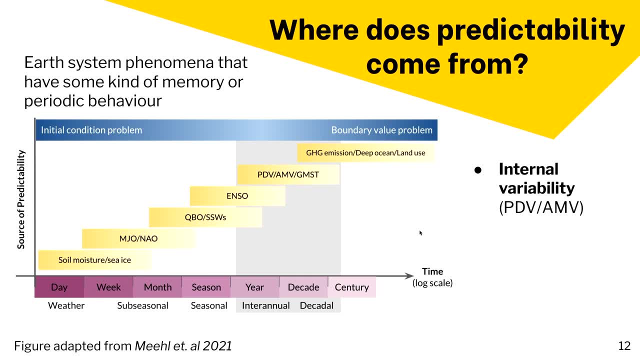 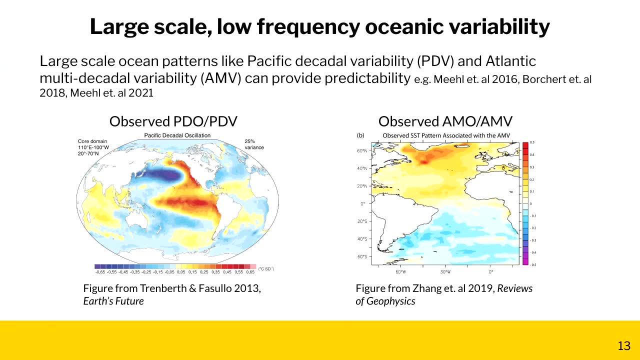 And so in particular I'm interested in these two acronyms here: PDV and AMV. they stand for Pacific Decadal Variability and Atlantic Multi-Decadal Variability. So these are forms of large-scale low-frequency oceanic variability, and I've included two. 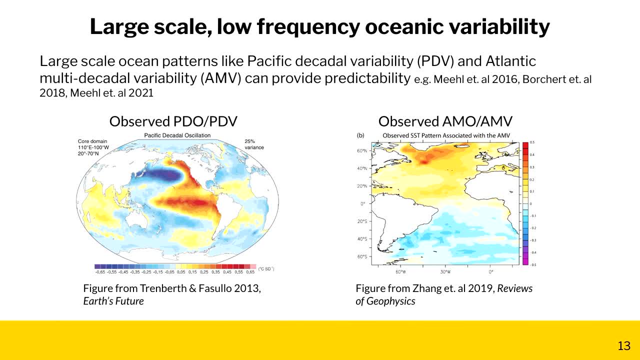 figures of their corresponding characteristic patterns, and the real takeaway here is that these are sort of large, you know they span the entire meridional extent of the ocean patterns that describe where heat is stored And they sort of propagate on these decadal to multi-decadal timescales. 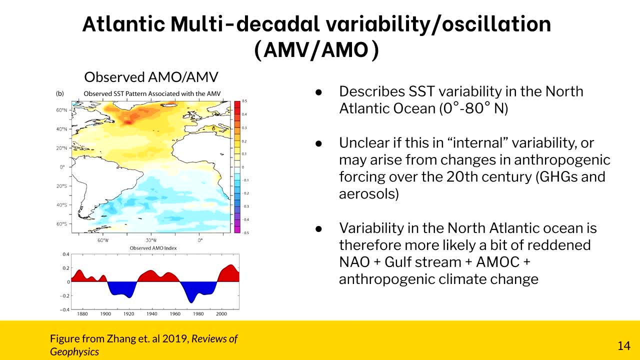 So Atlantic Multi-Decadal Variability or oscillation, depending on you know who you are, where you come from. you might choose AMV, AMO, but this describes sea surface temperature variability, or SST variability, in the North Atlantic Ocean. 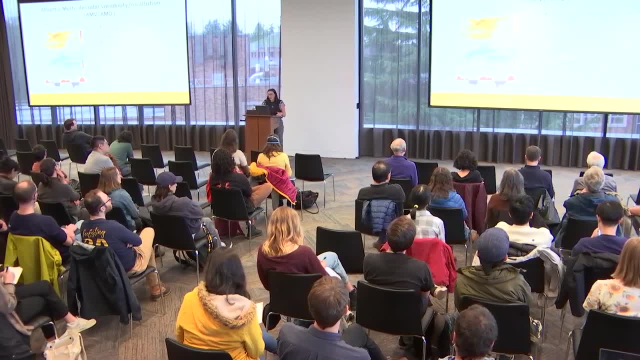 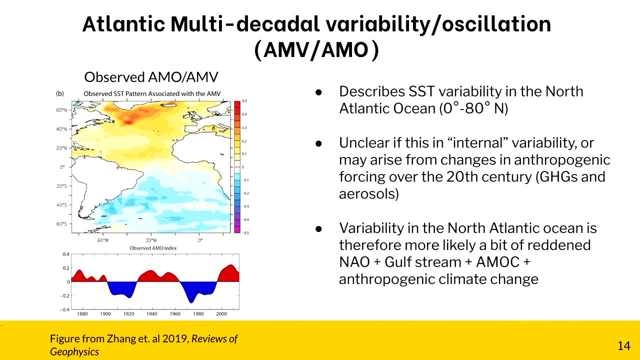 And it's unclear if this is actually fully due to internal variability or some of the variability may arise from changes in anthropogenic forcing over the 20th century. So no matter sort of where you fall on this, it is, I think, fairly clear that there has 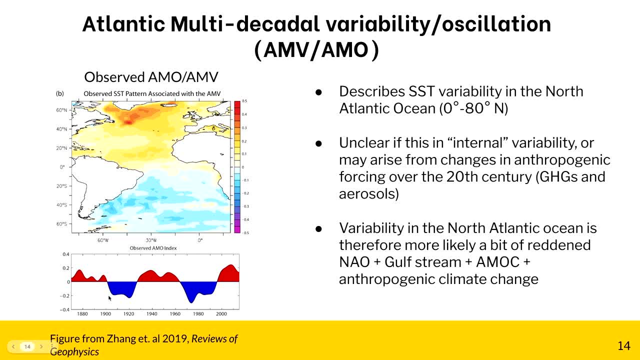 been some kind of inter-decadal variability in the Atlantic Ocean, and this is shown in this time series. Here is the index of this variability, And so it's thought to be sort of a combination of some North Atlantic oscillation, so NAO. 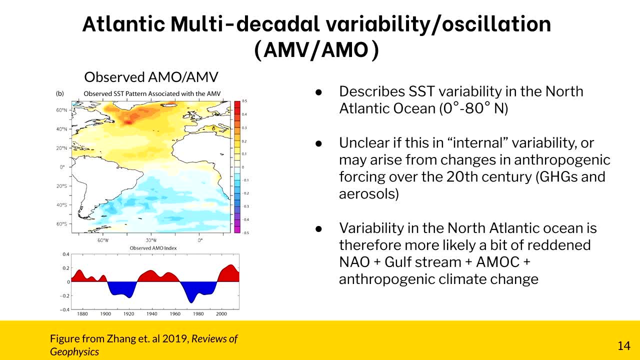 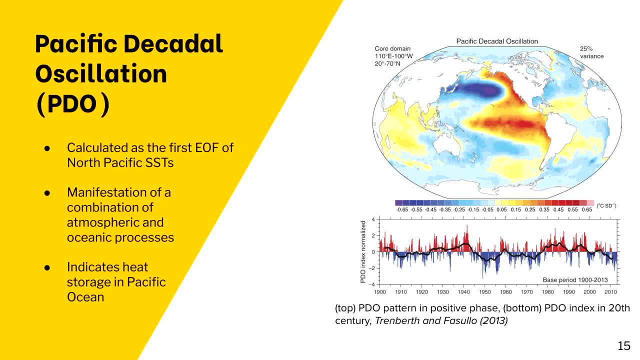 plus some Gulf Stream variability, plus some AMOC, so ocean overturning circulation, plus a bit of anthropogenic climate change. When and where each of these matter is still up for debate. I'm also interested in this. I think this is a really interesting topic. 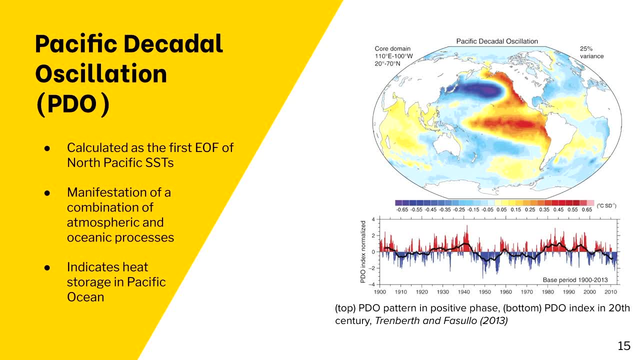 I think this is a really interesting topic. I'm interested in the Pacific-Decadal Oscillation or Pacific-Decadal Variability PDO-PDV, And this is calculated as the first EOF. so first empirical orthogonal function of North Pacific sea surface temperatures. 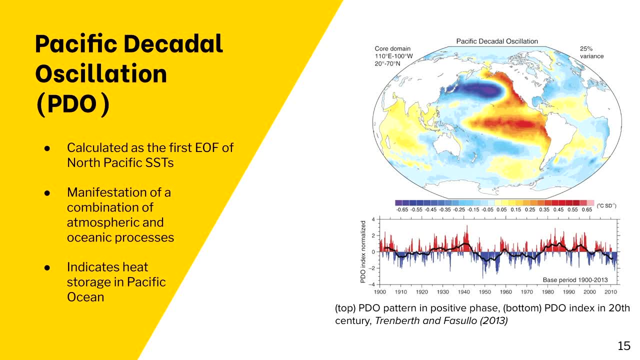 Like AMV, it's thought to be a manifestation of a combination of atmospheric processes and again it indicates the heat storage in the Pacific Ocean. Once again along, this panel here shows the time scale of the Pacific. sorry, the time. 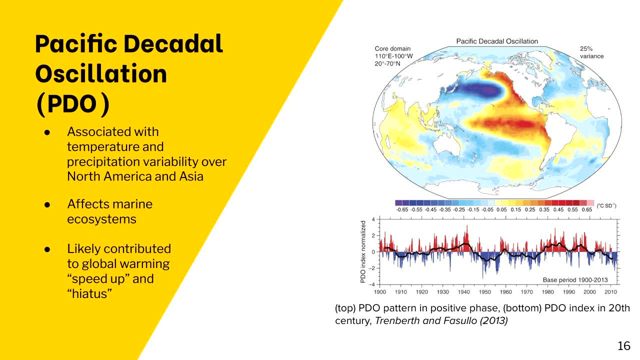 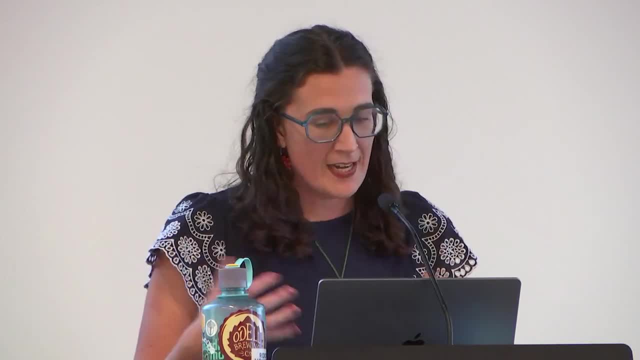 series of the Pacific-Decadal Oscillation in the 20th century. So interesting with the PDO is it's associated with temperature and precipitation variability over North America, so if it's in a certain state the precipitation might be a little bit anomalously high over, for example, the West Coast. 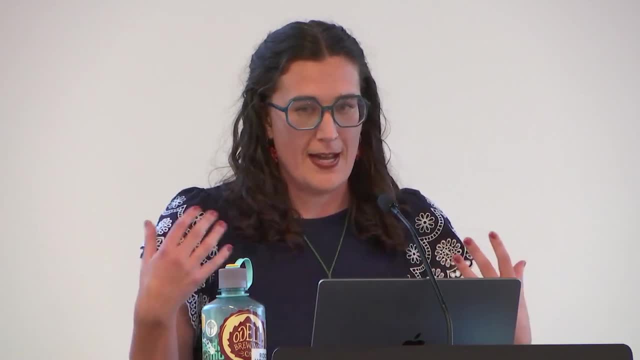 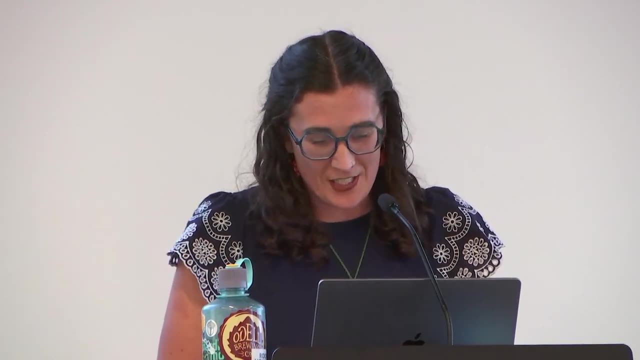 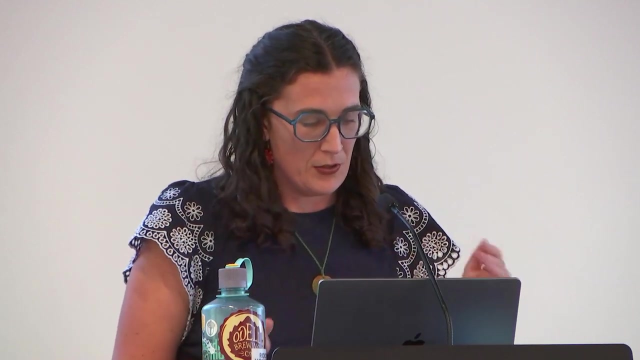 It also affects marine ecosystems. so interestingly, the PDO was discovered by people, I think at UW, actually looking at fish populations, And this pattern is so large that it's likely contributed to modulations in the rate of global warming. So it's thought to have contributed to sort of a speed up of global warming around the 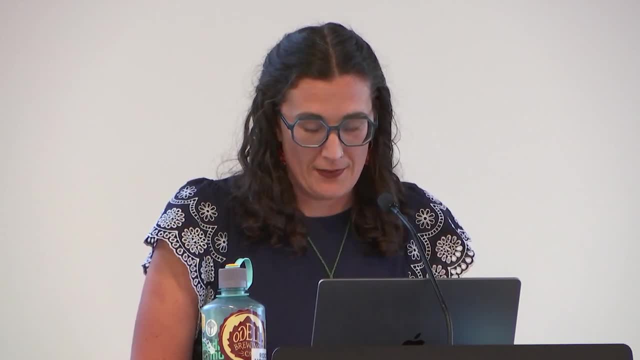 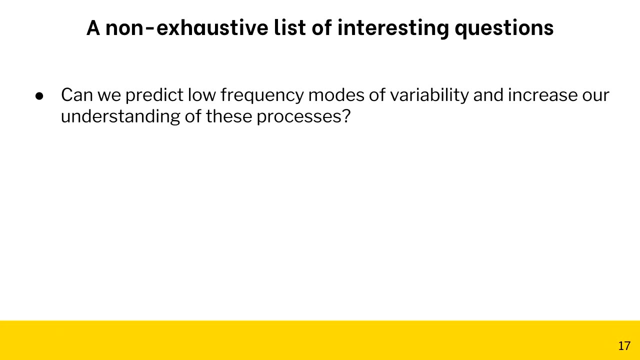 1980s and then also the hiatus period around the early 2000s. So I sort of I'm calling this a non-exhaustive list of interesting questions, because I you know there are so many interesting questions in the world, but these are the ones that. 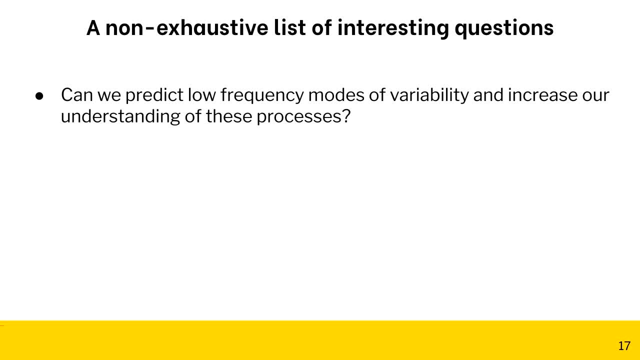 I'm interested in. Can we predict low frequency modes of variability and increase our understanding of these processes? Can we identify states of enhanced predictability- so this is going back to before- these states that are more likely to have predictable outcomes and their contributing mechanisms? 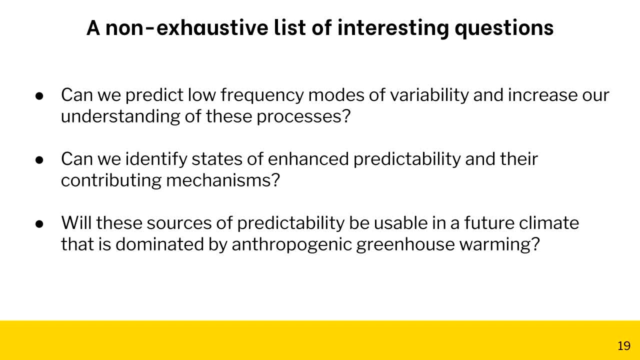 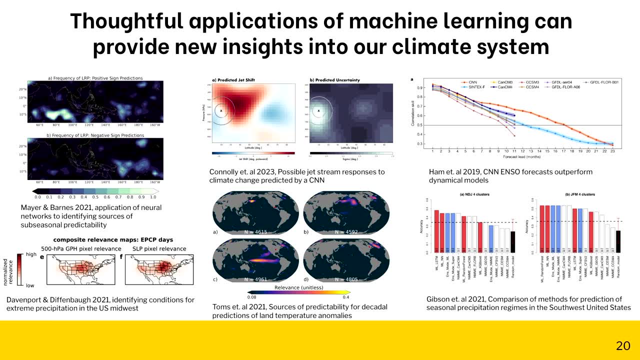 And, lastly, what does predictability look like in a future climate that's dominated by anthropogenic greenhouse gas warming? And I'm going to use machine learning for my work and I'm not going to go through all these studies here, but I you know these are some really lovely machine learning papers. 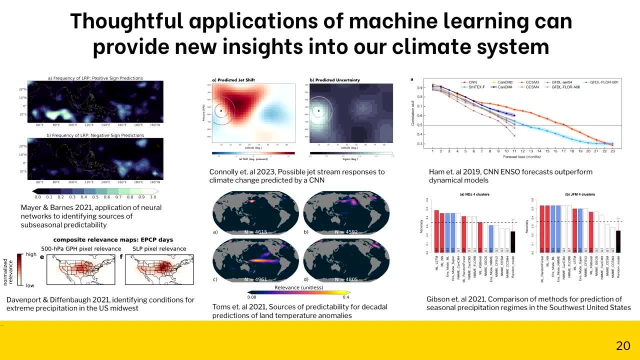 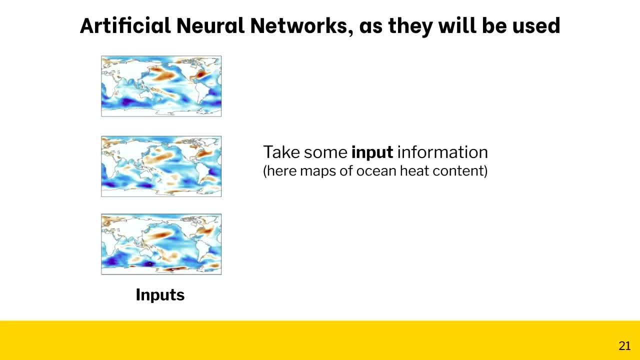 in climate and atmospheric science, which have shown that we've been able to make some really good insights in recent years using these new tools. So I'm going to use in this first study an artificial neural network and I'm going to go through briefly how this works. 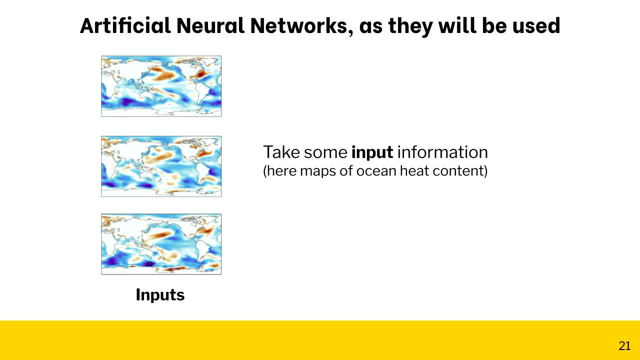 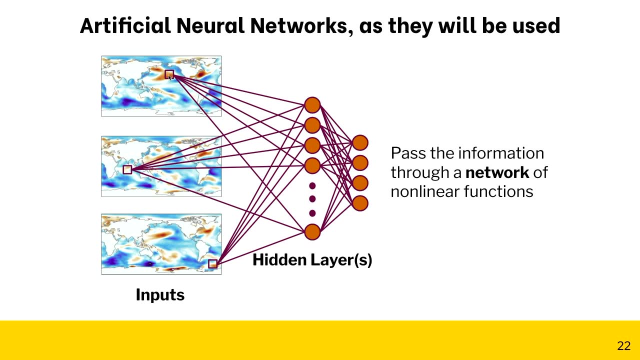 So we're going to take some input information. so here it's going to be maps of ocean heat content and we're going to connect them to our neural network, which is a network of non-linear functions, So we can consider each of these points on these maps here as being connected to each. 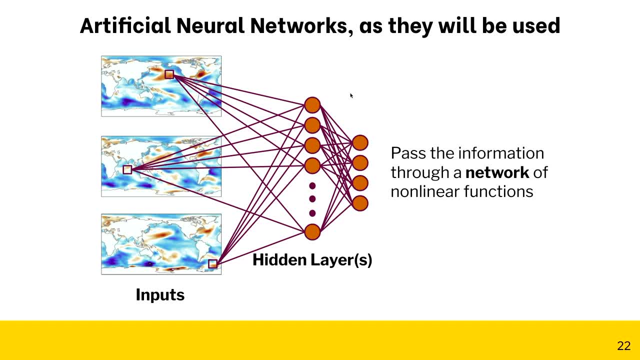 of these nodes, Each connection represents a weight, and then when we get to these, each of these nodes, we add a bias term and then surround that, We surround that whole thing with an activation function which sort of governs if or how. 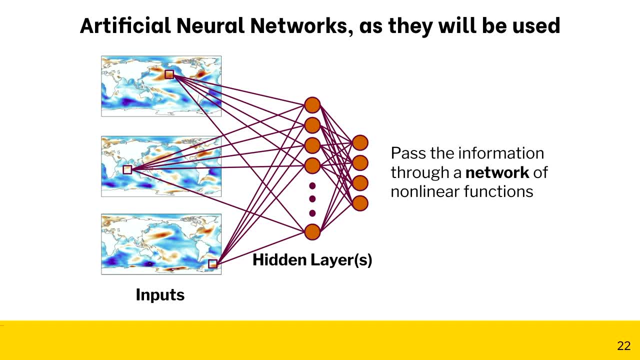 much information is passed forward into the next layer. So you can see, we have, you know, this layer of nodes where we're sort of deciding how much information to pass forward, and then we can add another layer, a weight on all of these, another bias, more activation function. 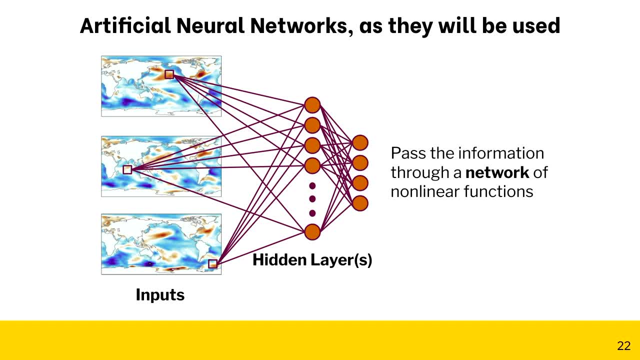 So we can build up these sort of nests of network, I guess would be the word- of non-linear functions. So this is a neural network, and then our output will be a prediction of something which should probably be related to the input. 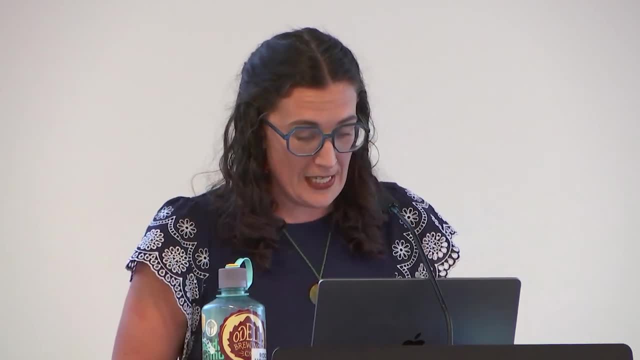 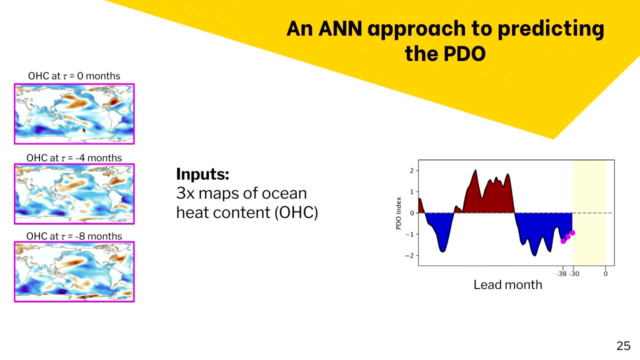 So I'm going to go through an example of using ANNs to predict the PDO. So, like this previous example, I'm going to input maps of ocean heat content, lagged by four-month intervals, into a very, very simple artificial neural network. 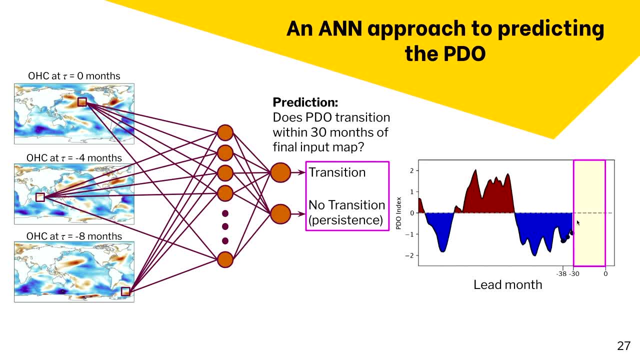 And then our prediction problem is going to be asking this neural network, will the PDO change phase? So will it switch sign in the next 30-month period? So you know, if this is our input period, these three black dots, what's going to have. 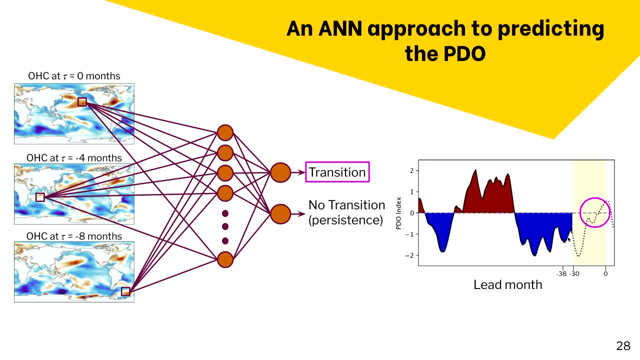 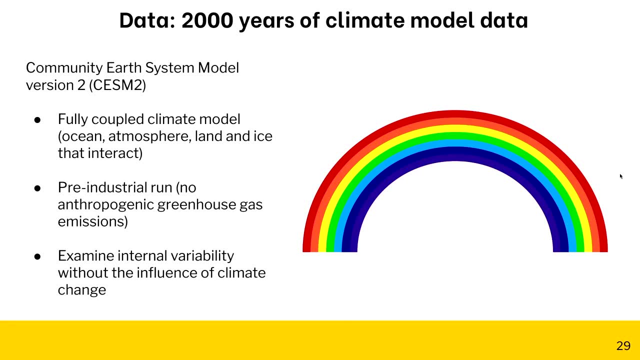 to happen within this pink window here. So an example could be following this dotted line. we cross through zero here, so we do change sign, so a correct prediction here would be transition. For this study, I used 2,000 years of climate model data from the Community Earth System. 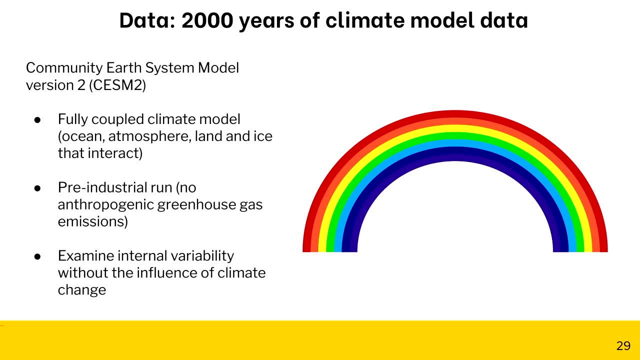 Model Version 2, so CESM2.. This is a fully coupled climate model with you know, ocean, atmosphere, land and ice. It's a pre-industrial control run, so there's no anthropogenic greenhouse gas emissions, And the reason we use this is it allows us to examine internal variability without the 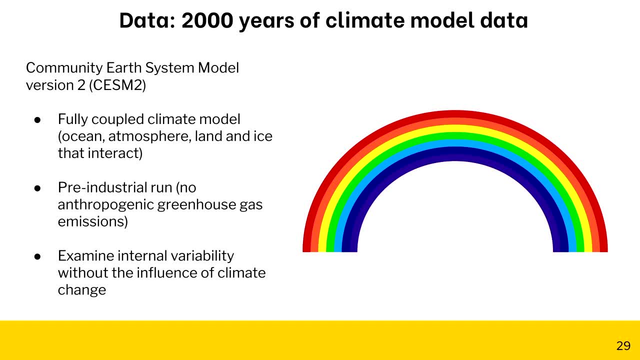 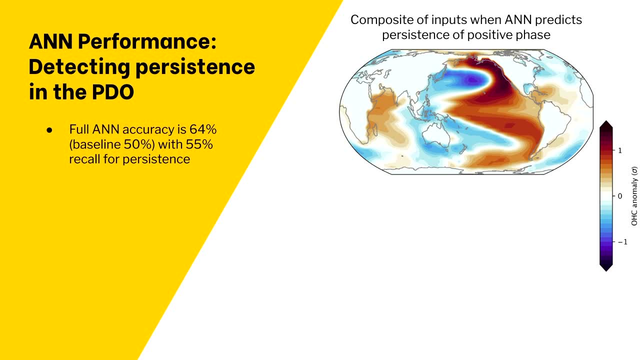 influence of climate change. So I call this rainbow world because you know, humans aren't there to mess everything up. So I'm going to go through some sort of basic results. So first of all I'm looking at predicting persistence in the PDO. 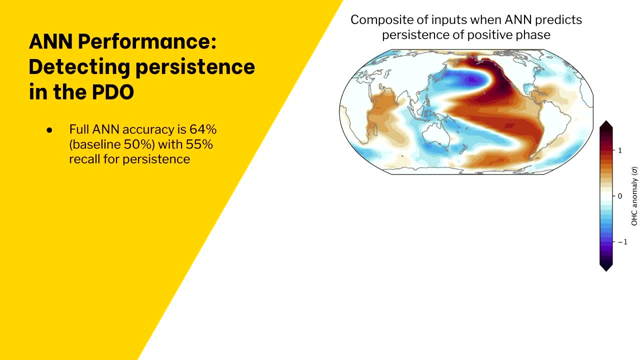 So this is saying the sign of the PDO does not change. so we're looking at persistence of the positive phase. So this is a composite of the correct input maps for a positive to positive persistence. And this is a composite 30 months later, not super interesting. the PDO didn't change because 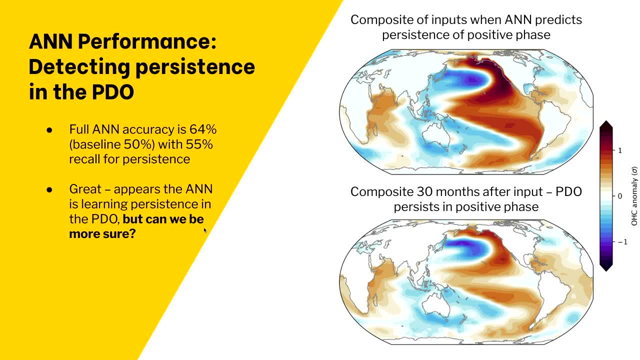 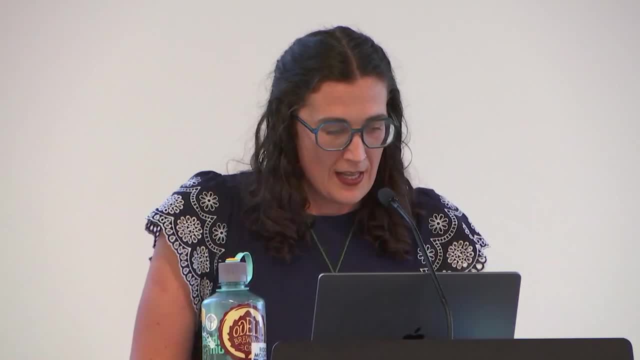 you know it's a positive. So it appears that the ANN is learning persistence in the PDO, but can we be more sure about why our neural network has made its decisions? So I'm going to use an explainability technique, an explainable AI technique called layer-wise. 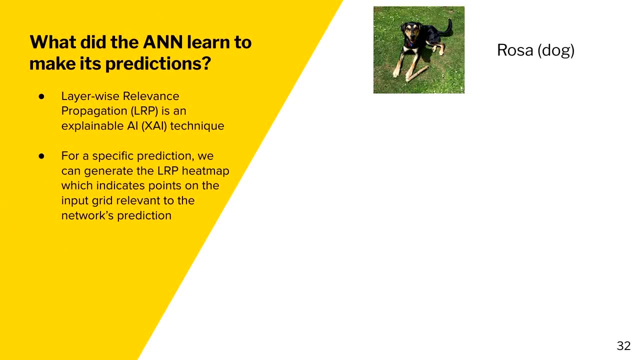 relevance propagation, or LRP. So for a specific prediction, we can use LRP to generate a heat map which will indicate points on the input map that are relevant to a network's prediction. So, for example, we could take this picture of Rosa the dog and put it into an online 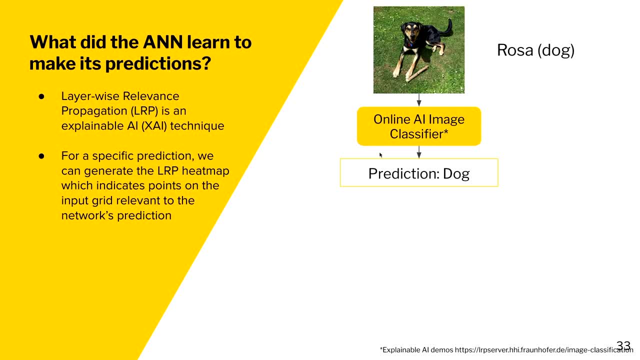 image classifier Which gives us a prediction of dog. So good job. online you did it And then apply LRP to our prediction to get a heat map of the points that were relevant to the prediction So you can see here for Rosa, they have indicated her eyebrows and her ears a little bit of. 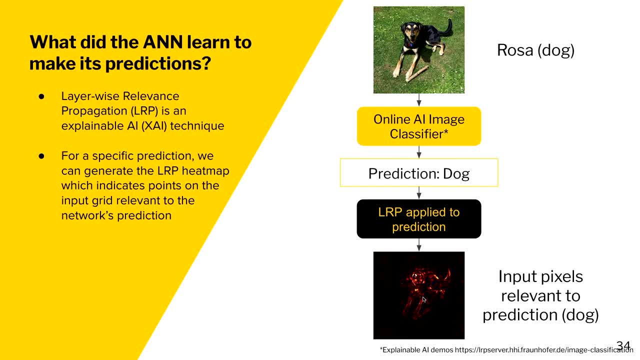 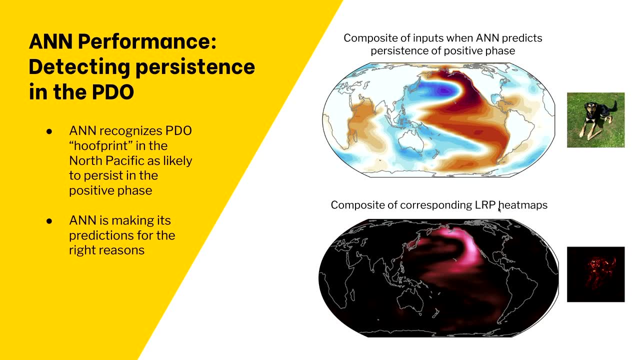 her tail and also her dog tags. They've noticed that. you know, dog tag means dog. So, in the context of this problem that I was looking at before, this is our composite of inputs. So this is our persistence inputs. 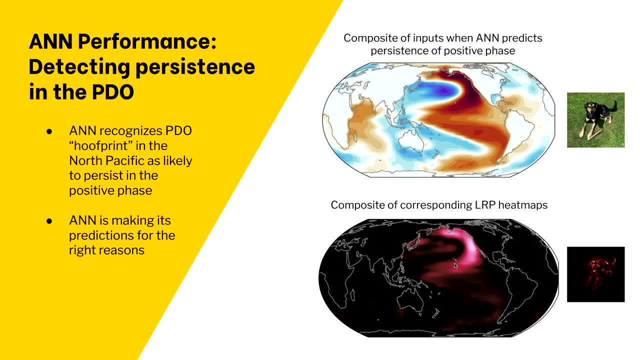 And then this is the composite of inputs. So this is the composite of the corresponding LRP heat maps. And so we see that, yes, the neural network has noticed that this sort of characteristic horseshoe pattern in the North Pacific Ocean is indicative of persistence in the PDO. 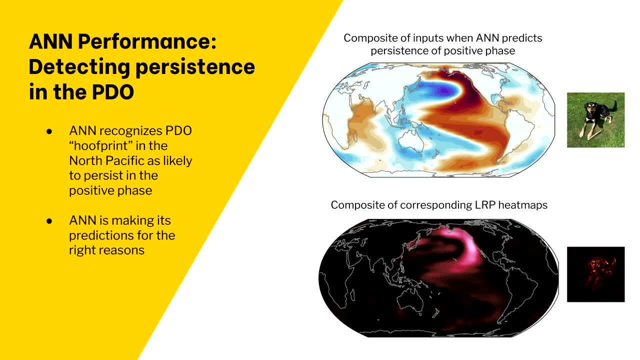 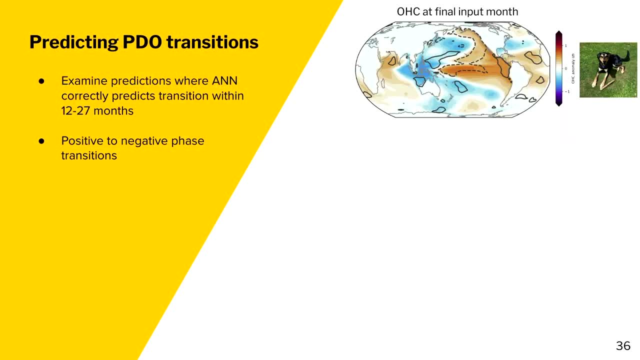 So this is, you know, suggesting that our ANN is making the right prediction for the right reasons. But you know, let's look at something that may be a little more interesting, And that's these transitions in the hello Male. Speaker 1. Is the state of the model just the heat map or is there a change in the 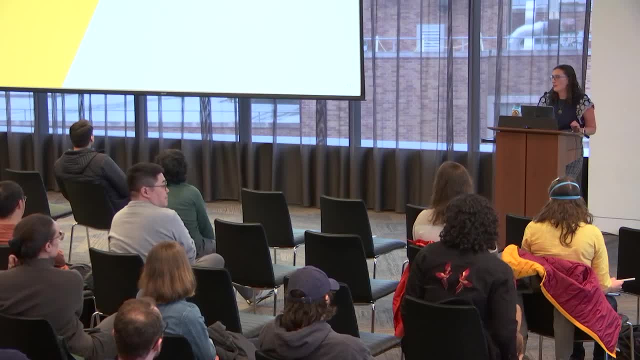 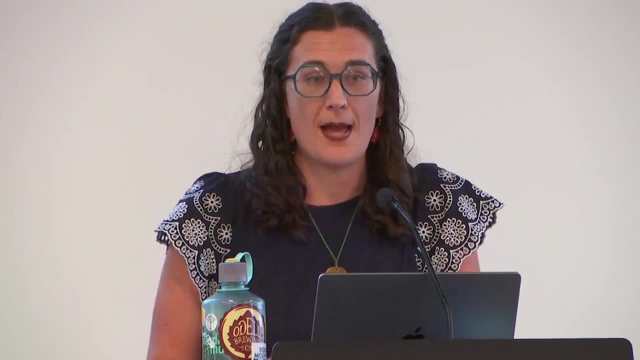 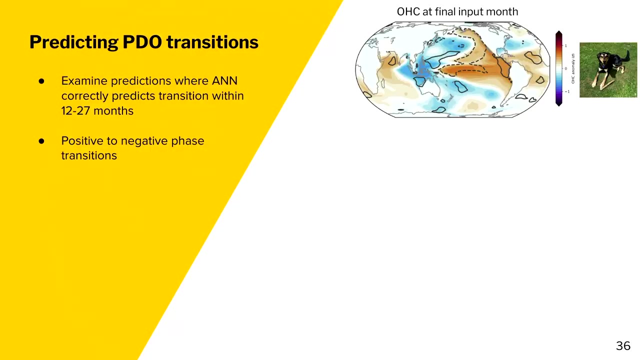 world or other fields that are missing from the PDO's. I'm inputting three ocean heat content maps Here. I'm just showing the final input map. Yeah, Cool, Yeah. So now we're going to examine transitions in the PDO. 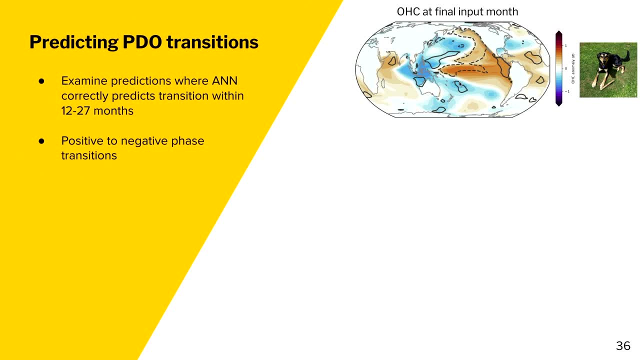 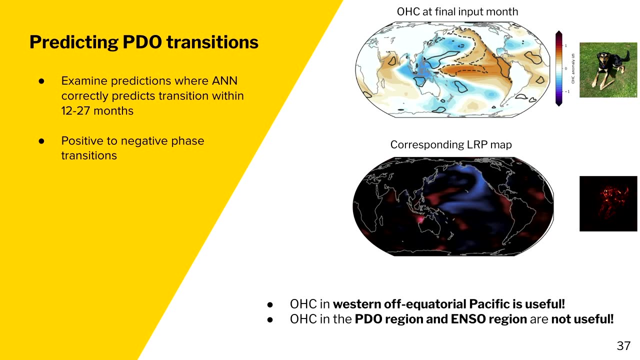 So here is our OHC, that final input map, the composite for positive to negative transitions, And I've contoured over top the in the solid contours, the positive right-hand side of the relevance regions for making a transition prediction. And here is the corresponding LRP heat map. 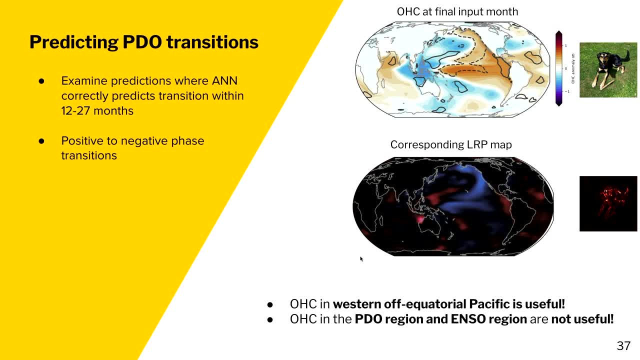 And so we find that heat content in the Western Equatorial Pacific is important for making our PDO transition predictions. But in the sort of in the PDO regions and the ENSO regions or in the tropical Pacific, it's actually not particularly useful. 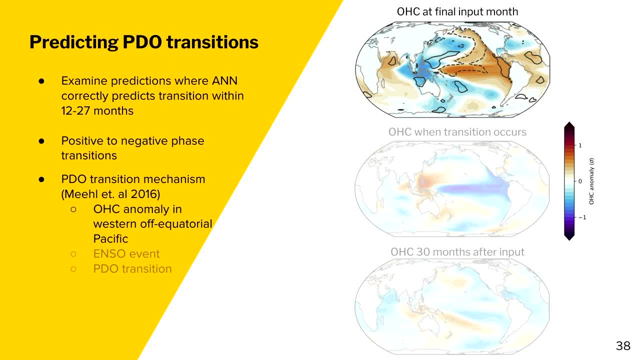 So why might that be? So? there is a PDO transition mechanism that has been posited in the literature, which sort of posits that we have this buildup of heat content, And in the Western Equatorial Pacific, which were followed by an ENSO event. so in this, 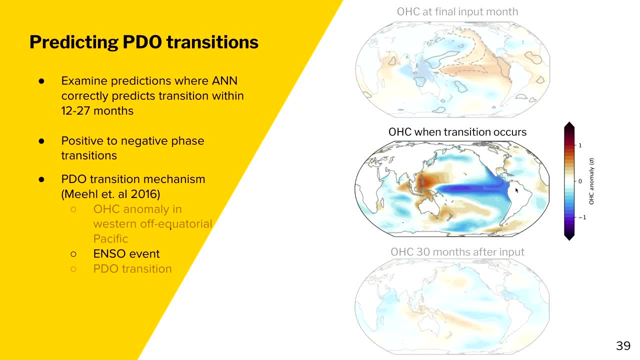 case a La Nina. so we have these negative anomalies in the tropical Pacific can force a PDO transition. So this is sort of the following through from this input map that I had: When I look at when transition occurs, we do find these a strong La Nina event. 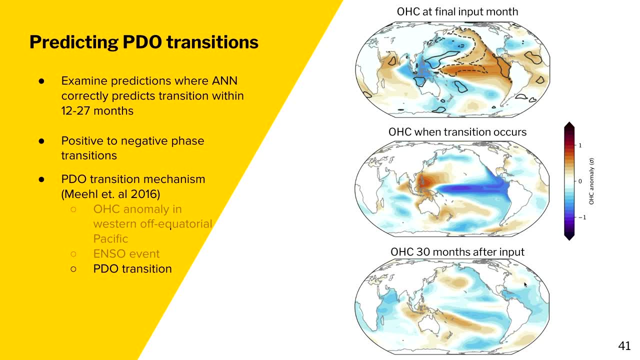 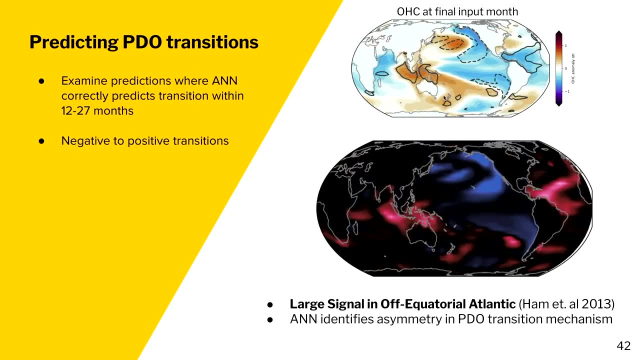 And then, 30 months later, indeed, the PDO has changed sign. So this is indicating that the neural networks were able to sort of learn these preconditioning for a PDO transition. So then we look at negative to positive transitions, which actually behave a little bit differently. 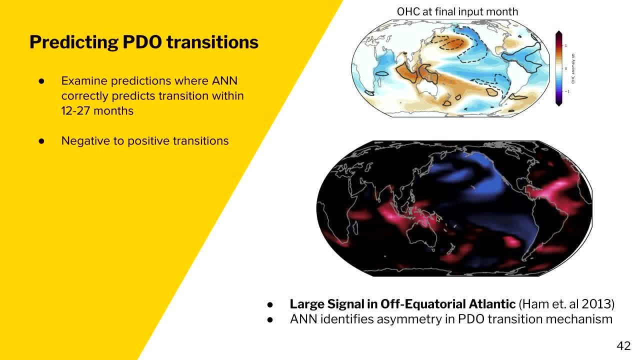 So again, we have this relevance in the olfactorial Western tropical Pacific, but we also have a really strong anomaly here in the Atlantic Ocean, And so I said before that to cause a PDO transition we need an ENSO event. 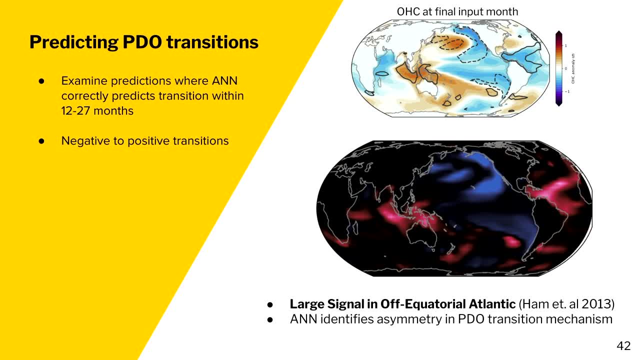 In the previous case it was a La Nina event, but in this case we need an El Nino event to transition from a negative to positive PDO, And El Nino events are thought to be a little harder to predict than La Nina events. 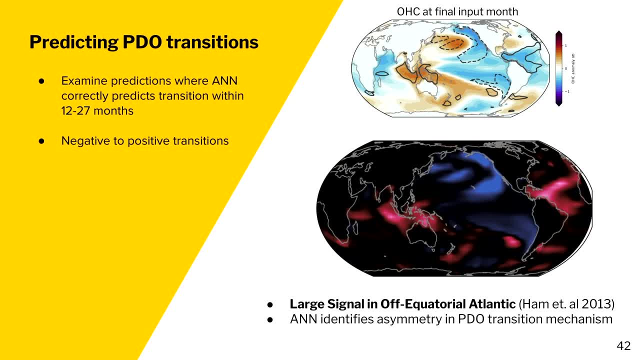 La Nina events often fall. They can follow from an El Nino, but El Ninos sort of need a bit more ocean preconditioning, And one of the things that's positive to sort of be a precursor of an El Nino event is this: 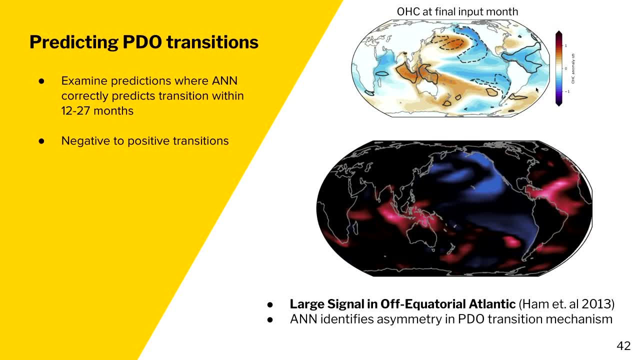 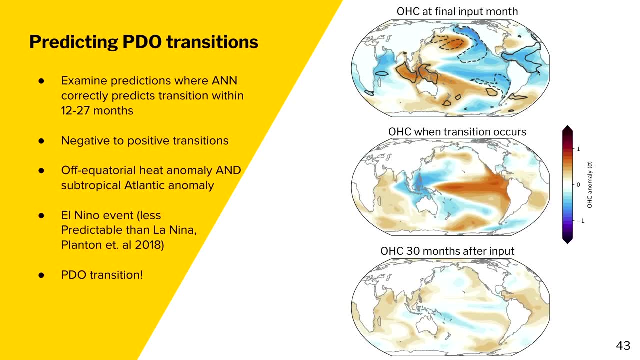 negative anomaly in the Atlantic Ocean here. So it appears that the neural network has learned a sort of extra information it needs for this opposite sign transition. So once again we can go through the similar story, looking at our OHC in the final input. 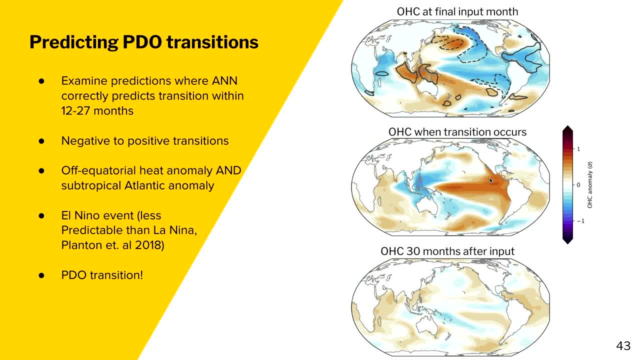 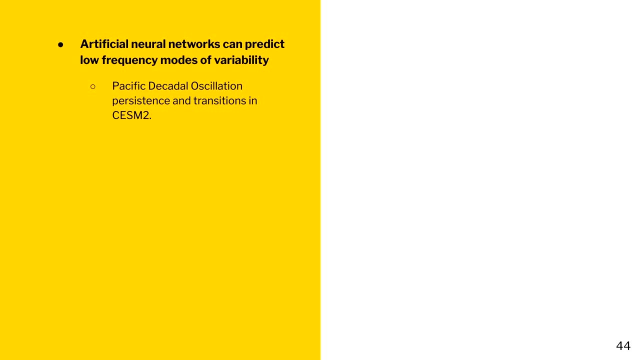 month When the transition occurs. indeed, we do have an El Nino event- and then 30 months later we have our PDO transition. So just quickly going through the results of this first part, we find that our artificial neural networks can predict load frequency modes of variability. so we've learned about 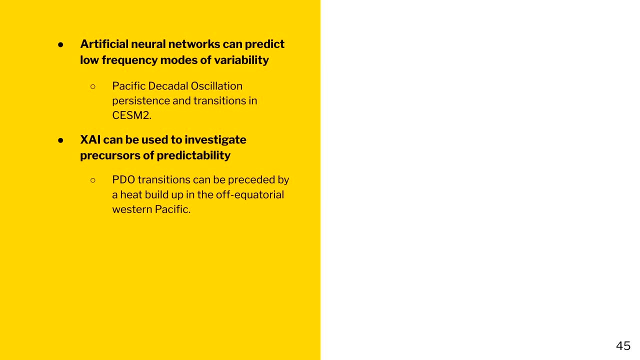 the PDO in CESM2.. We can use XAI to investigate precursors of predictability. So these transitions seem to be preceded by a heat content buildup in the off-equatorial Western Pacific, and then also that the ANNs can recognize the asymmetry and predictability. 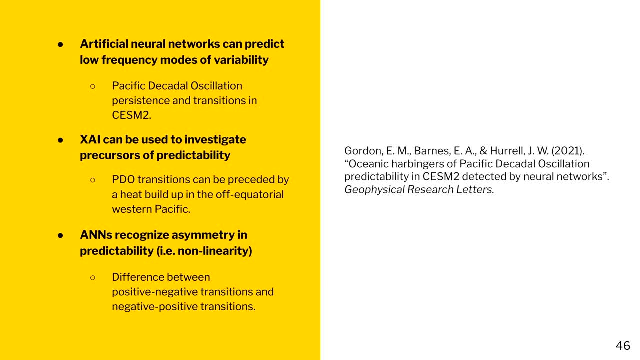 all this sort of non-linearity between El Nino and La Nina. So we can use XAI to investigate precursors of predictability. So these transitions seem to be preceded by a heat content buildup in the off-equatorial Western Pacific, and then also that the ANNs can recognize the asymmetry and predictability. 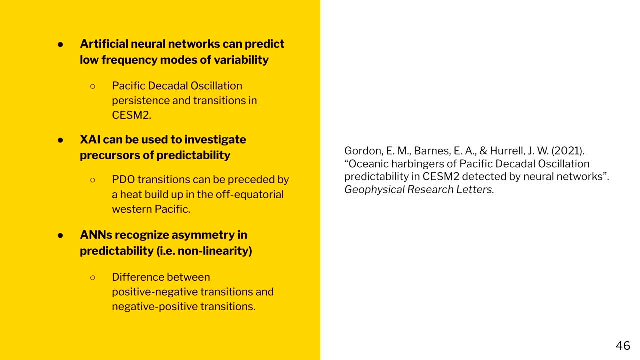 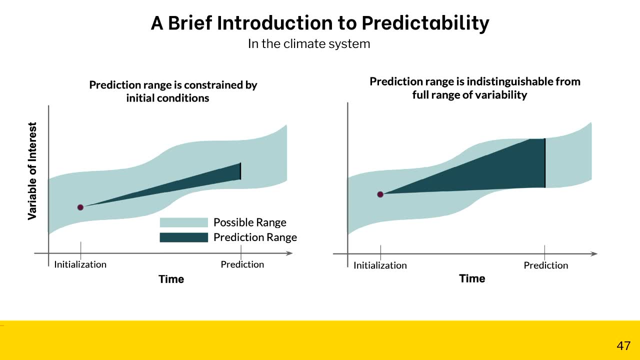 of the ELNs. So we're going to return now to the schematic that I showed earlier about sort of the difference between a prediction that is constrained by initial conditions and a prediction that isn't. So we find that some initial states have more skillful outcomes than others. 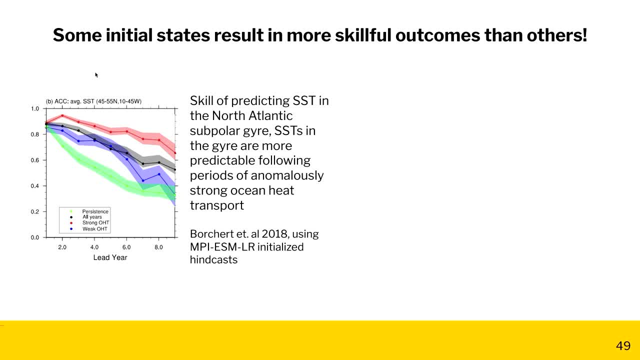 So we have found that this is true on multiyear timescales. This figure is from a paper which looked at the skill of predicting sea surface temperatures in the North Atlantic sub-polar gyre, And this red line here is for the skill of forecasts that were initialized during periods. 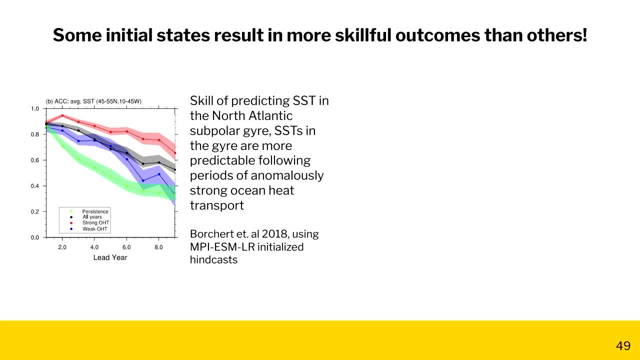 of anomalously strong ocean heat transport into the gyre and the blue is for anomalously weak transport into the gyre And this is showing anomaly correlation coefficient. so the skill of these forecasts. And we see that this red line is higher than the blue line, so there do appear to be periods. 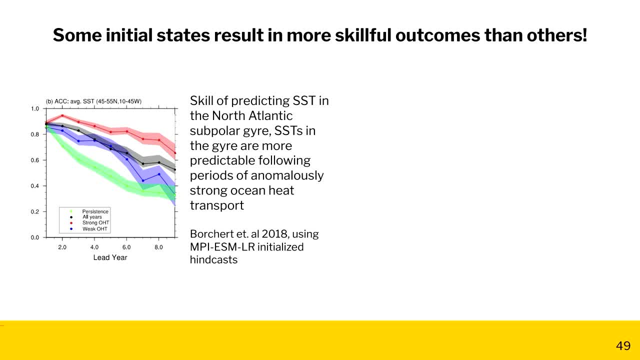 where these forecasts are more skillful and this is a state of sort of more predictability for North Atlantic sea surface temperatures. Similarly, a study used the CESM Decadal Prediction Large Ensemble and found that the information retained in a hindcast, so the sort of information within the forecast is higher for forecasts. 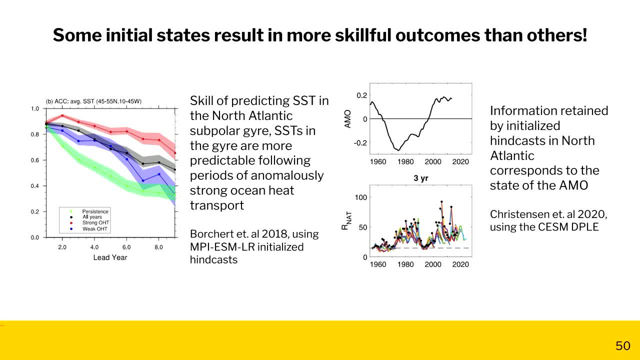 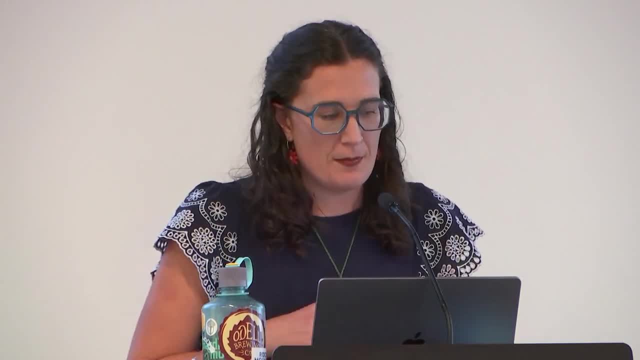 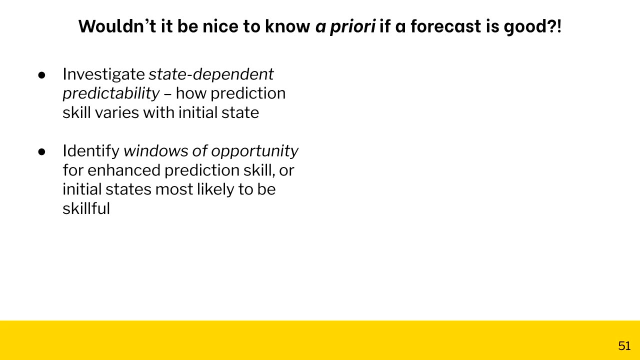 that begin during a sort of anomalously high state of AMO, so basically a lot of heat in the North Atlantic Ocean. So this is building on this idea that, like wouldn't it be really nice to know a priori if our sort of climate-level forecast is going to be good? 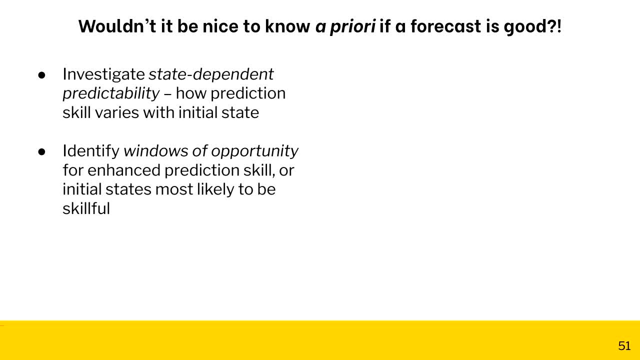 So I'm going to investigate this thing called state-dependent predictability, so how prediction skill varies with initial state. so I'm sort of giving a name now for this concept that I've been sort of going over And in particular, we're going to look at identifying windows of opportunity for enhanced 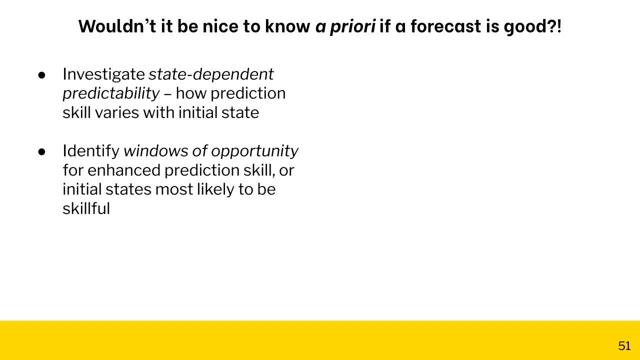 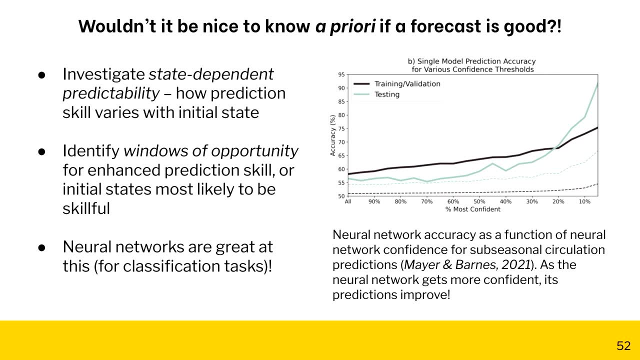 prediction skill, or the initial states that are most likely to be skillful, And it's been demonstrated that neural networks are more likely to be skillful. Neural networks are great for this In particular. this is previously done in classification tasks, so here we have a study. 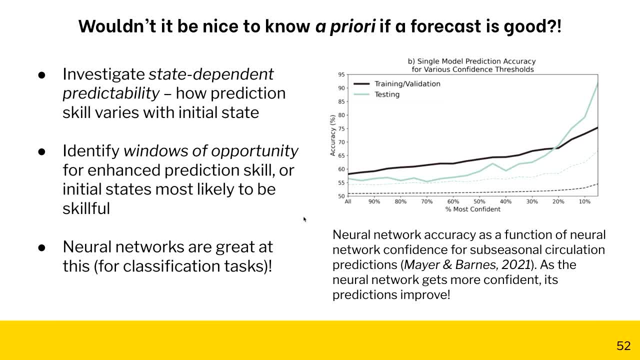 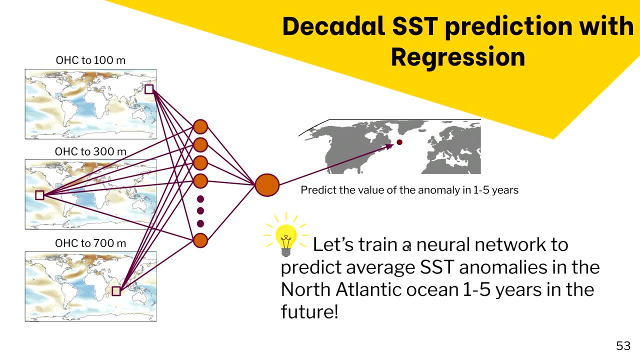 that looked at the predictability of sub-seasonal circulation predictions and they used the neural network's confidence output to find the most predictable states for North Atlantic circulations. So I'm going to look at training a neural network to predict sea surface temperature anomalies at this point in the North Atlantic Ocean. 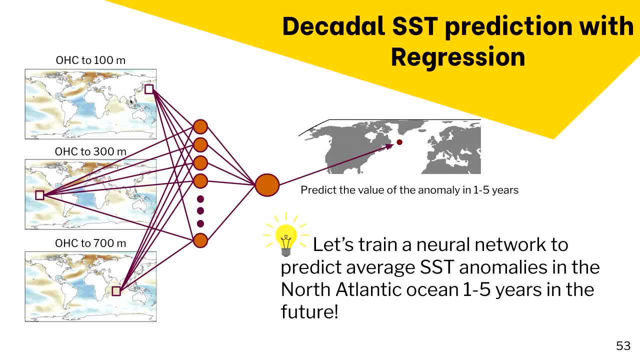 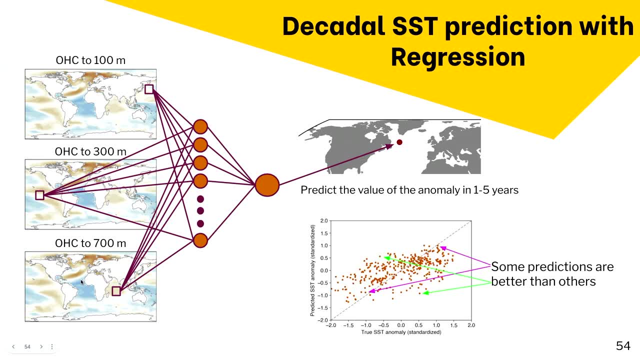 And I'm going to look at this in one to five years- and a similar neural network set up to before and putting information about ocean heat content, this time at different levels in the ocean. So if we sort of naively set this up as a neural network regression task, so we're asking. 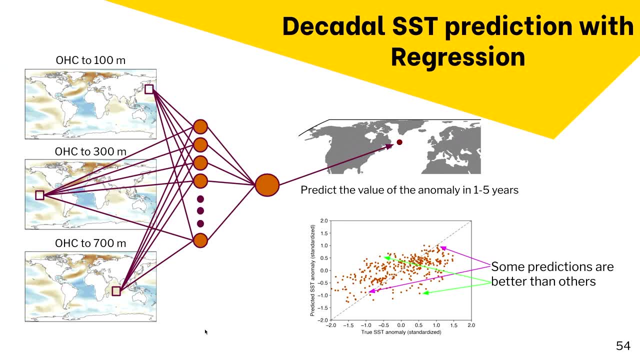 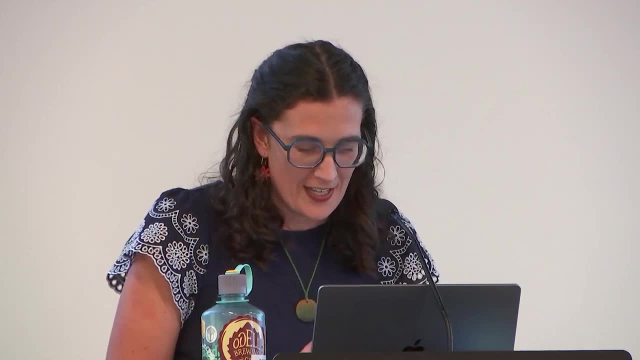 our neural network to predict a future anomaly, we'd get something like this. So, with our truth along the x-axis and the predicted along the y-axis, this is not a great fit really, You would. Some of these dots, So I've indicated with pink arrows, are better than other predictions with the green arrows. 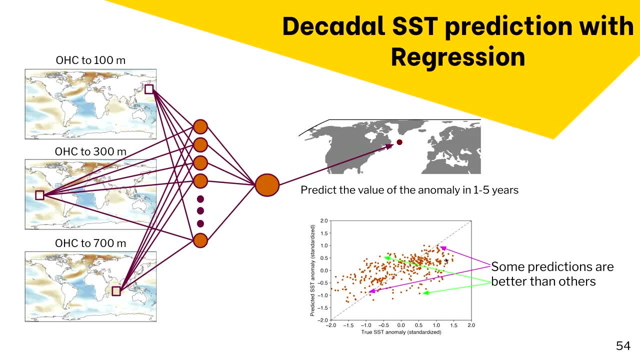 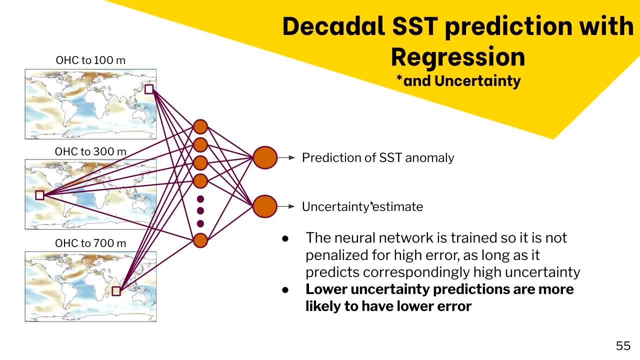 So we want to somehow know if our prediction is going to be closer to this one-to-one line or our prediction is going to be closer to the truth. So instead of just predicting a sea surface temperature anomaly, we're also going to get our neural network to give us an uncertainty estimate with its prediction. 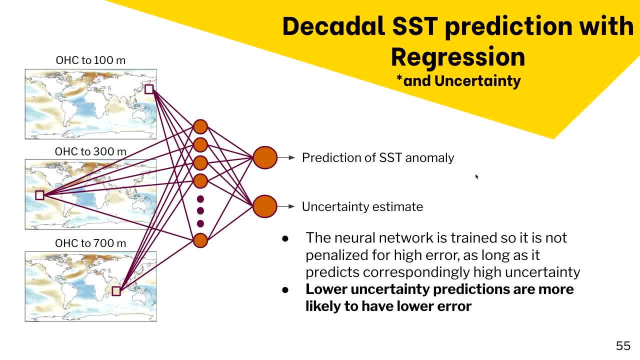 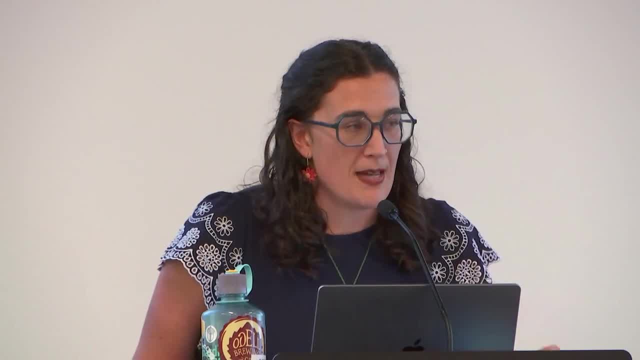 And our neural network is trained so that it's not penalized for predicting a high error anomaly as long as it guesses a correspondingly high uncertainty. And so what this means Is that if we grab our predictions with relatively lower uncertainties, is that their predicted 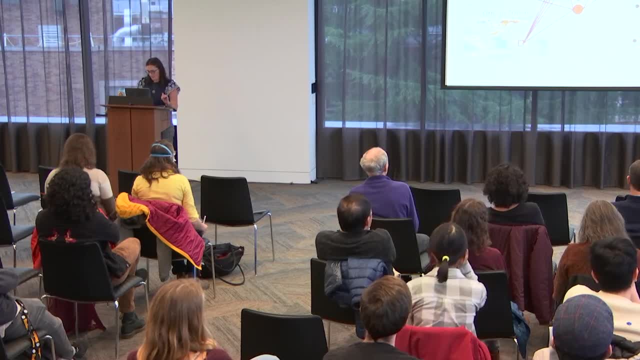 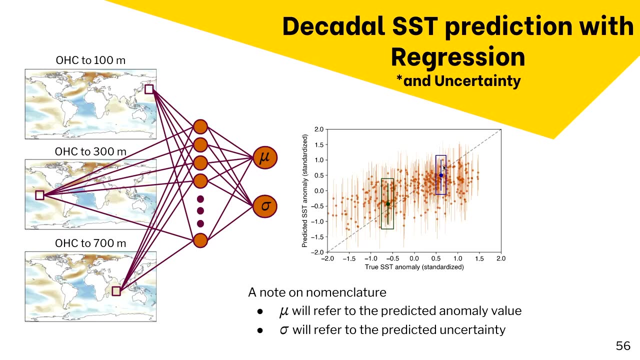 anomalies should be closer to the truth. So I've indicated this here, that once we add these uncertainty bounds, we can sort of see- Well, we can see the uncertainty bounds. And a note on the nomenclature that I'm going to use. 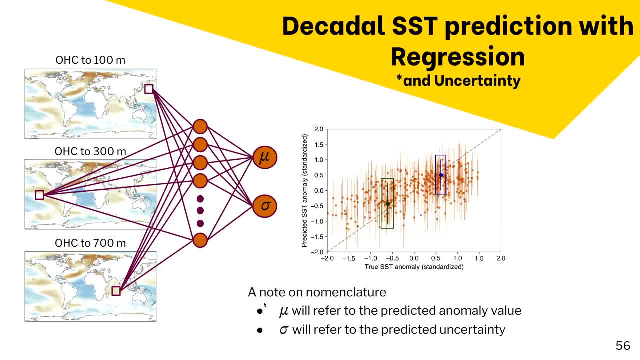 So when I use mu, I'm going to refer to the predicted anomaly and sigma to refer to the predicted uncertainty. Once again, I'm using my 2000 years of clinical data. So I'm going to use mu, I'm going to use mu. 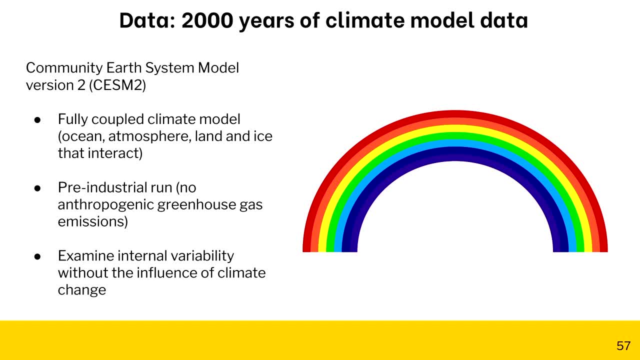 I'm going to use a modeling problem problem, So let's see how I do this. So we use the most common model for the improvement of our general analysis of climate model data, because we're wanting to examine internal variability without the influence of climate change. 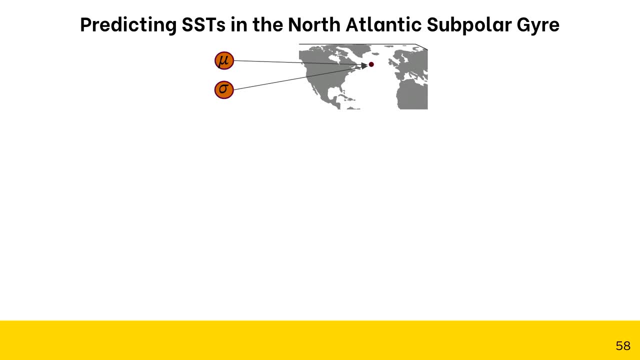 So we're predicting sea surface temperatures in the North Atlantic subpolar gyre, And so this is our map of truth versus predicted. Once again, not the best, But can we find these states of enhanced predictability? So one way I'm going to do this is using this thing called the discard test, which, as it, 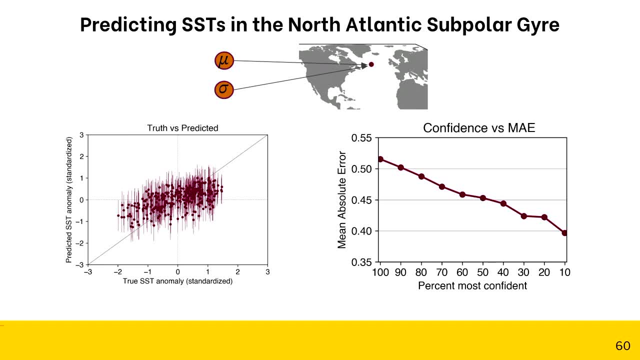 says on the tin, it's discarding samples with increasingly Increasingly low uncertainty. So, for example, if we look here at the 100% most confident, so this is keeping all of our testing data. so this is just the skill across the entire testing set and our mean. 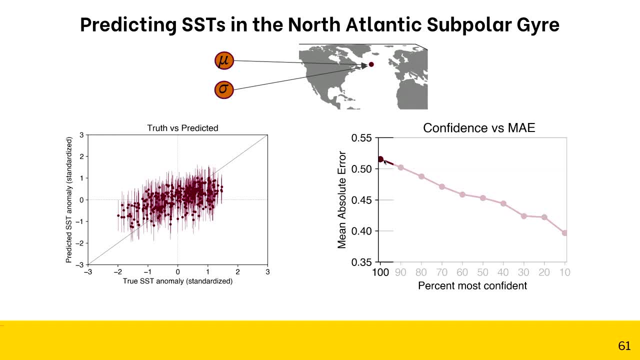 absolute error is 0.52 on this standardised error. However, if we only keep 20% of our samples and we choose the 20% of samples that have the lowest predicted uncertainties, we find that our error has now dropped to about 0.42.. 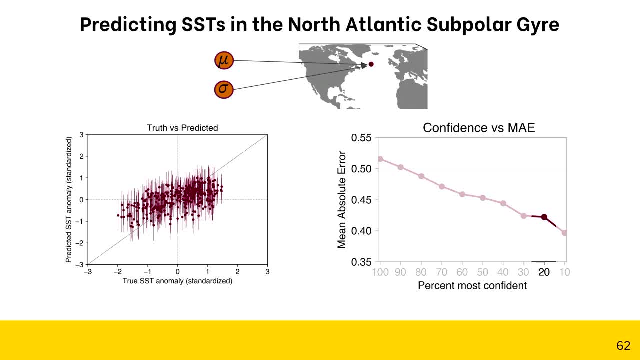 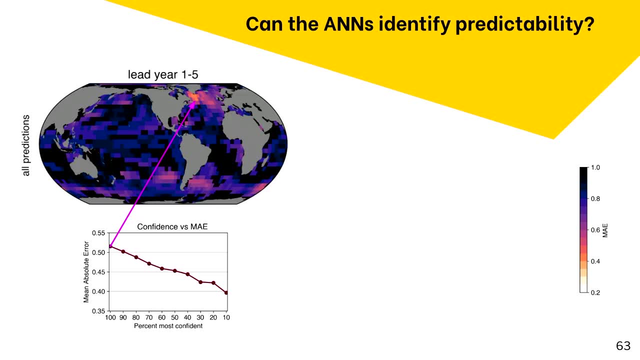 So this is demonstrating that our neural network is able to identify predictability within the data by assigning it a relatively higher or lower uncertainty. So I trained a neural network at each point in the ocean. so this is, you know, pointing to this point up here. 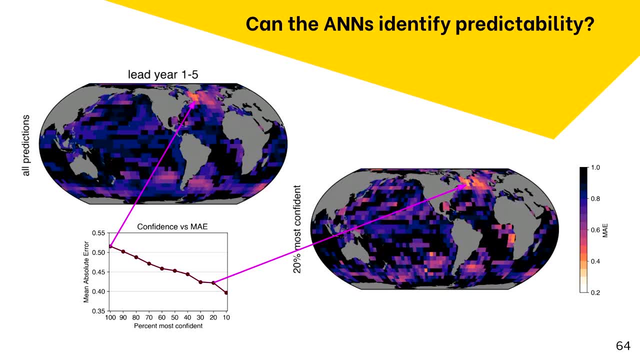 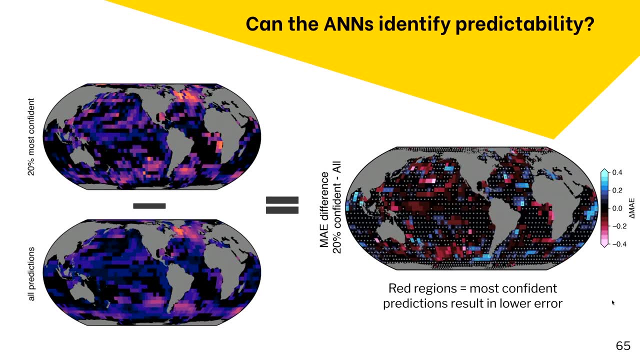 And then, if we do the same thing at each grid point, we look at the 20% most confident predictions- this is this map here on the right- and we're looking at mean absolute error, so brighter is better. And then we subtract the two to find places where 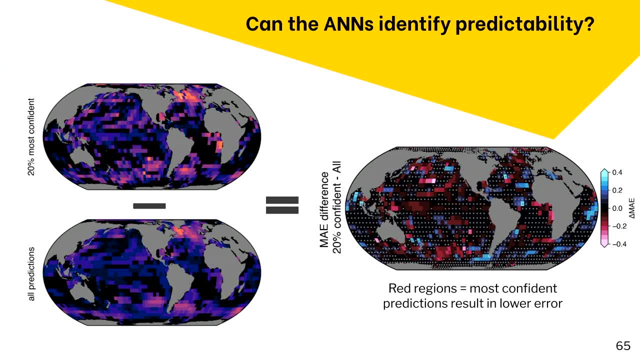 Okay, The 20% most confident samples have better skill. so the places where we are identifying these states with enhanced predictability, So that's all of these red regions here. So this is indicating that you know, even in the mean we might not have that much predictability. 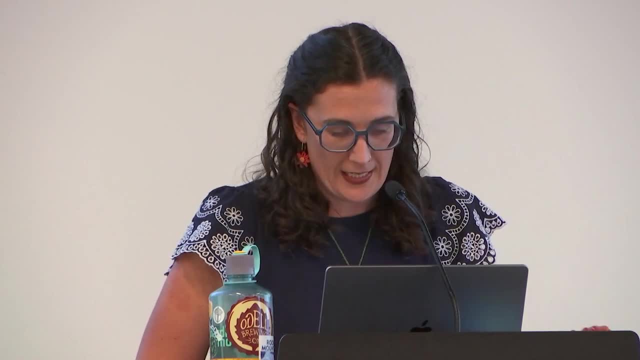 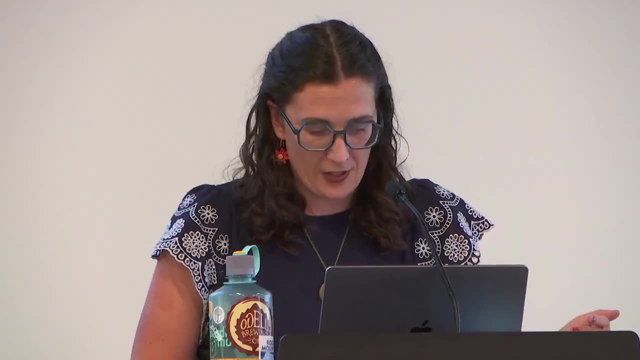 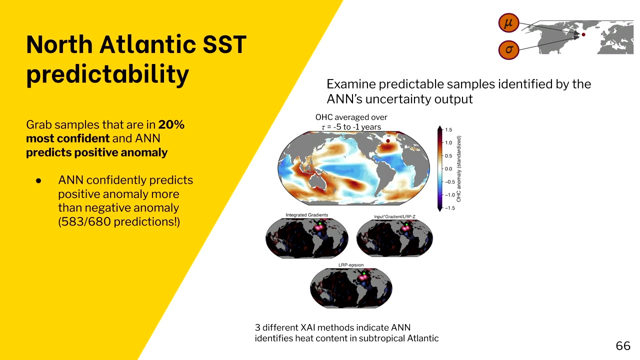 but when we start to really probe these states of enhanced predictability, it really exists sort of widespread across the ocean, in particular sort of North Atlantic, North Pacific and across some of the Southern Ocean. Okay, So once again we want to think: okay, what are the actual mechanisms that are providing? 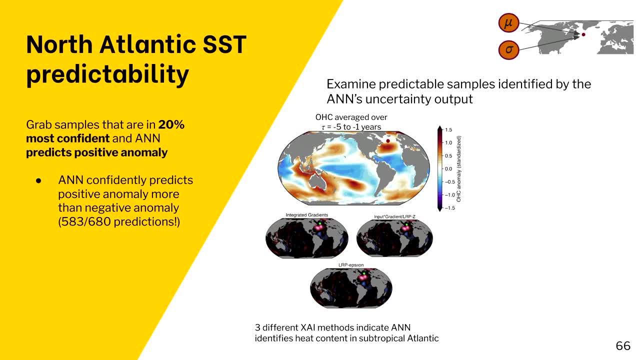 us predictability on these timescales. So I'm going to look again at our point in the North Atlantic Ocean and look at the samples, the predictable samples, identified by the ANN's uncertainty output. So we grab the 20% most confident samples here and it just so happens that these are 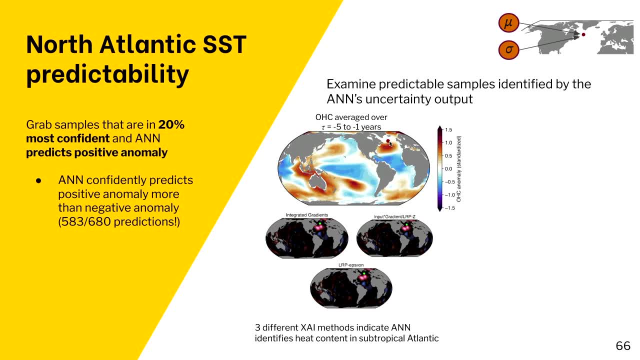 mostly predictions of positive anomaly at this region here and this is using. So this is a composite of these 20% most confident samples. And then down here we have the Down. here we're using three different XAI or XAI methods for understanding where the 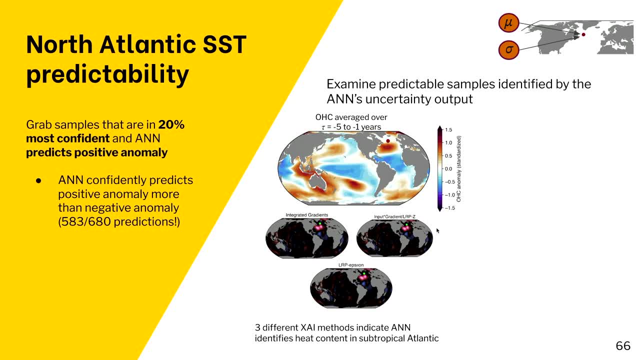 For understanding which grid points were relevant to our neural networks predictions. So we find that they sort of overwhelmingly point to this ocean heat content anomaly in the subtropical Atlantic Ocean. And if we look at the sea surface temperature over this period as well, we find that we 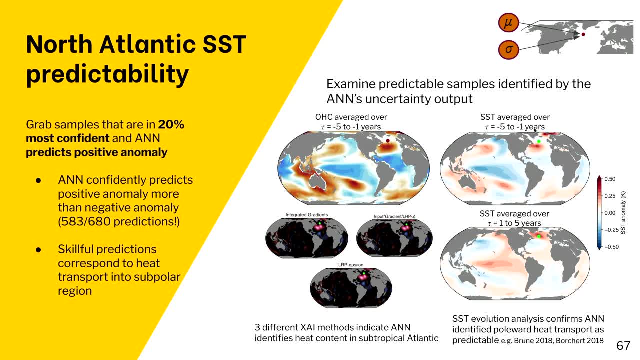 have a corresponding sea surface temperature anomaly, you know, one to five years before our prediction, Which has moved into the subpolar zone. So we have two different XAI one to five years later, suggesting that it is one of these states of enhanced predictability when we have a period of enhanced northward heat. 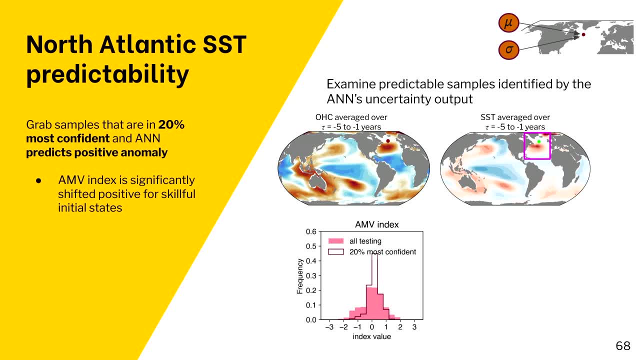 transport. Something else that was interesting to me here is to look at sort of what's going on sort of basin wide here. So we look at the AMV index, so sort of an index of Atlantic variability. The shading here indicates the full range of variability within the data. 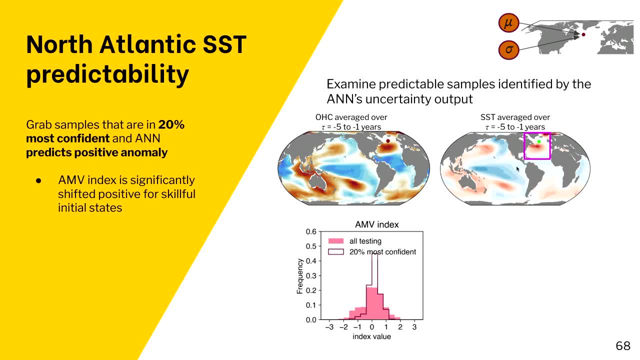 And the solid line is just for these samples in particular, and we find we have a slightly positive AMV index when we have a skillful prediction, which is, I think, slightly unsurprising. but if we look in the Pacific Ocean- so here I'm using something called the IPO index- it's very 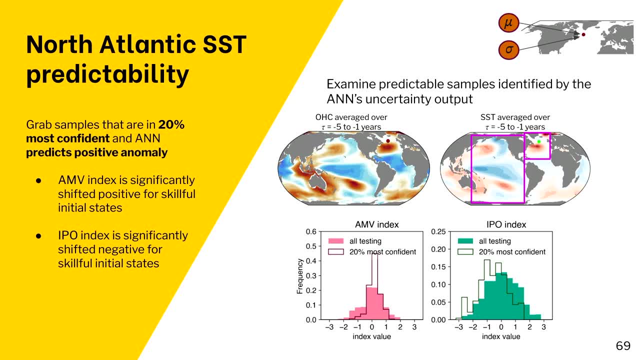 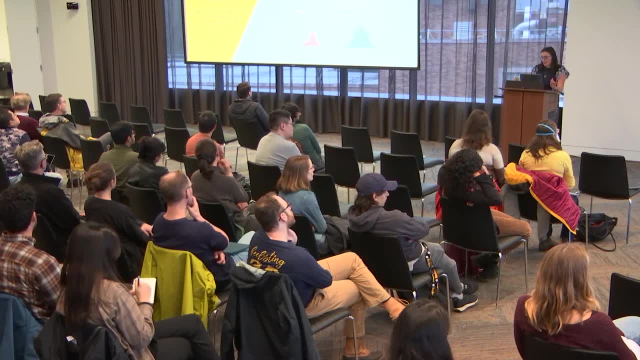 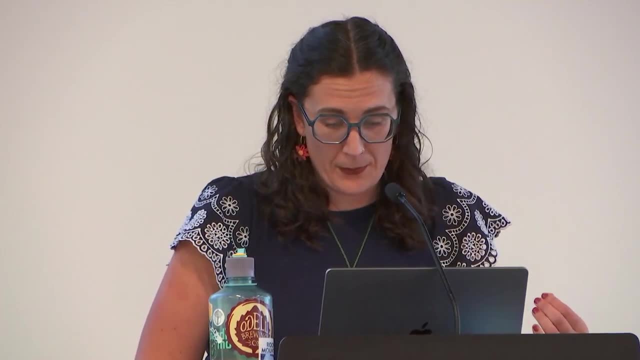 similar to Pacific decadal variability, but it includes the full meridional extent of the Pacific Ocean. So once again we have our shading as the full testing data, but our 20% most confident samples are this outline here, And so we find that when our ocean is preconditioned for this predictable state in the North Atlantic, 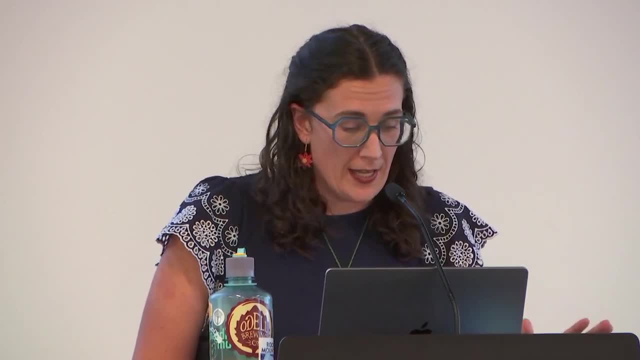 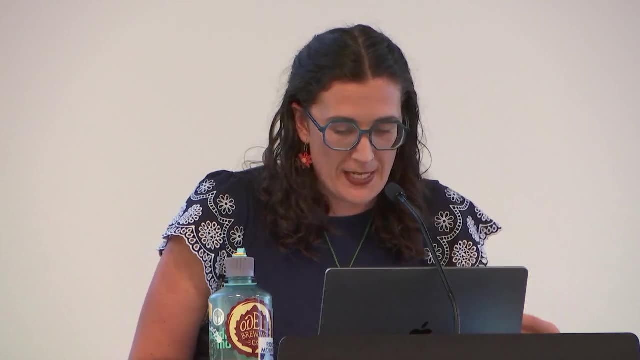 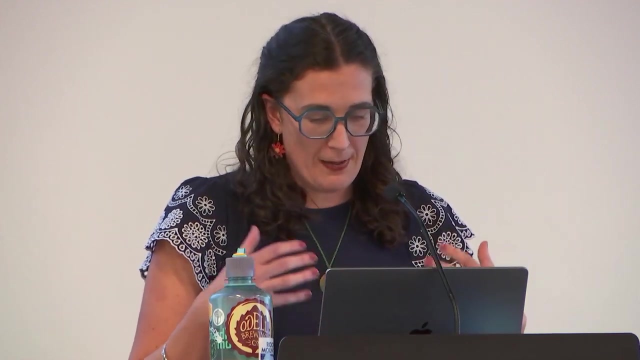 Ocean. we have a really strong negative IPO signal here and this is really, really interesting to me: this idea of, if our explainability method is highlighting this region here in the North Atlantic Ocean, what else is happening in the ocean that may be helping to build. 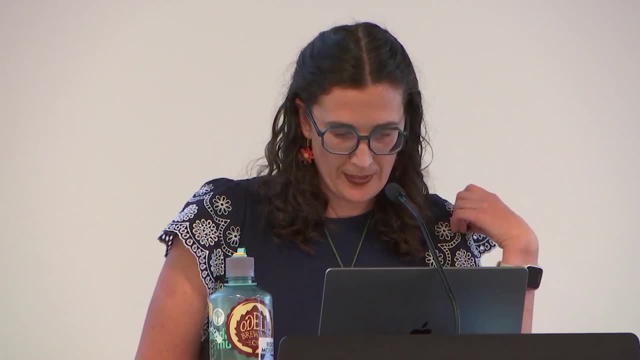 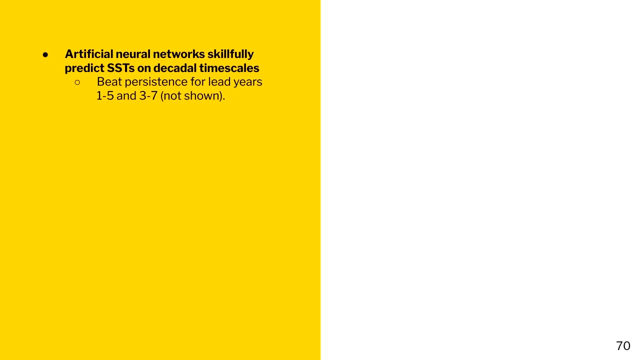 these predictable initial states. So to summarize this section, I looked at artificial neural networks predicting sea surface temperatures on decadal timescales. It beats persistence for two different lead times which I have in the supplemental Neural networks. identify these more predictable states by assigning lower uncertainty to predictions. 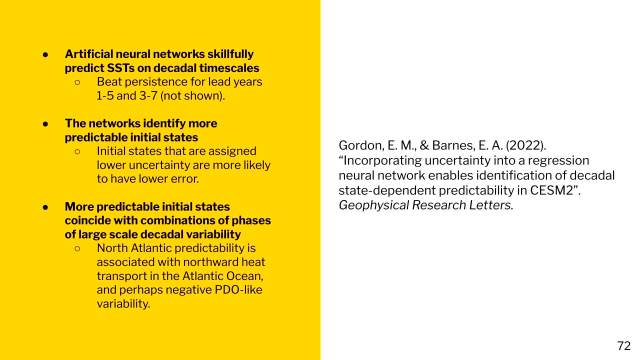 that are more likely to have lower error And we can use these predictable initial states to sort of probe the predictability, the mechanisms leading to predictability, and I have shown an example in the North Atlantic Ocean And once again, this study is also available in geophysical research leaders. 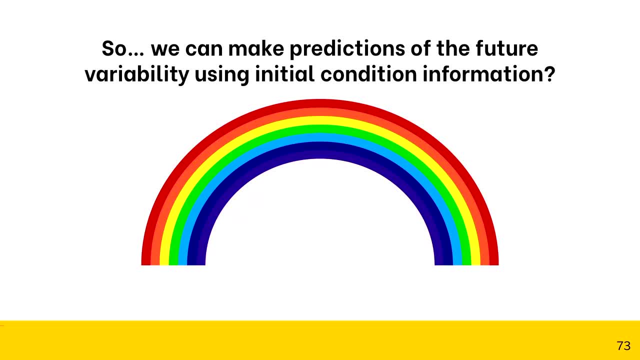 Okay. So I'm sure we're all thinking, oh my goodness, this is great. we can make predictions of our future variability using our initial condition: information. right, we're living in this rainbow world? No, we're not. We're living in a world where humans have had, you know, quite an influence on our climate. 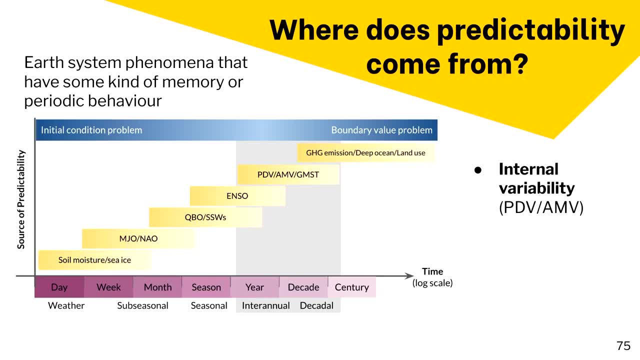 in the last you know, 100, 150 years or however long. So I sort of skipped over this a little bit earlier, where I said that predictability comes from Earth system phenomena that have some kind of memory or periodic behavior, because predictability also comes from the human impact on the climate system. 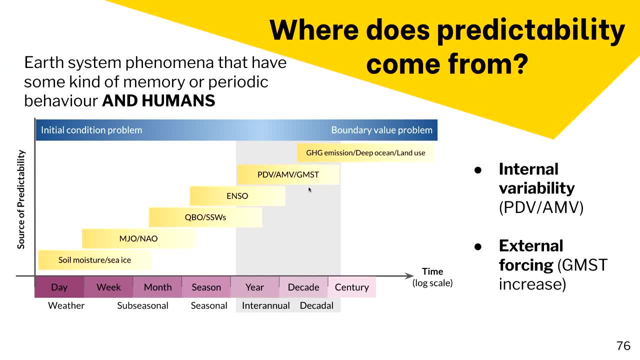 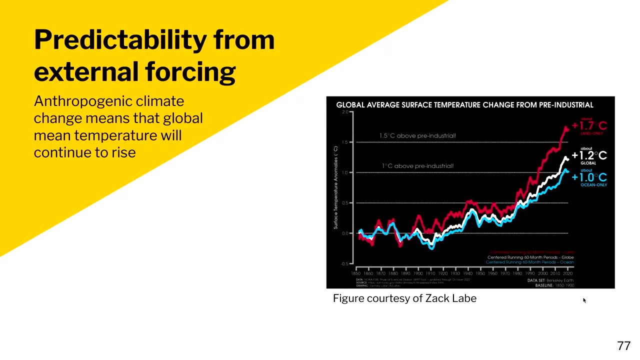 So here now we've added this little GMST here, which stands for global mean surface temperature. So the predictability on decadal time scales can be provided by the expected increase in global temperatures in the next few years, also from the external forcing in the system. 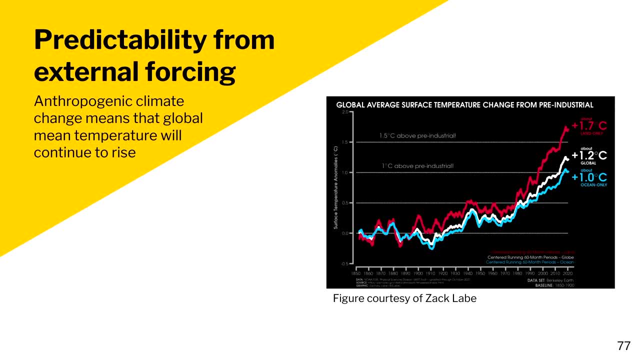 So I'm going to go through an example of what we mean by predictability from external forcing. So this is a figure here which is showing global global temperature. Okay, So global mean surface temperature. so the red is land, only the white is global, and 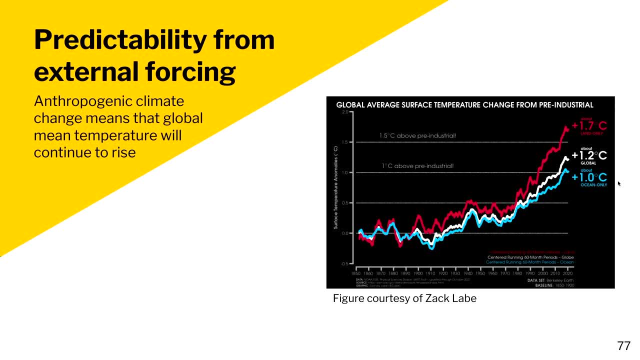 the blue is ocean only, And these are all showing a rise in temperature over the last sort of 50 years or so. Now this is like a thought experiment, because I don't have a million dollars, but I will give you a million dollars. 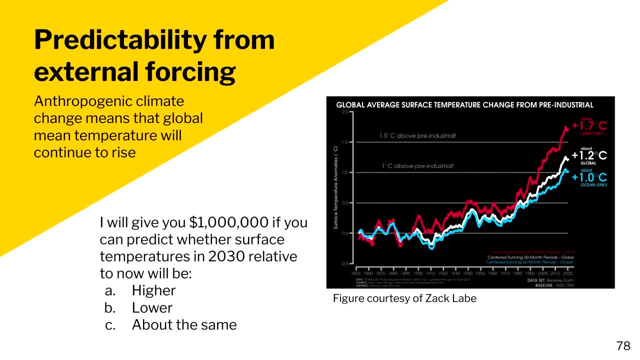 If you can predict whether surface temperatures in 2030, relative to right now, let's say, in the Washington region, will be higher than they are now, lower than they are now or about the same Now. So I'm going to say higher because you want to win a million dollars. 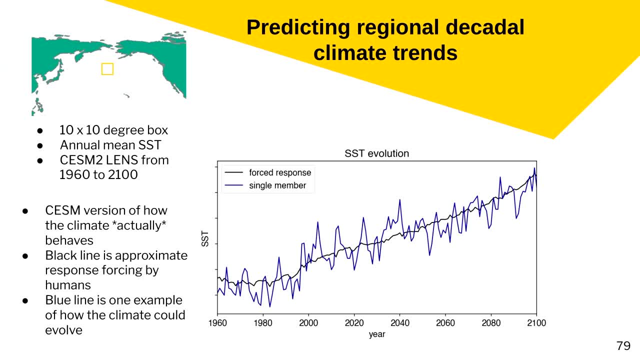 But actually, when we look on more regional scales in the climate system, there's much more variability than we actually, than just you know. temperatures will continue to rise, So here I'm showing a time series of sea surface temperatures from this box here in the North. 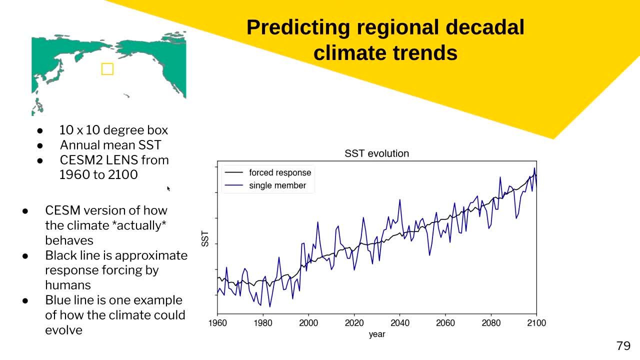 Pacific Ocean from the CESM2 Large Ensemble. So this is a climate model version of the historical period and also the next sort of 80 years up to 2100.. And the blue line is one version of how the climate might actually behave. 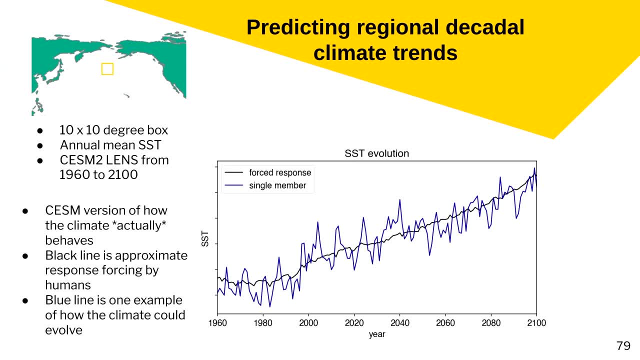 And the black line is an estimate of the approximate forcing from humans. So I'm highlighting this region here from 2020 to 2060. And I've drawn on four sort of consecutive decade or 10-year trends And what we can see is even within the next 40-year period, we have periods of, you know. 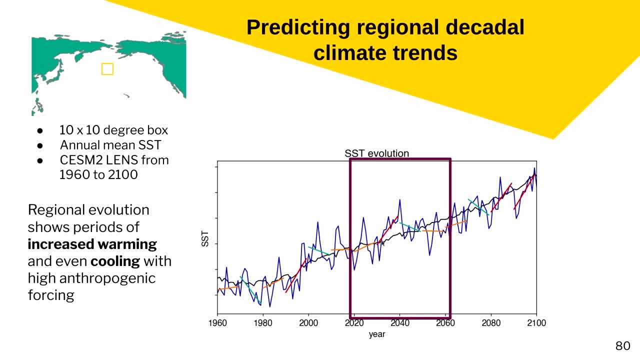 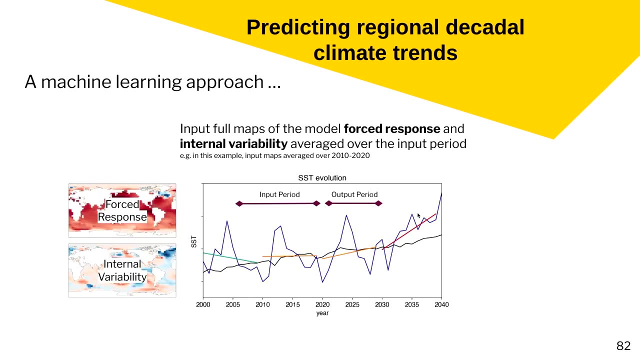 anomalously high warming or increased sea surface temperature trend, but we can have these periods of cooling as well. So in a question that I'm really interested in, would something like this be predictable in the presence of this background forcing trend? So we're going to take a machine learning approach to this. 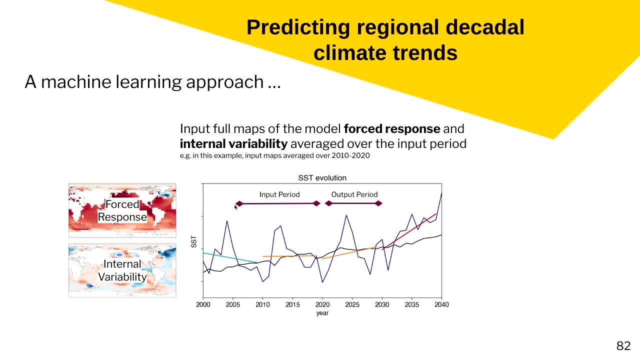 So I'm going to sort of give an example of how our prediction system is working. So we're going to go over an input period of about 15 years and input on your network, information about the forced response to climate change and information about the internal 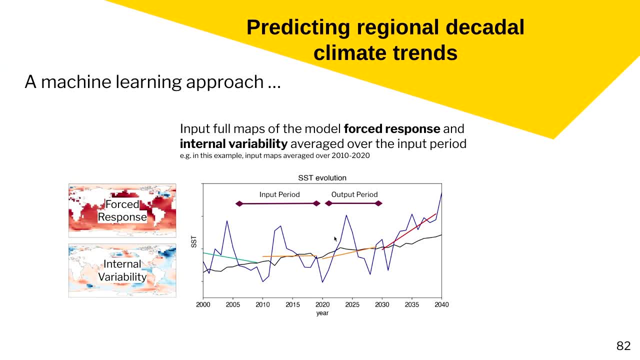 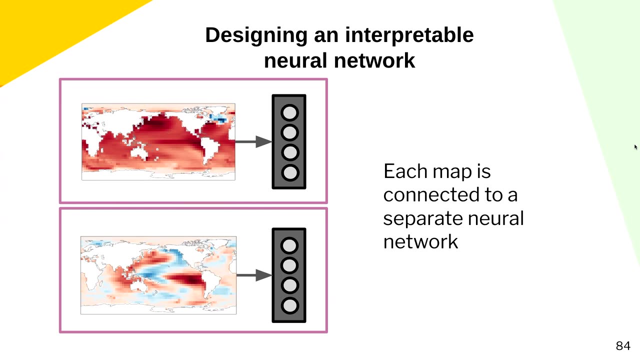 variability of the climate And our output will be a prediction in the next 10-year period. will the future 10-year trend lie in the lower, middle or upper third of the possible sea surface trend distribution? And the way we're going to do this is we're actually going to split this into two parts. 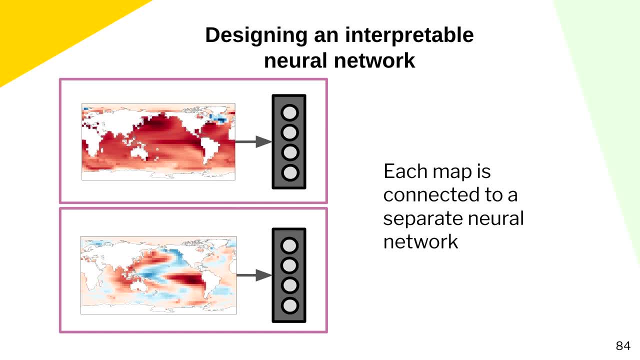 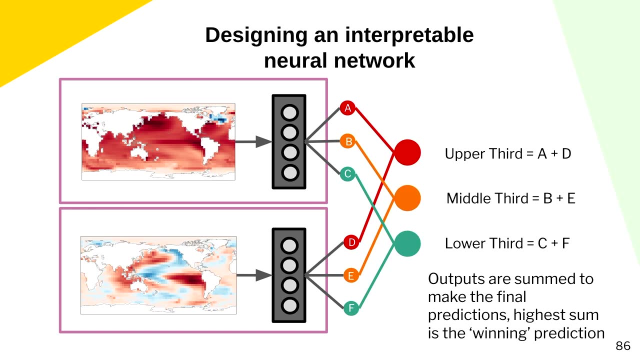 so we can really break this down into the contributing parts of the system. So we're going to connect the forcing to one neural network and the internal variability to another neural network, And each of these networks outputs its own tersile predictions. These predictions are then summed in the final step and the prediction with the highest 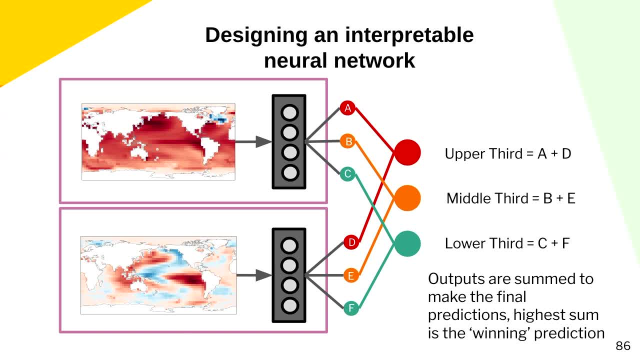 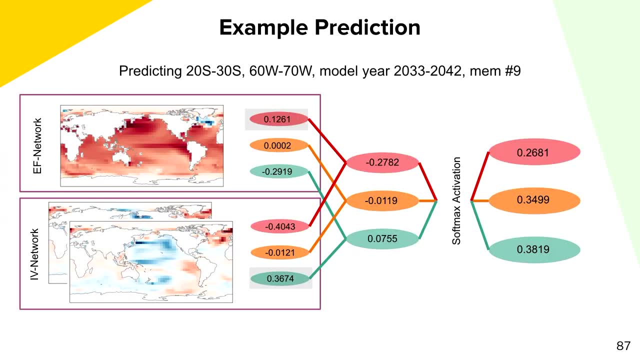 sum is considered the winning prediction. And these are trained at the same time, so the neural networks must sort of learn to work together to weight their contributions to the final outcome. So I'm going to go through just an example prediction. This is a real prediction from the neural network trained at 20 to 30 south and 60 to 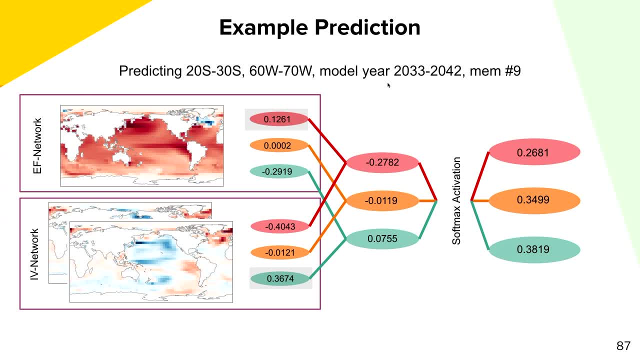 70 west. So this is a prediction of model year 2033 to 2042. in ensemble, member number nine. So this is real. you know typing it into my computer and telling me to output all these numbers. So the external forcing network predicts about 0.1261 here. so it's predicting a upper tersile. 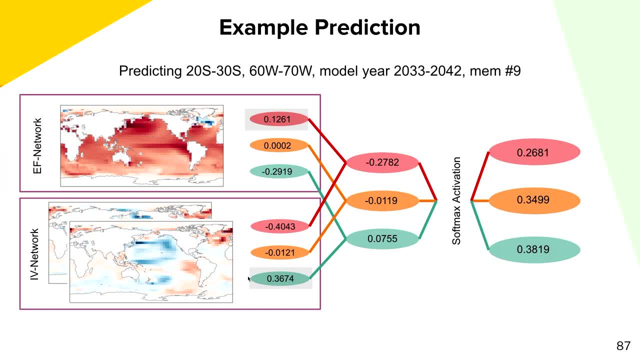 trend, But the internal variability network is putting a lot of weight on this lower tersile trend And then when we combine the predictions together, we find that it is the lower tersile trend that is the winning prediction. So this demonstrates that the lower tersile trend is the winning prediction. 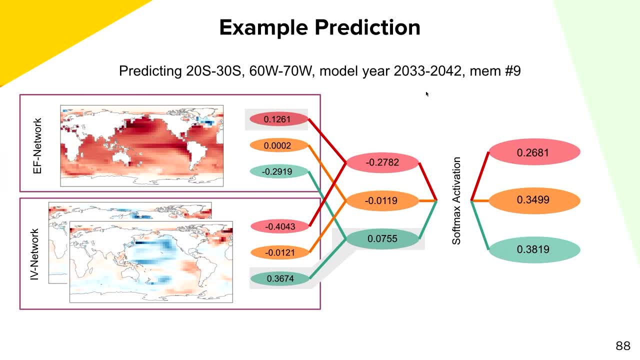 So we can see that even in this sort of period, in the next sort of 40 years, there are periods where we can make predictions of a negative trend from internal variability information. So internal variability is contributing to the predictability of the system. 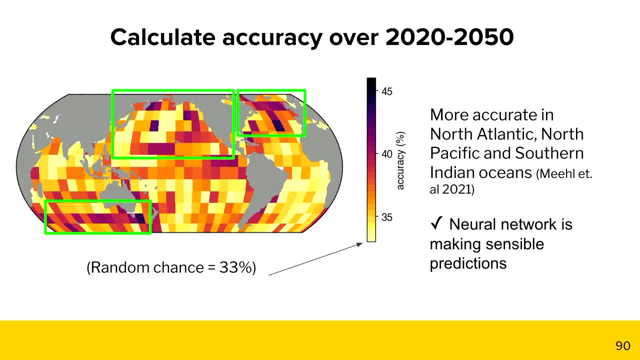 Oh, I just said all that, Okay. So once again, I have trained these neural networks at every point in the ocean, And here I am showing the skill of the neural networks, so just sort of as a quick check to make sure that we're getting more skill information. 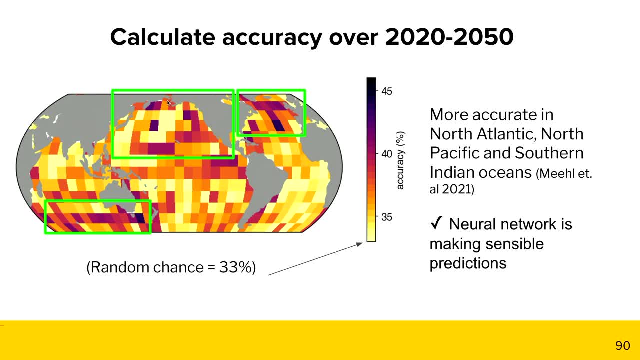 So once again, we have skill in the North Pacific, skill in the North Atlantic and then skill in the Southern Ocean, So we can sort of check the box. yes, these neural networks are making sensible predictions. So now we want to tease out the contribution of internal variability to our predictability. 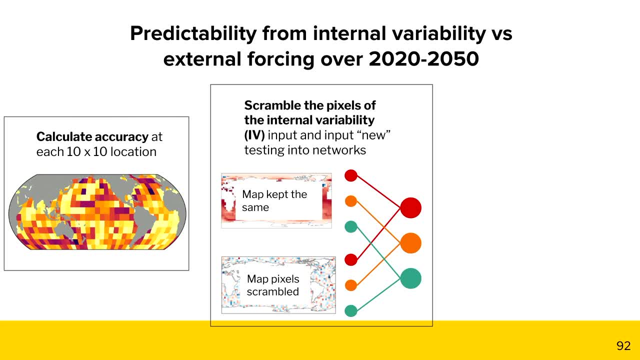 So this is the figure I just showed, And now we're going to do something called permutation importance testing to examine the contribution of internal variability. So we're going to keep our information about external forcing the same, But we're going to scramble this out. 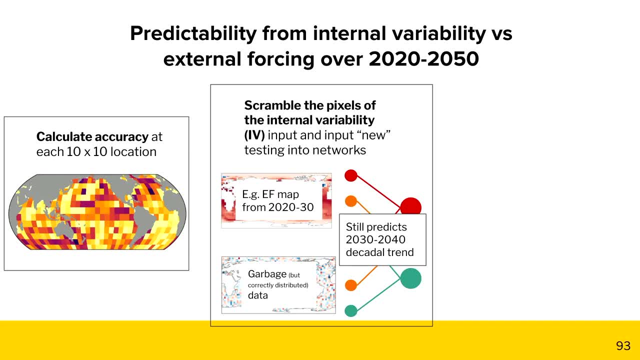 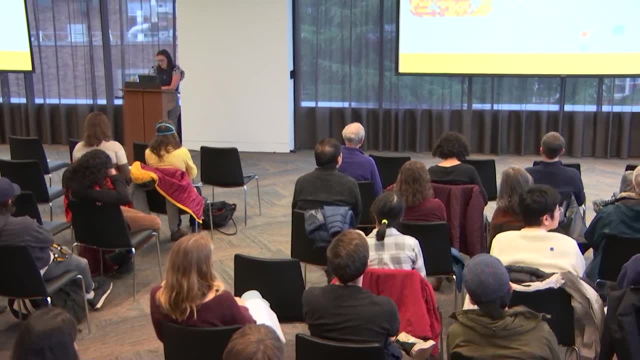 Okay, So we're going to scramble the information about the internal variability. So an example prediction task could be inputting the external forcing map from 2020 to 2030, and then inputting garbage. but you know, correctly distributed garbage into the internal. 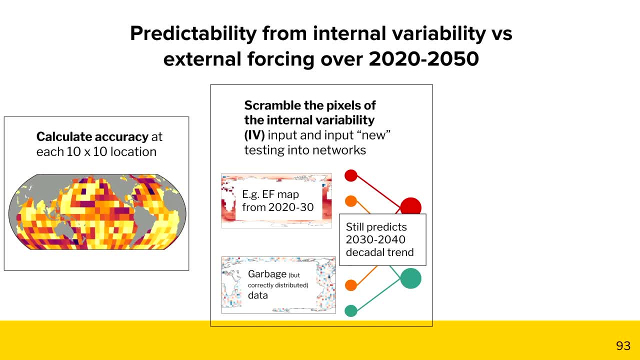 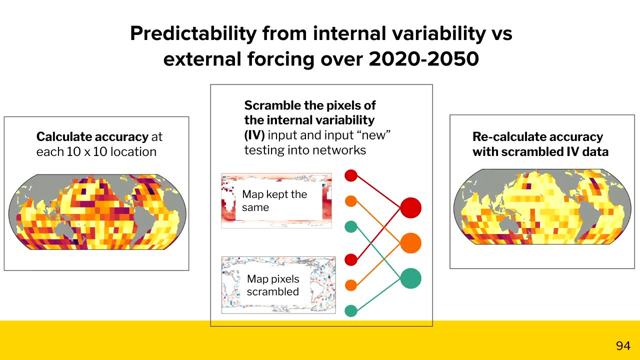 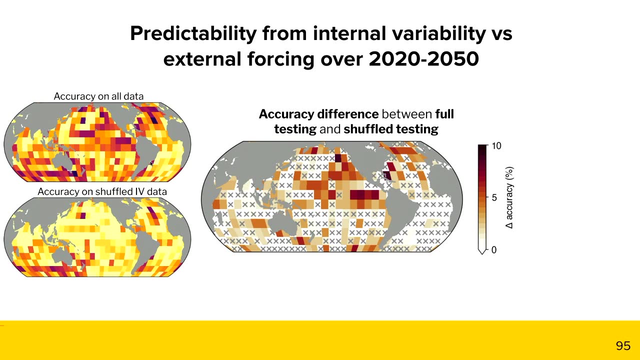 variability network and asking the full network to still predict 2030 to 2040.. And then we recalculate our accuracy at each grid point on this shuffled internal variability data. So this is as before. So this is our accuracy across all data, our accuracy with our shuffled internal variability. 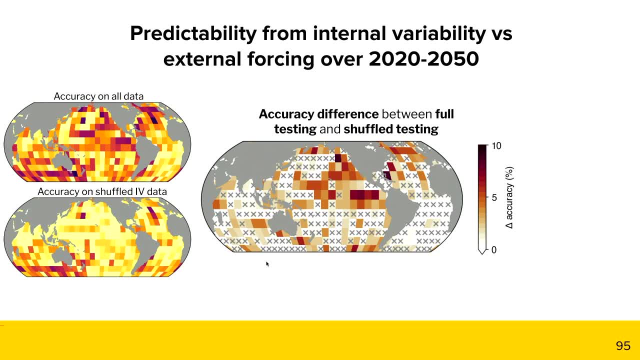 data And then this figure here is just the difference between the two, And so an interpretation of this figure was: if the networks were only using external forcing to make their predictions, this figure would be zeros everywhere, because internal variability would not contribute to the neural network skill. but we do find skill in the North Pacific. 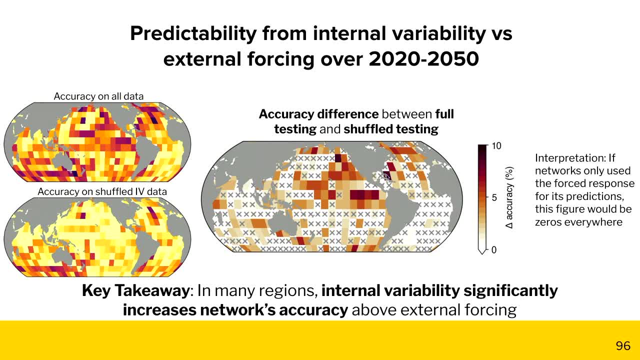 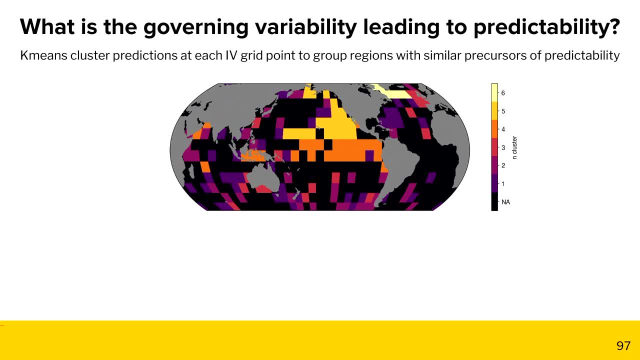 Ocean and in the North Atlantic Ocean. So this is suggesting that the internal variability does significantly increase the neural network's accuracy above external forcing. So another question might be: so what is the governing variability leading to predictability in all of these regions? So what I did is k-means clustering the predictions at each grid point where internal variability. 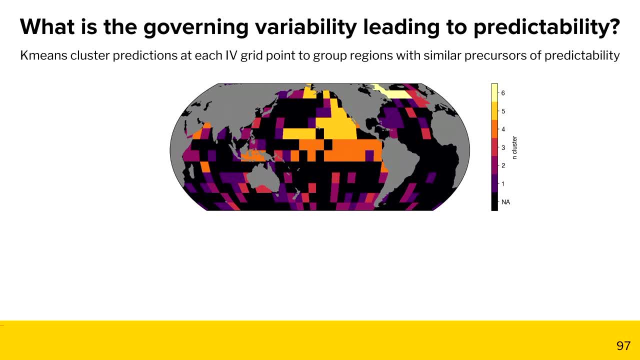 was important to predictability to look for regions grouped together, regions which had similar precursors of predictability. So this is suggesting that the internal variability does significantly increase the neural network's accuracy above external forcing. So we found that we had a cluster fallout that resembled the PDO horseshoe and examining 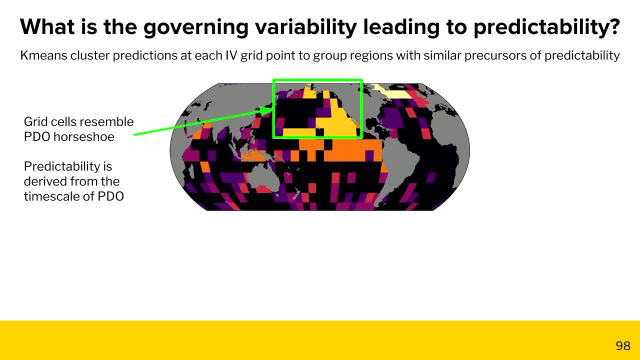 the variability at these points showed that this predictability was derived from the time scale of the PDO. We find a cluster that resembles which is in the tropical Pacific or in the ENSO region, and this appears to be predictability from sort of an aliasing of an interannual El Nino. 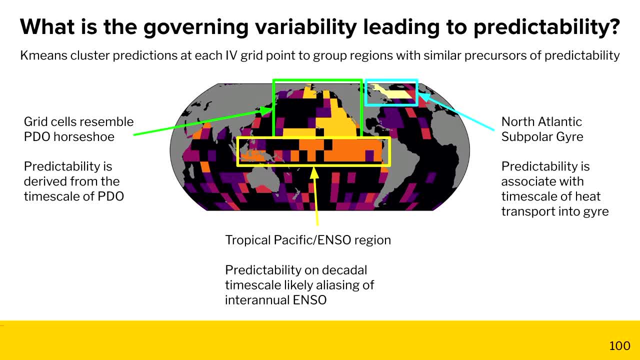 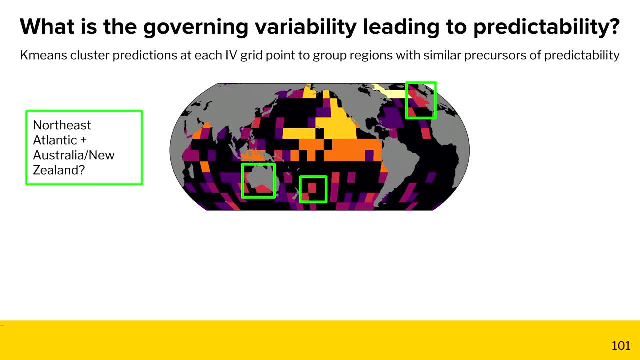 variability. And then we also find predictability in the North Atlantic sub-polar gyre. once again, this is the time scale of ocean heat transport into the gyre, But we also have these sort of remote clusters falling out, so we have this sort of one which 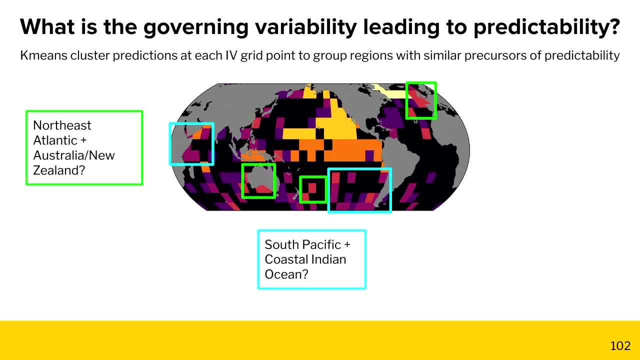 highlights points around Australia, New Zealand and sort of off the coast of Europe. We have this sort of South Pacific and coastal Indian Ocean cluster and we have also a subtropical Atlantic, subtropical North Pacific. So this is another interesting question to me. once again, we've had this sort of remote. 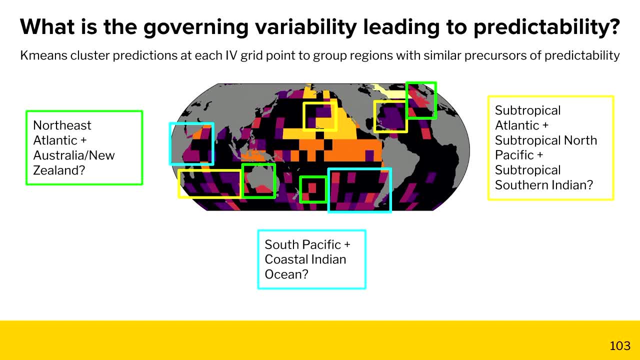 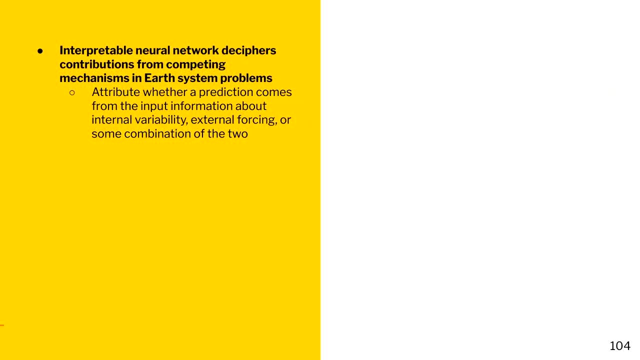 regions which are co-varying at the same time, when we have predictable signals. so what is leading to this co-variance in predictability? So, summarizing this section, we've designed this interpretable neural network to decipher contributions from competing mechanisms in the Earth system, to examine sort of attribution. 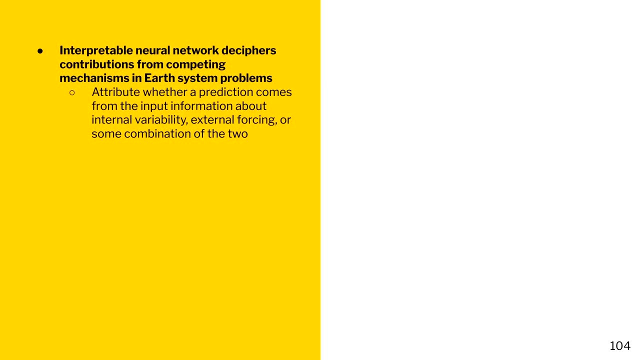 to predictability. So in this case, looking at internal variability and external forcing, We find that internal variability contributes to predictability even in a moderate to high forcing scenario. So in this case, it was the northern mid-latitude oceans and the tropical Pacific. yes, they. 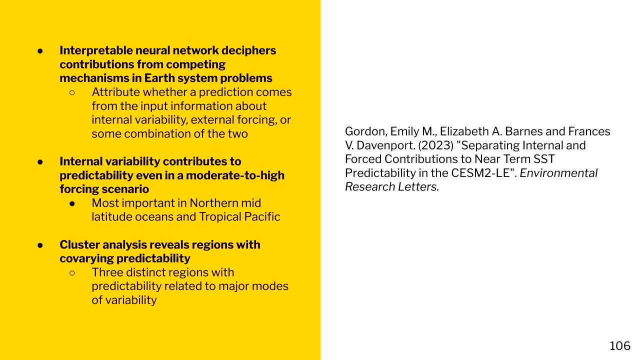 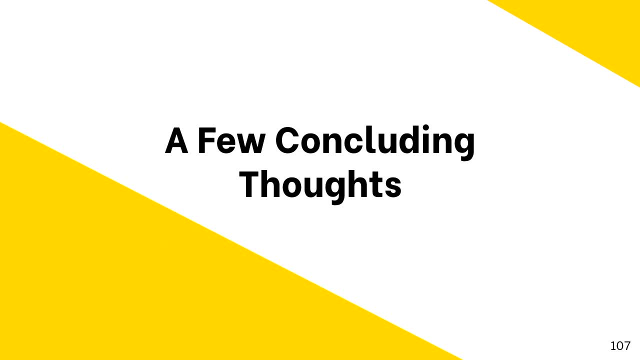 were important And cluster analysis has revealed the regions with co-varying predictability, and the study is in environmental research letters. So I have sort of a few concluding points. So I have sort of a few concluding points. So I have sort of a few concluding points. 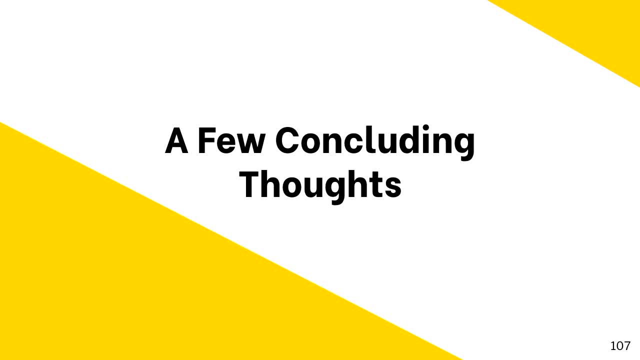 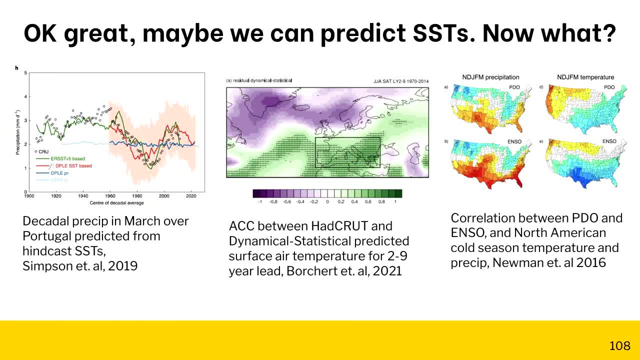 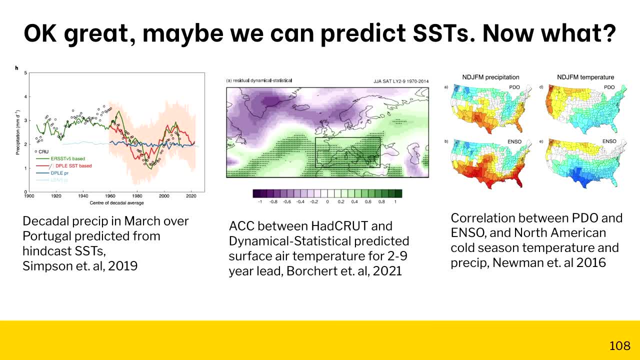 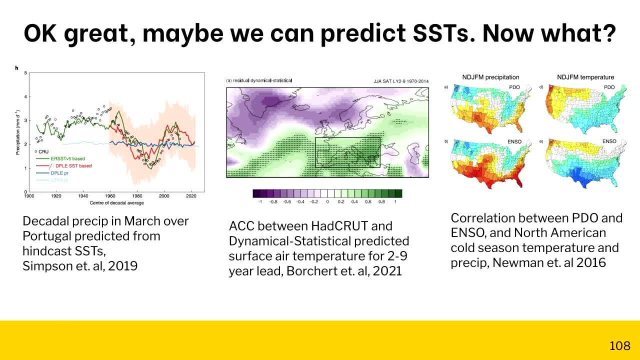 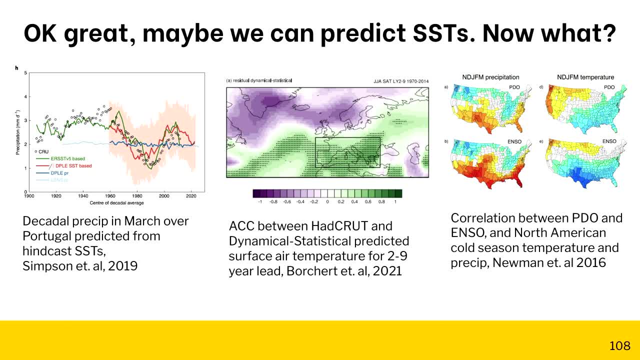 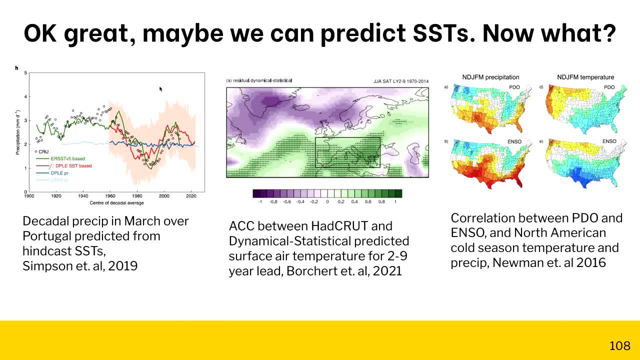 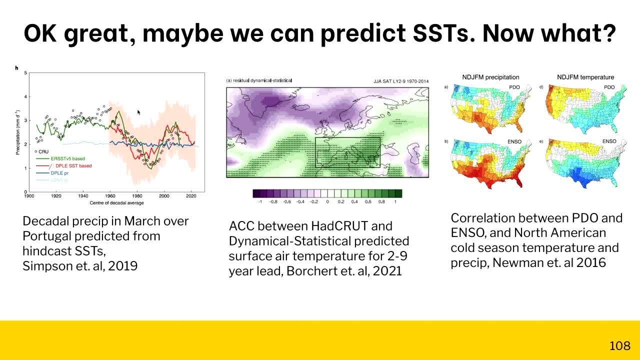 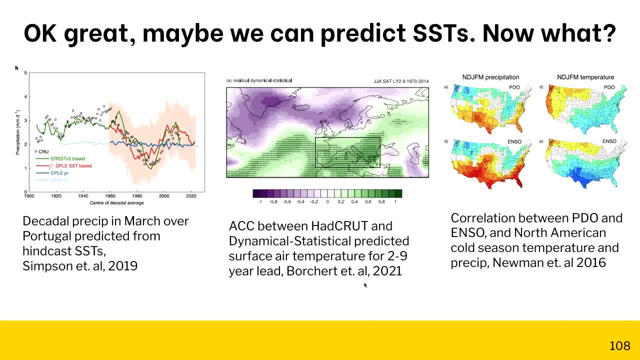 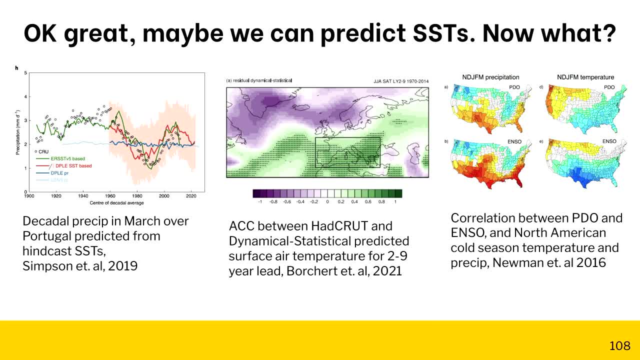 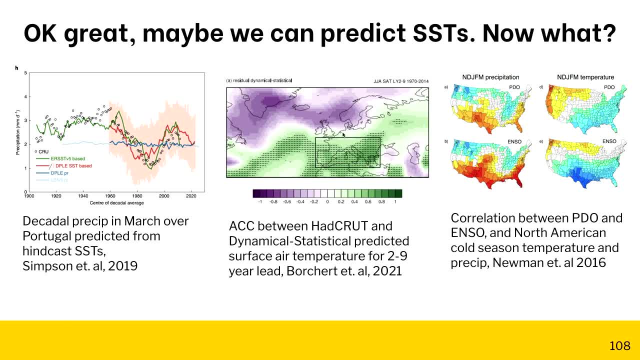 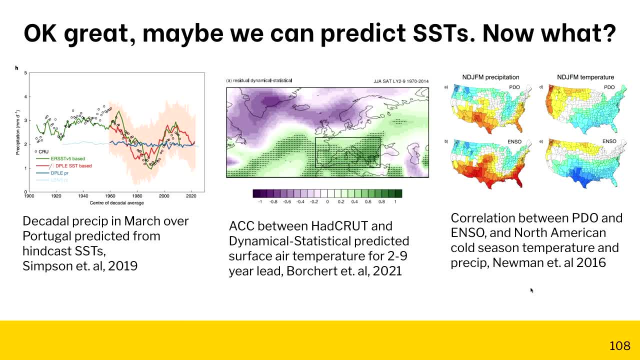 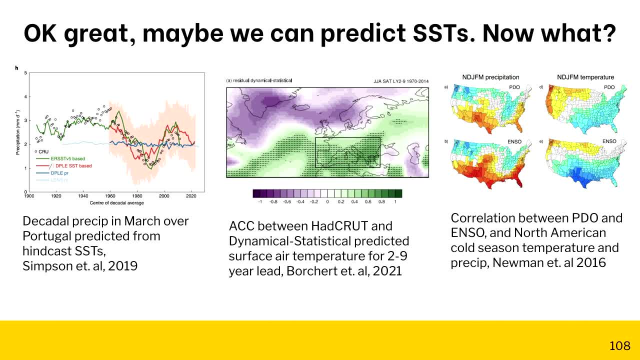 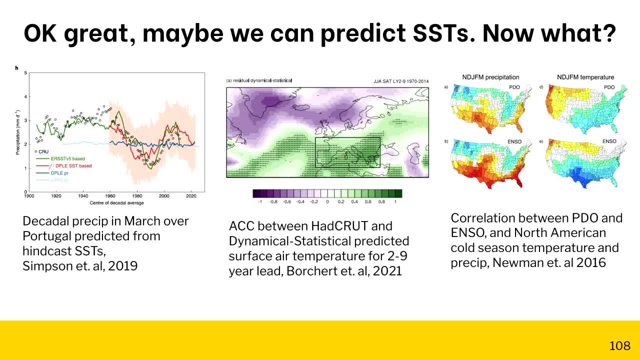 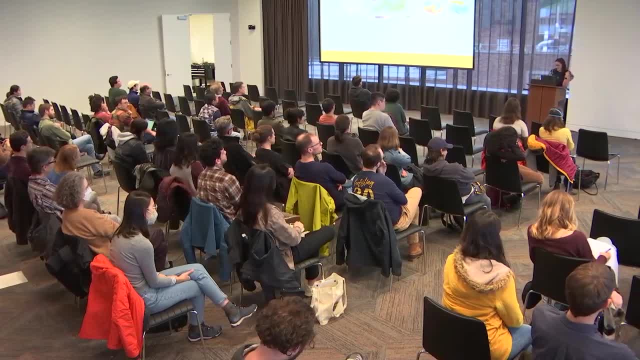 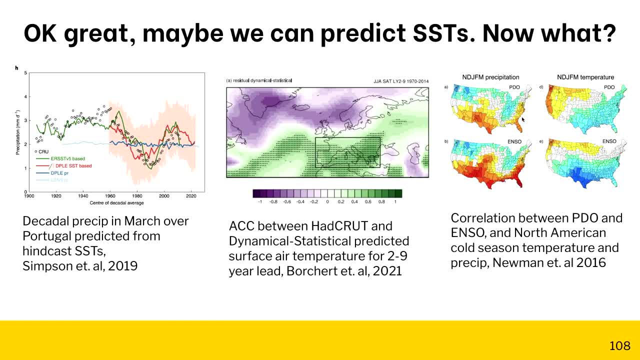 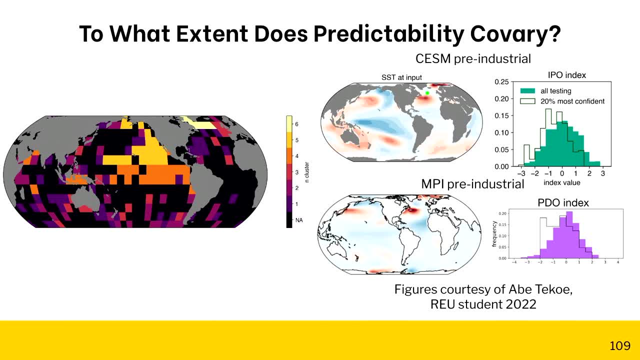 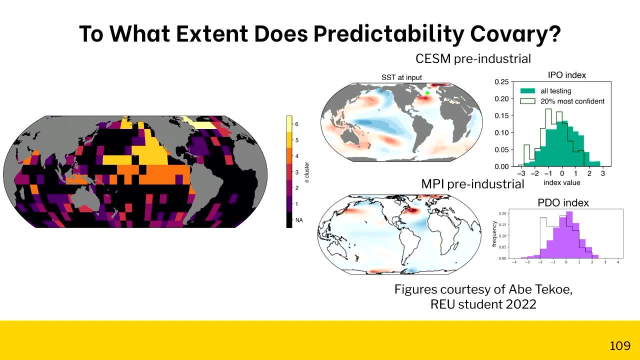 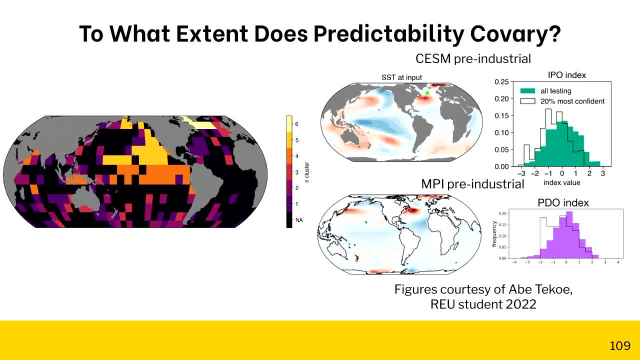 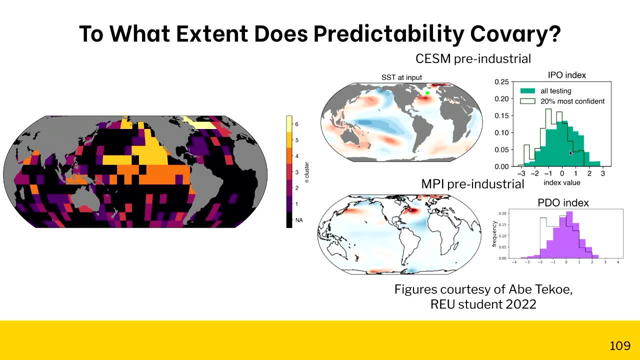 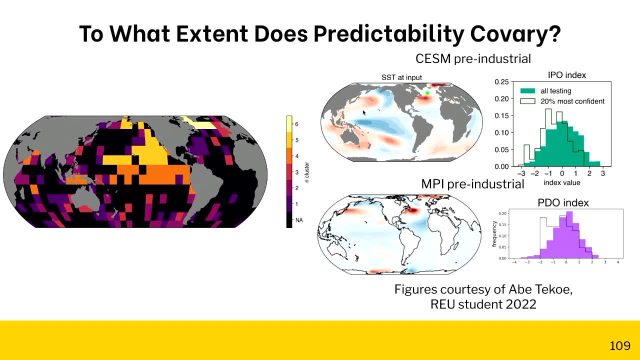 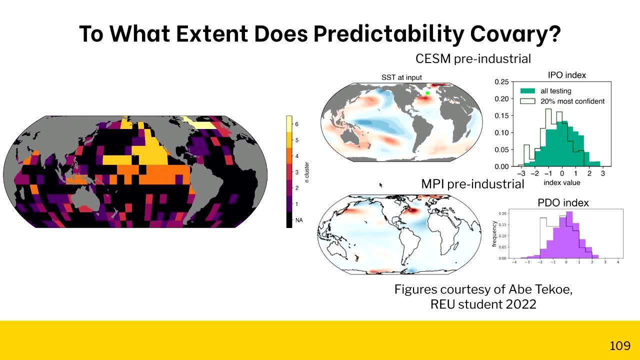 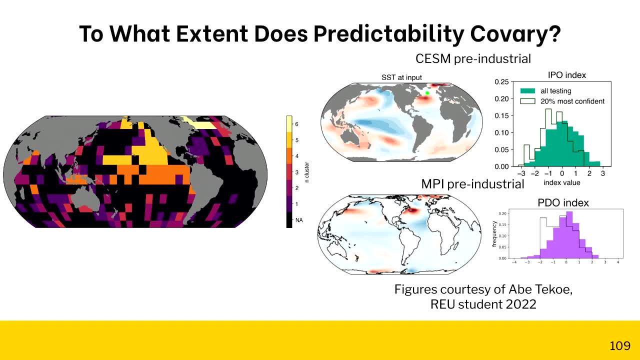 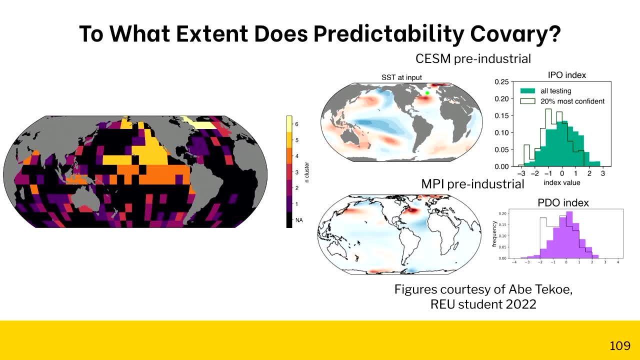 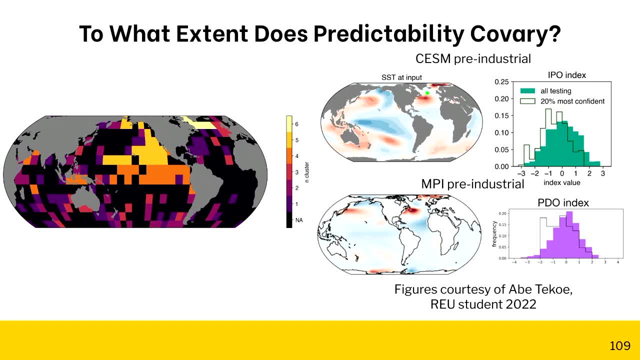 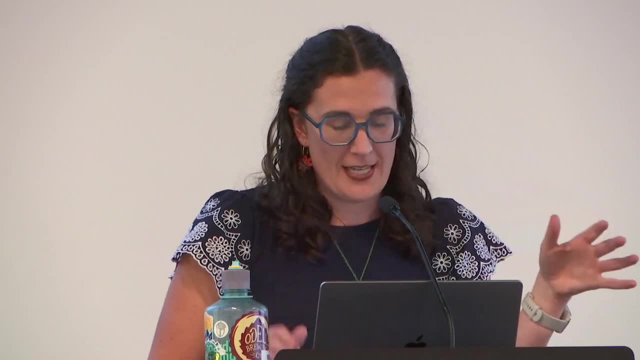 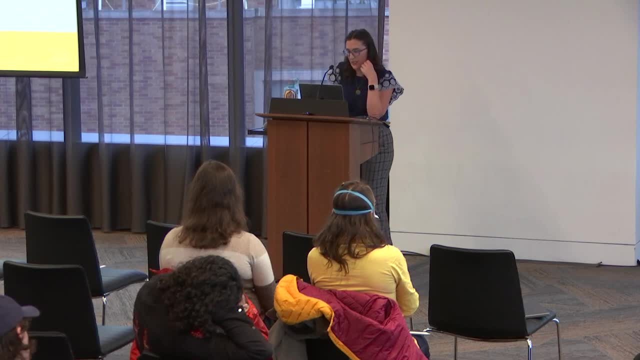 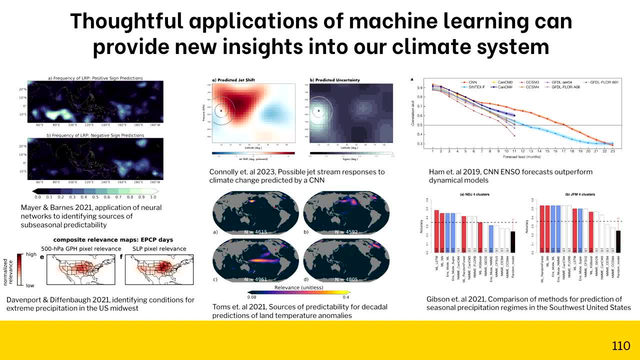 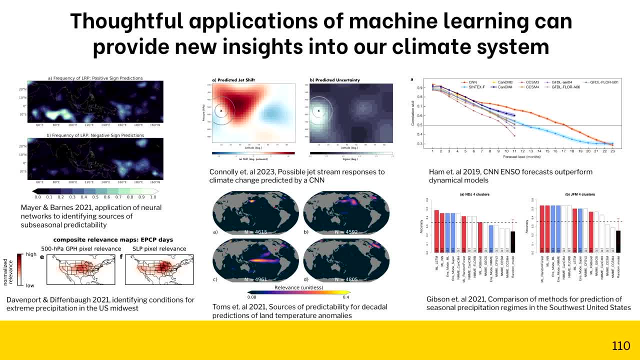 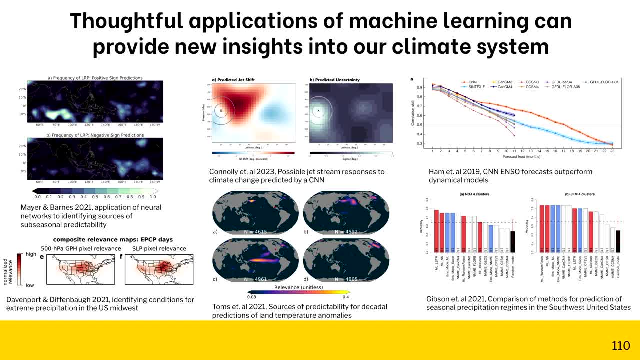 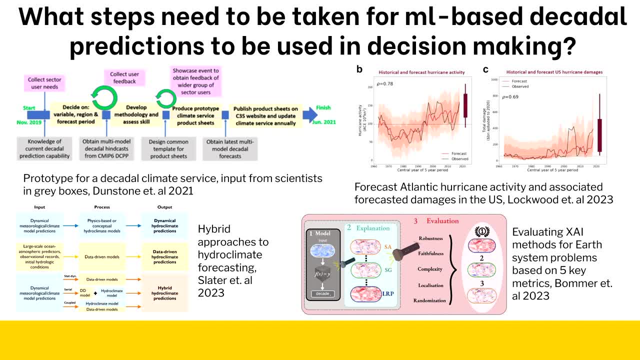 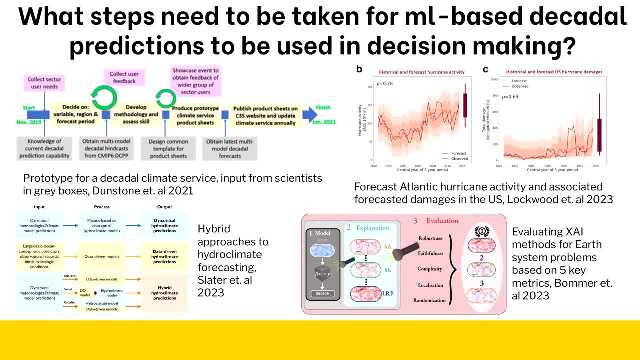 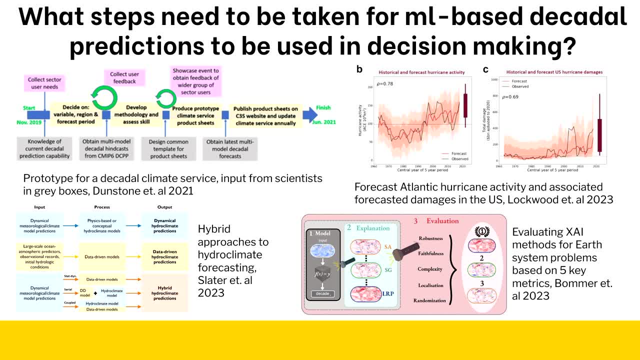 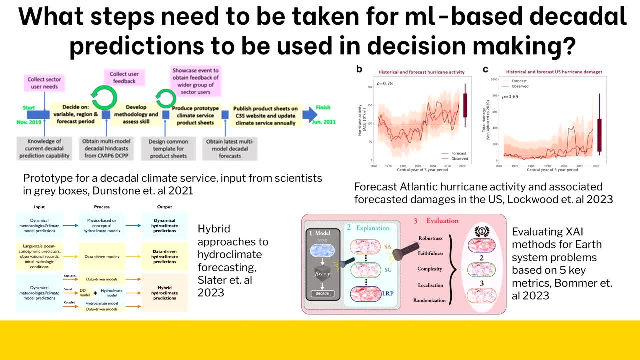 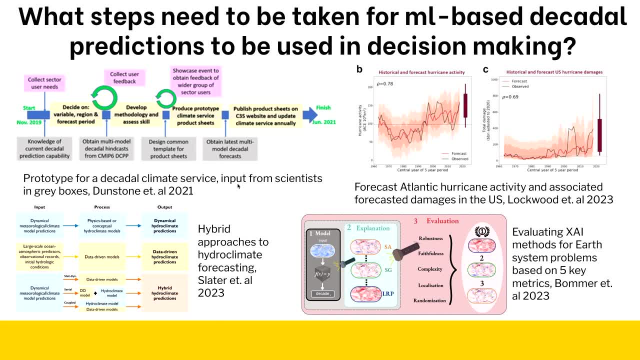 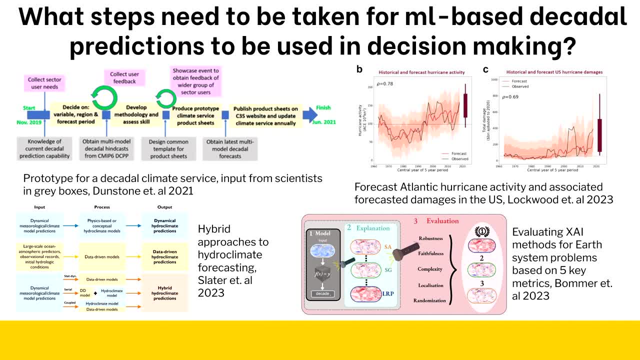 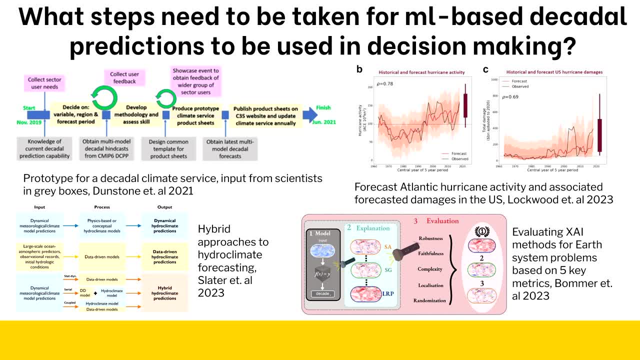 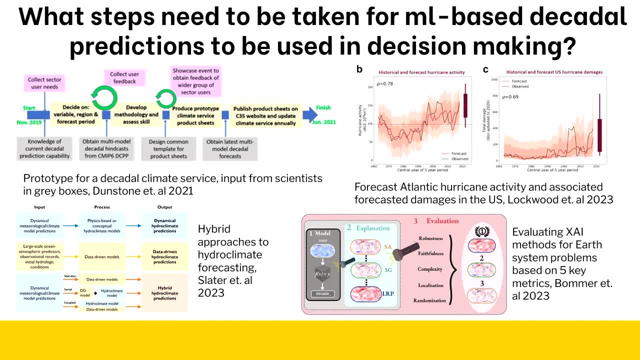 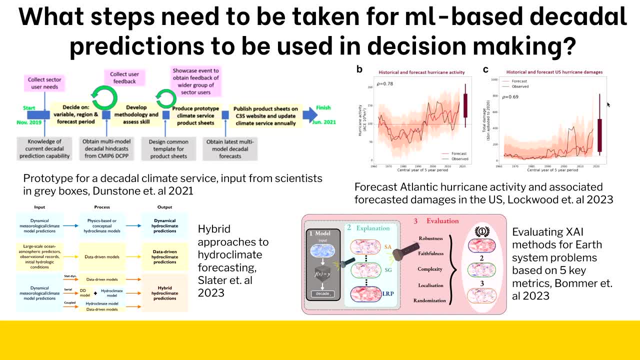 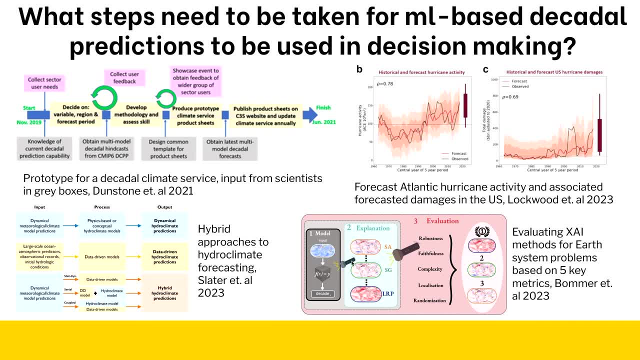 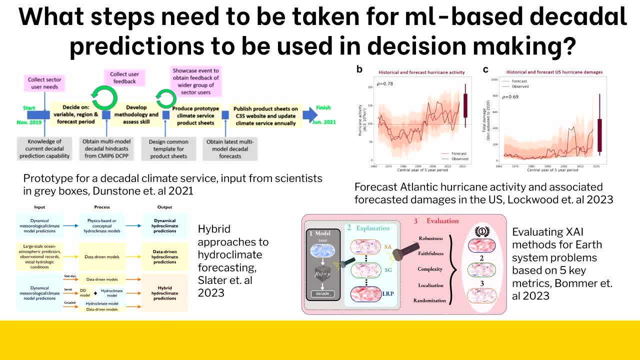 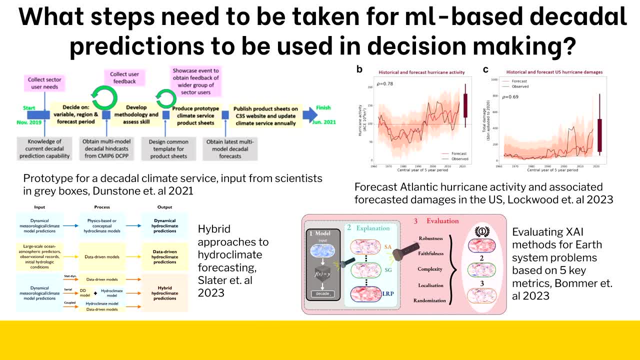 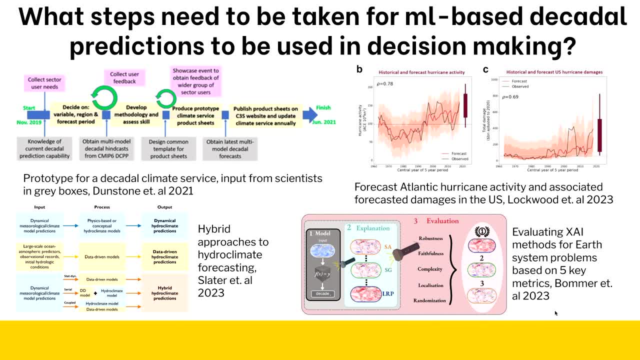 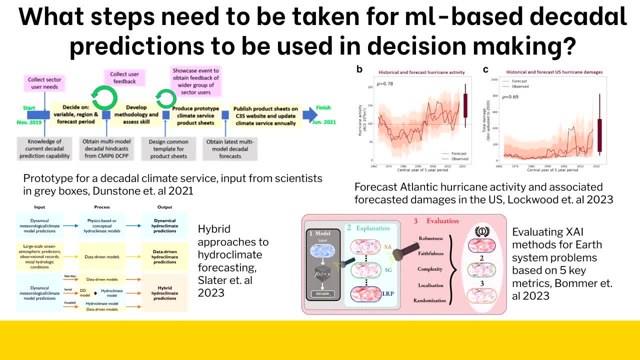 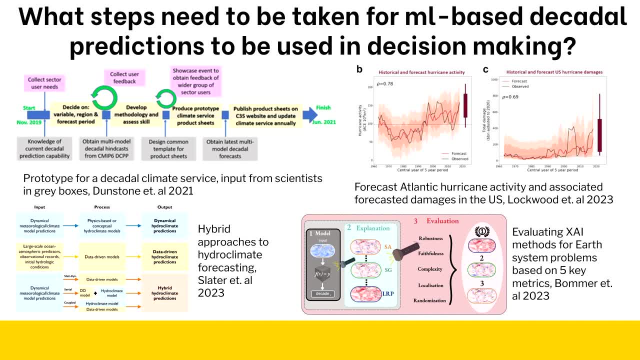 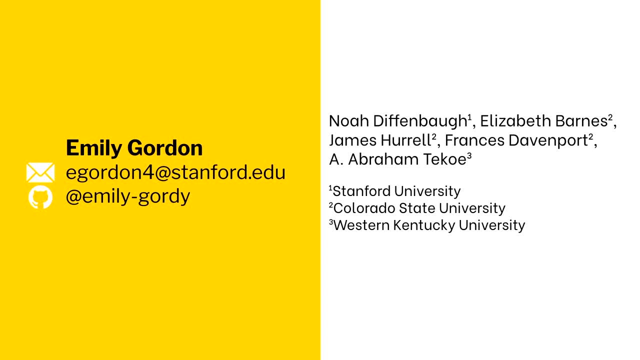 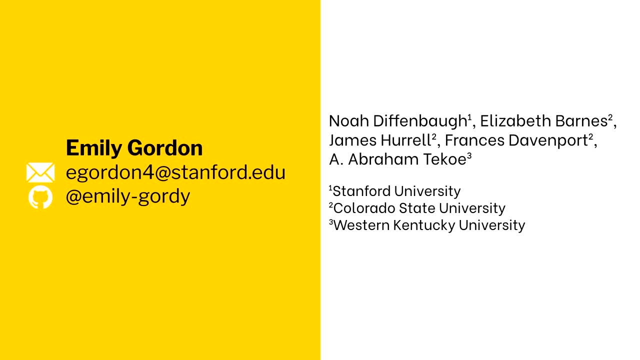 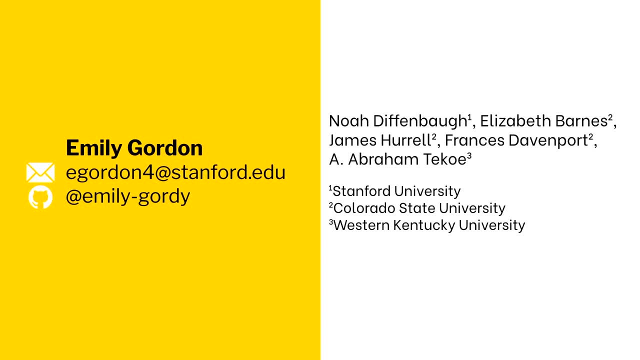 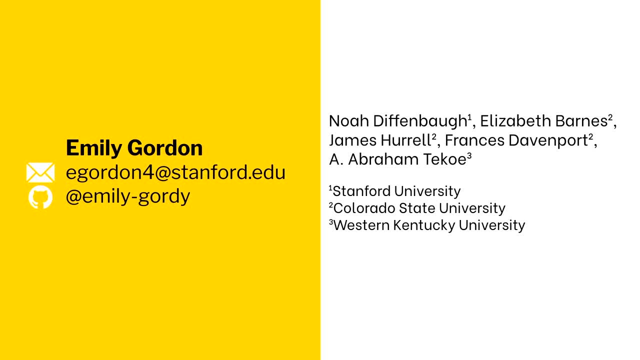 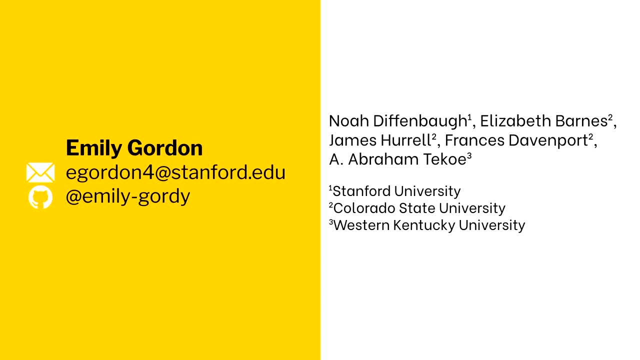 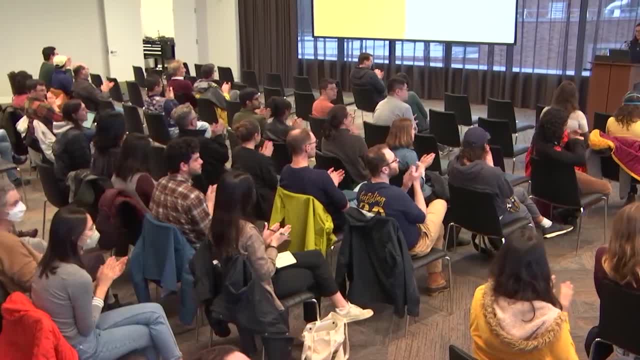 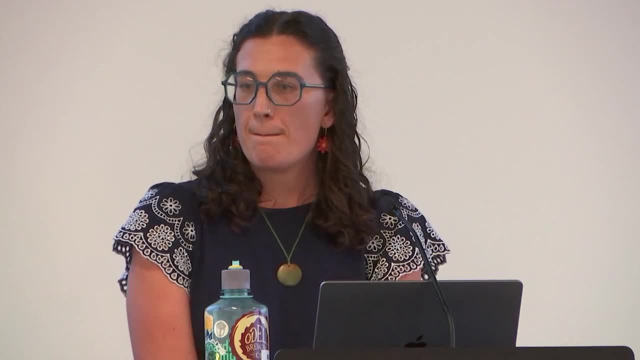 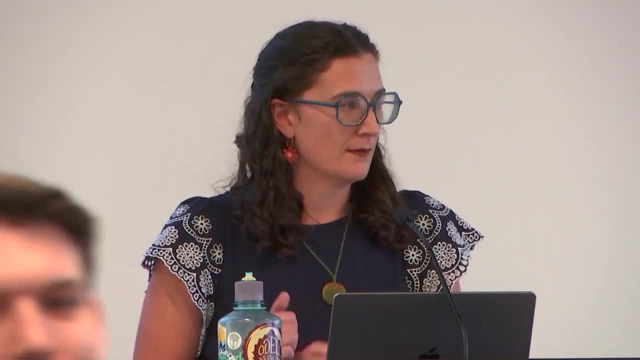 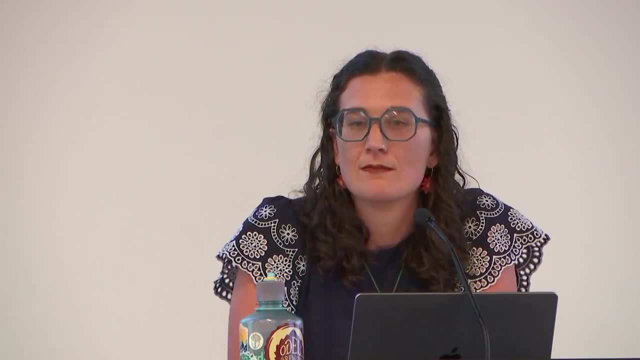 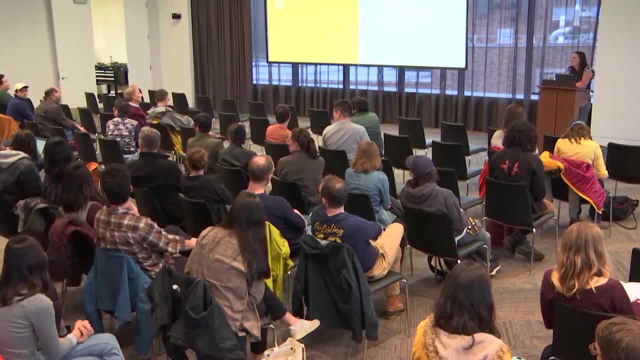 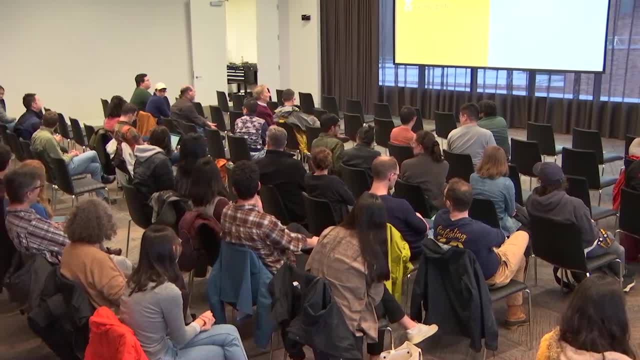 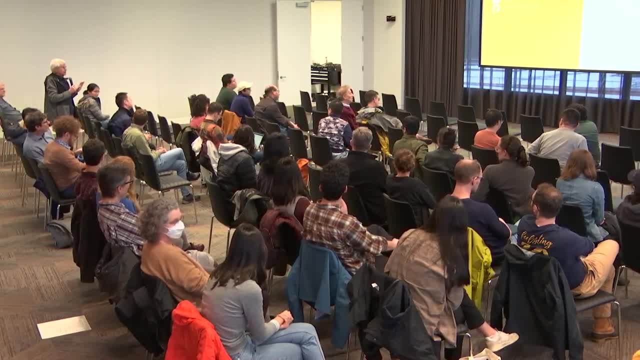 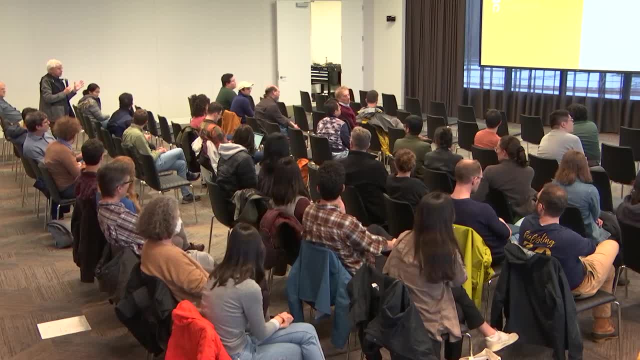 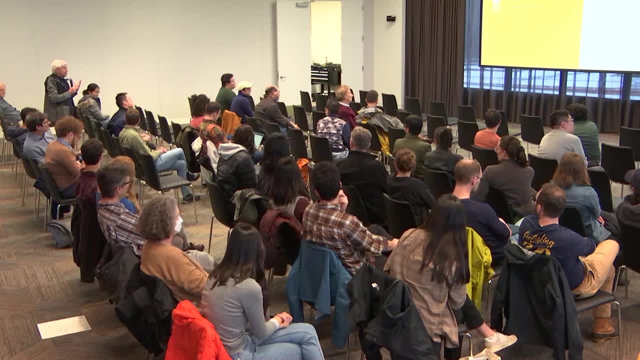 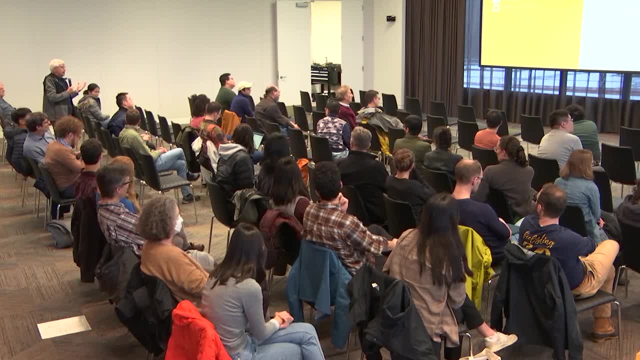 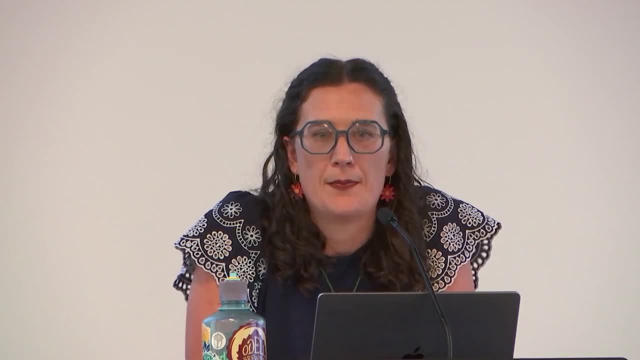 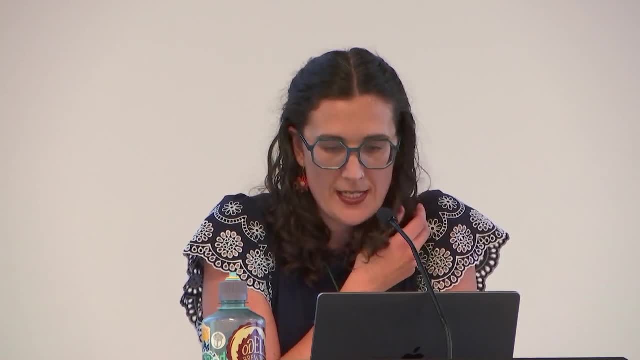 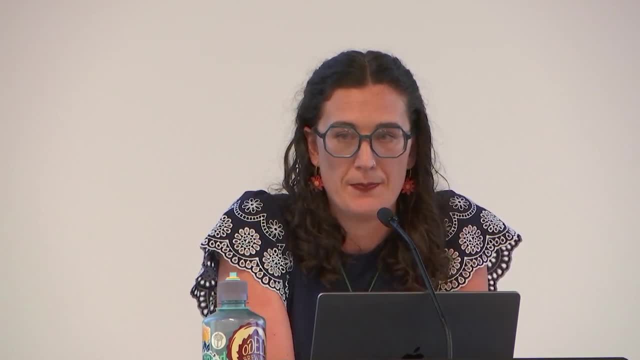 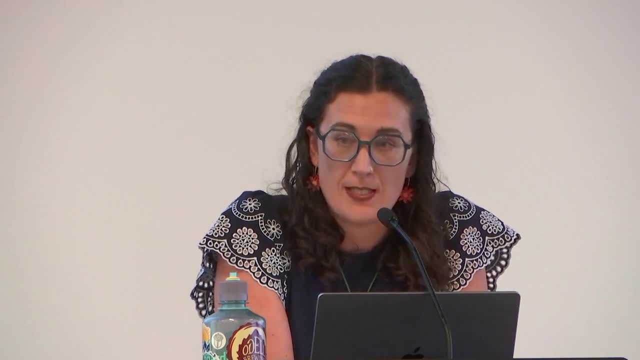 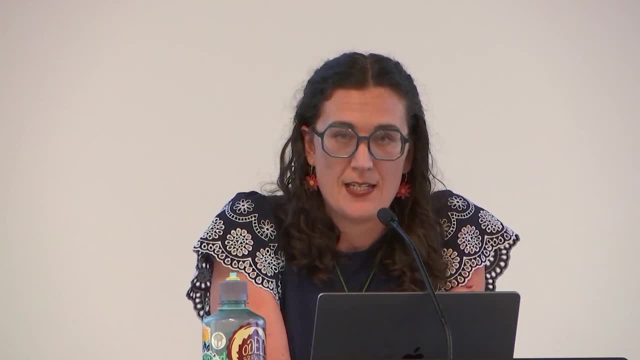 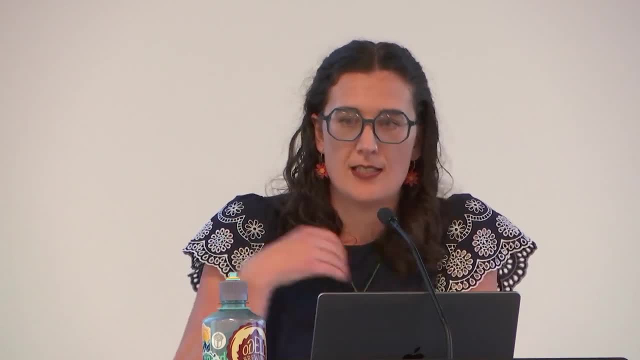 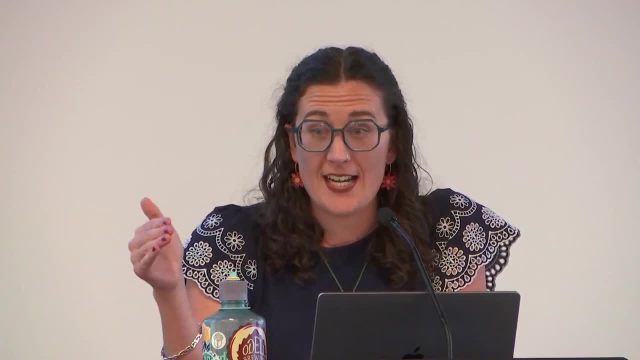 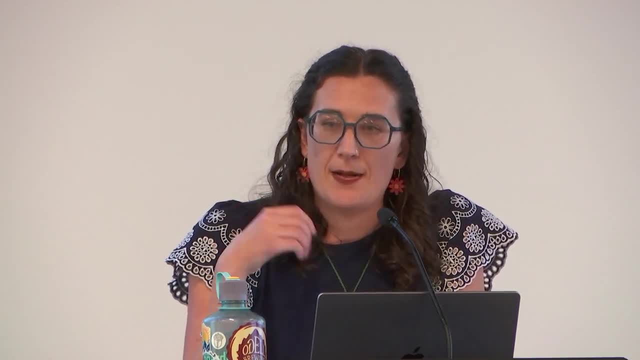 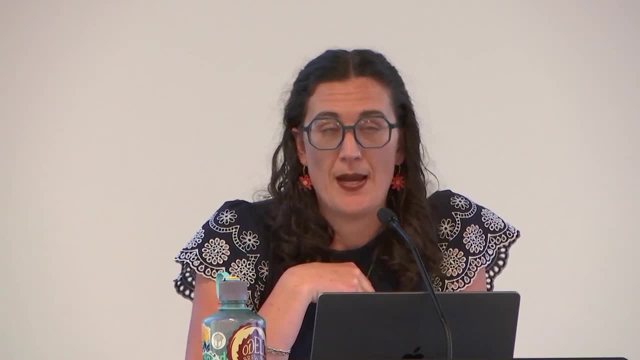 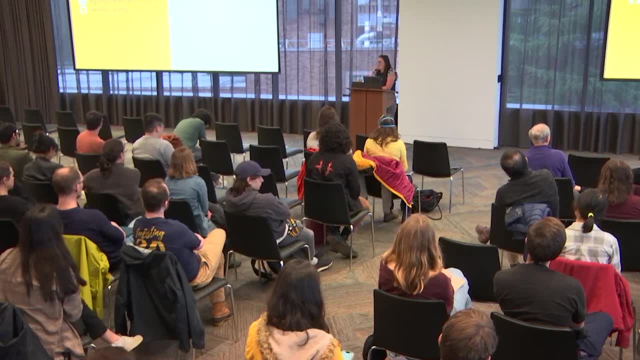 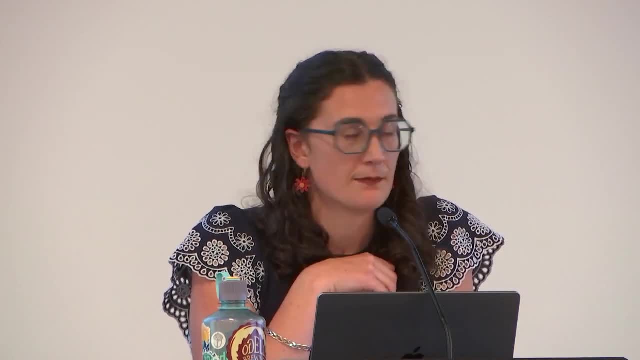 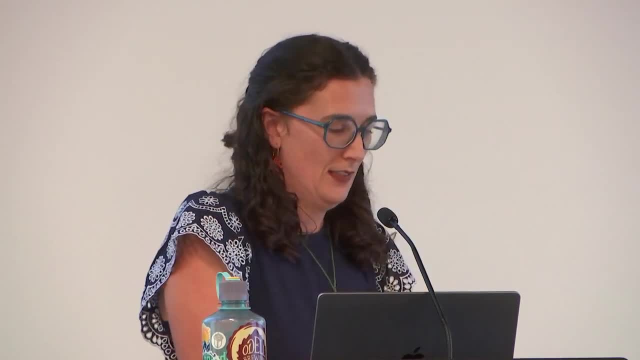 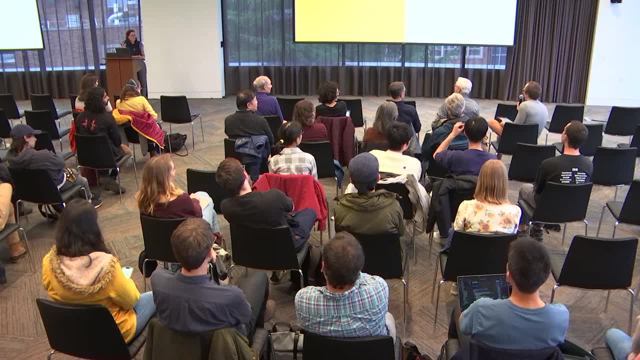 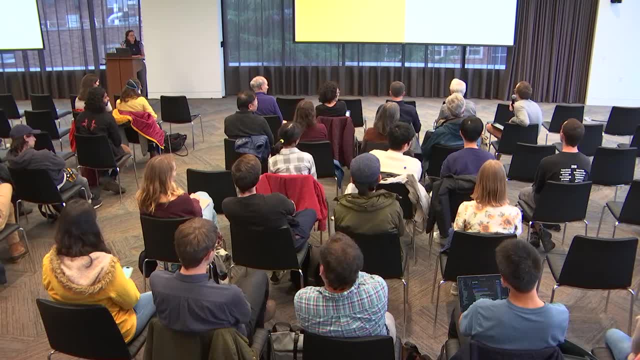 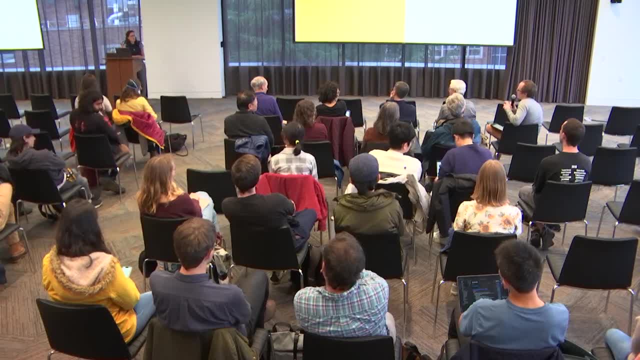 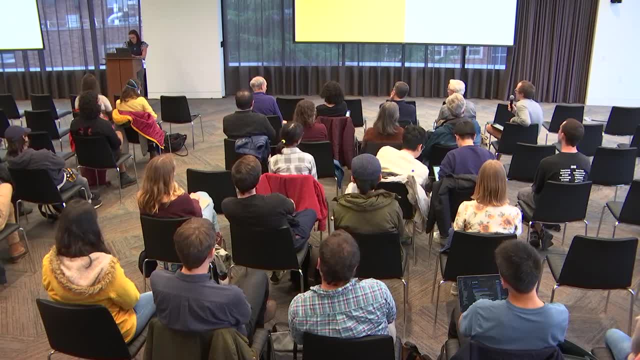 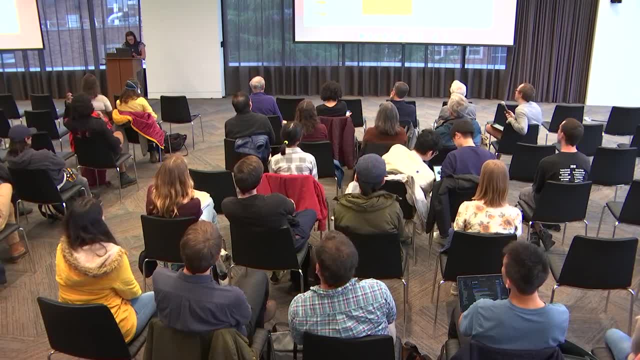 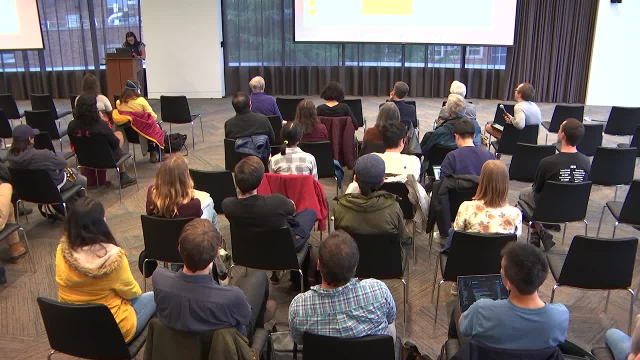 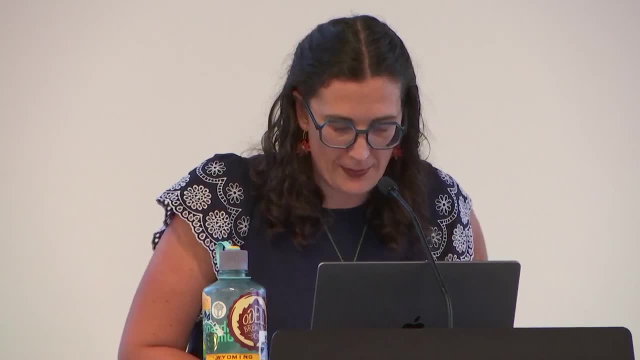 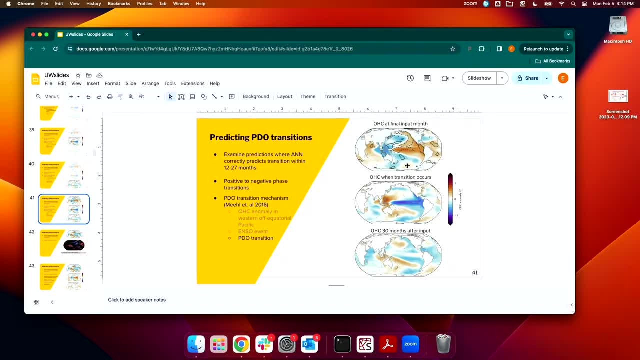 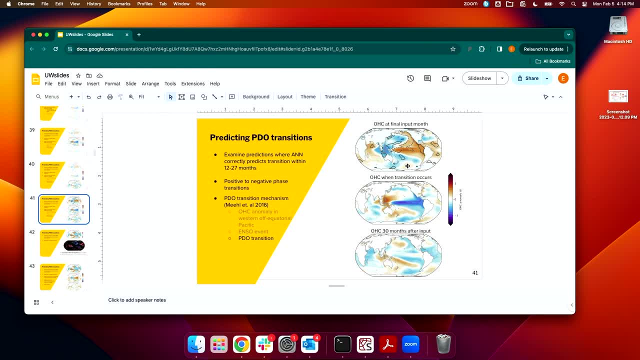 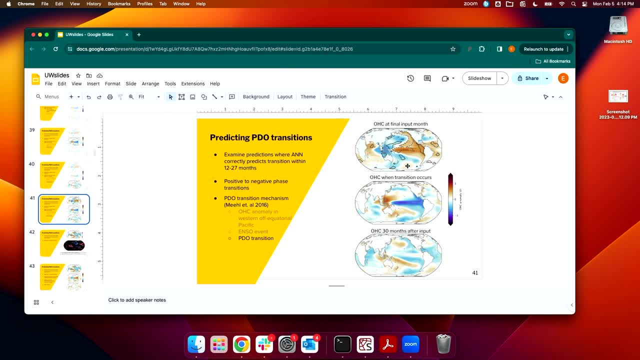 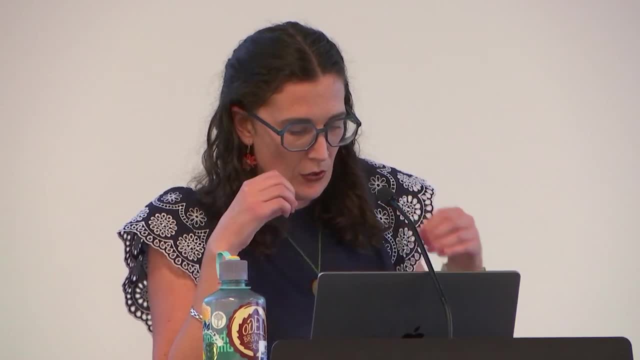 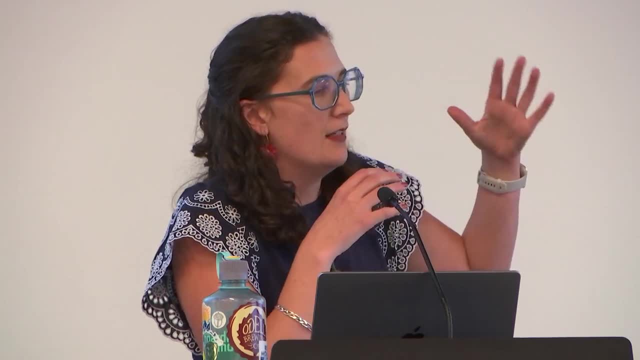 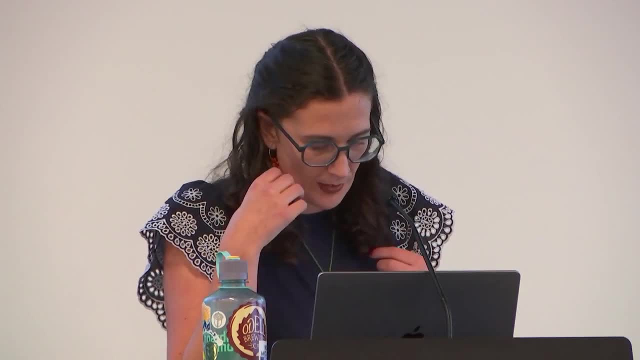 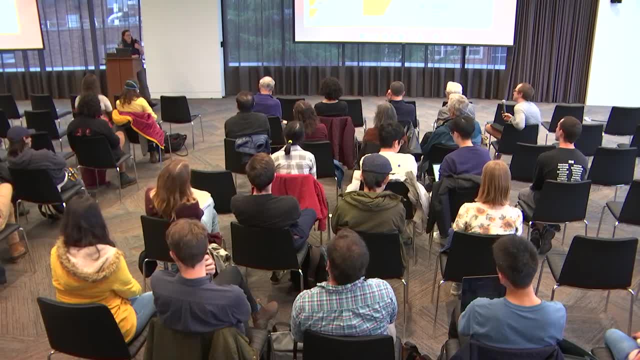 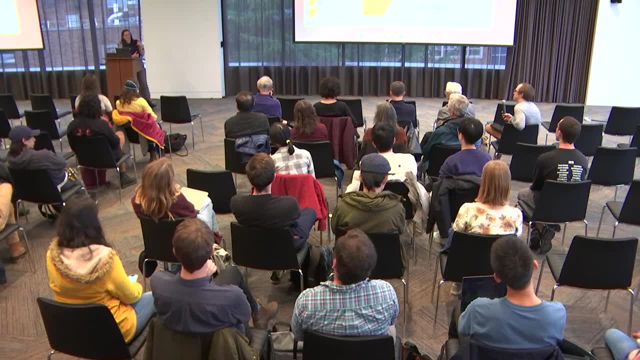 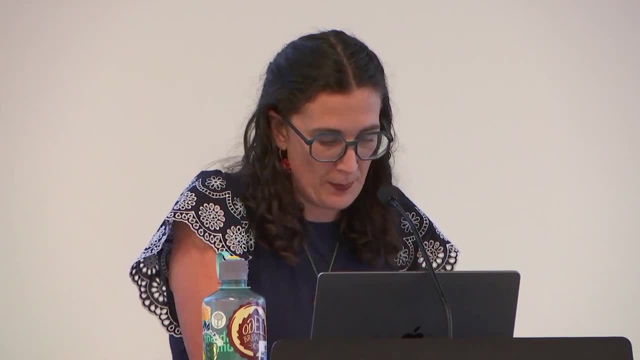 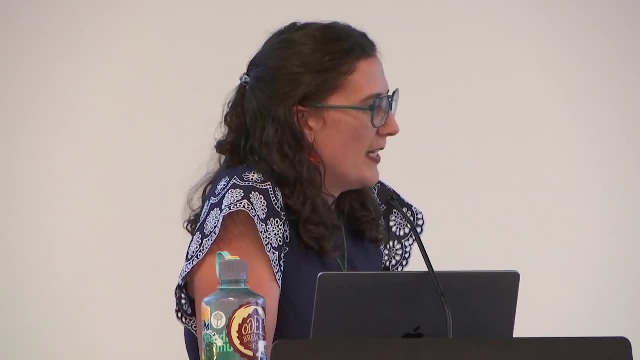 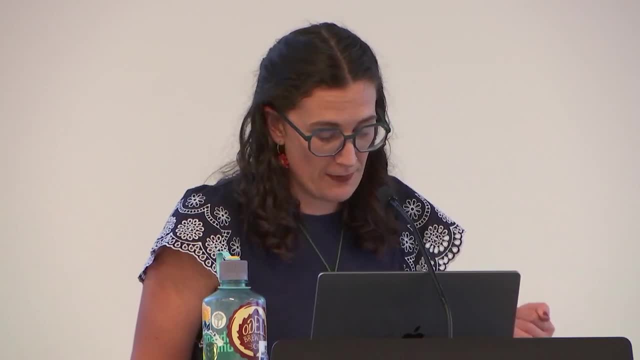 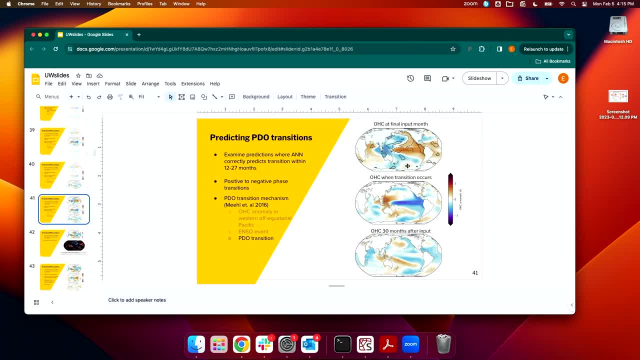 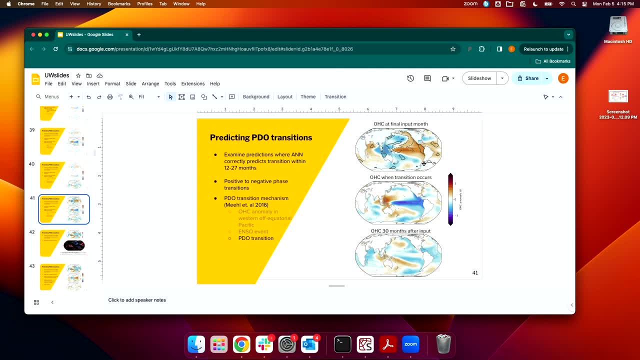 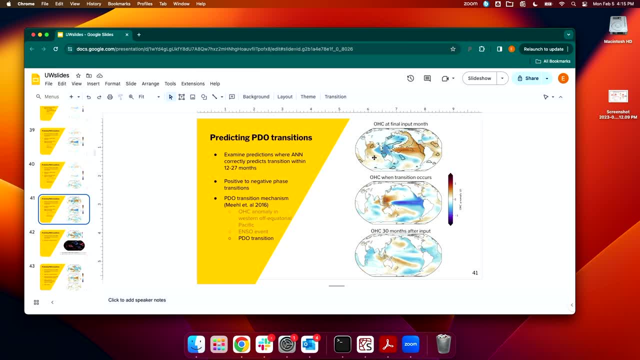 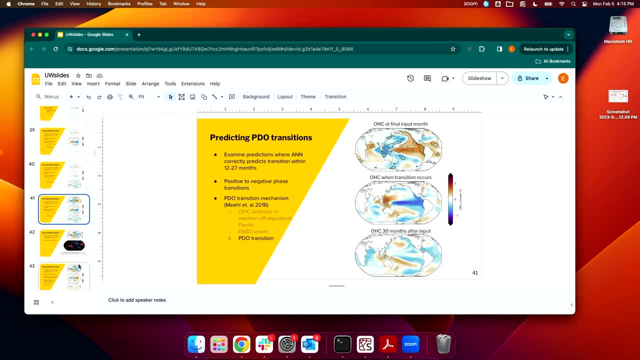 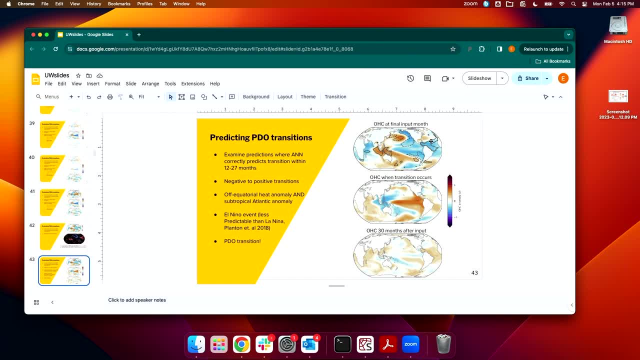 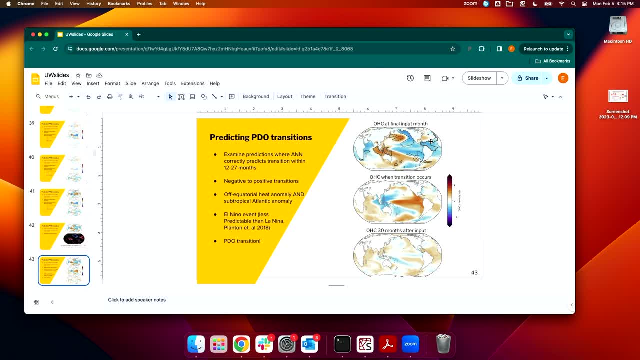 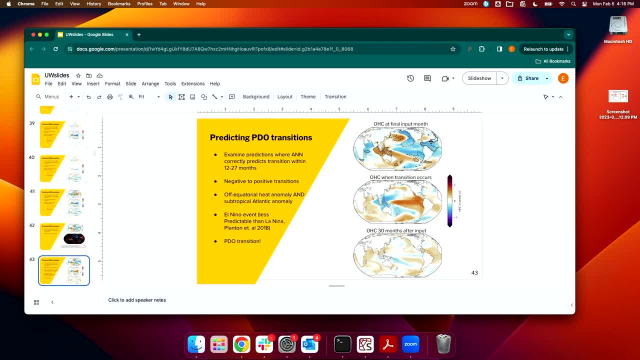 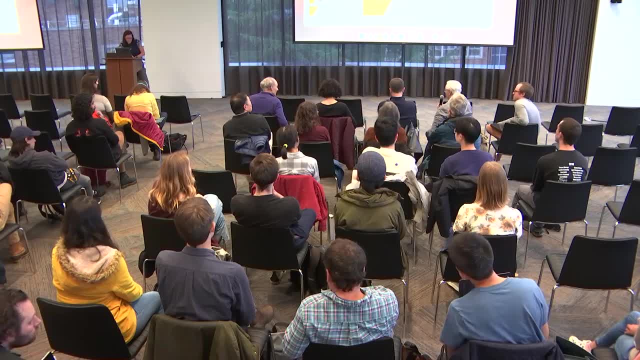 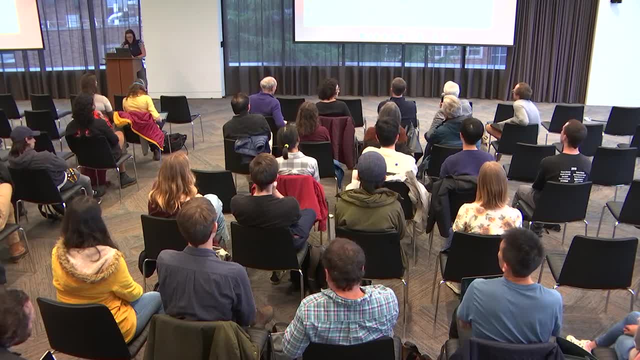 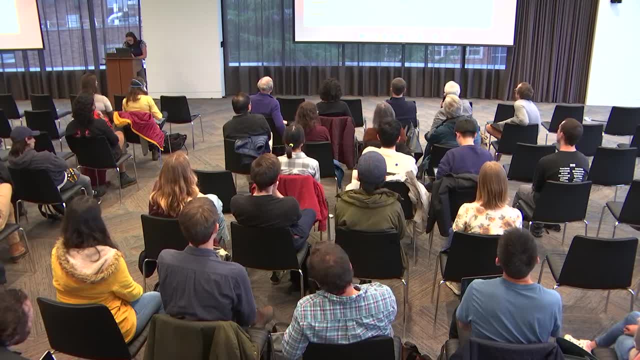 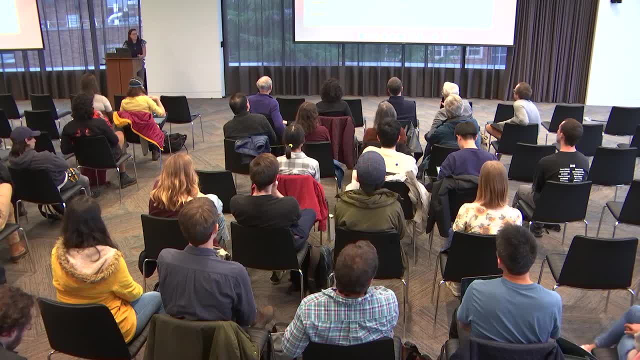 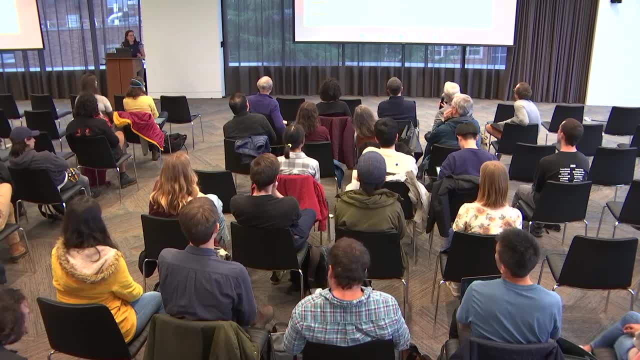 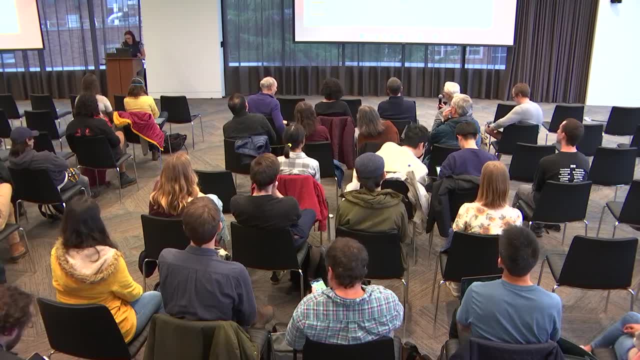 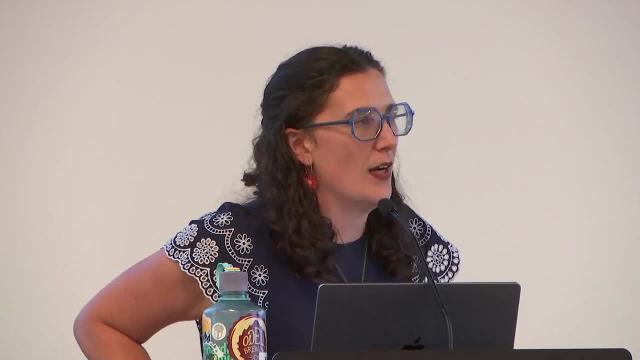 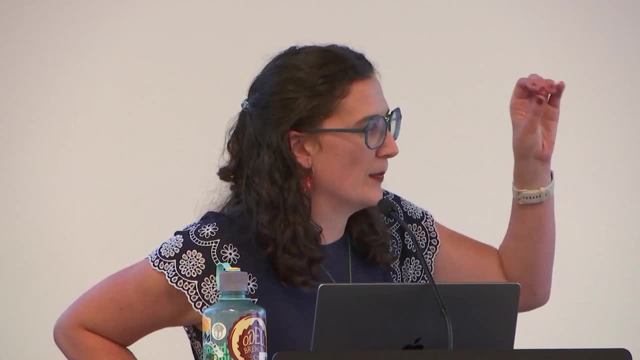 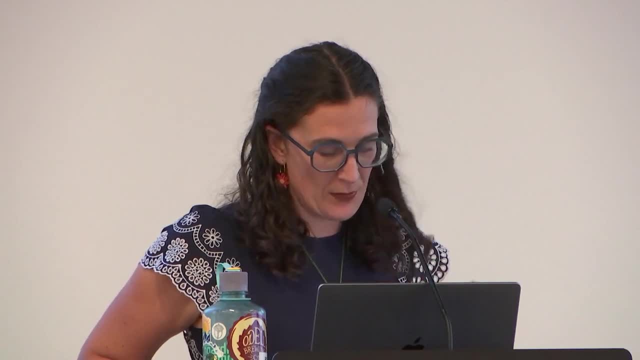 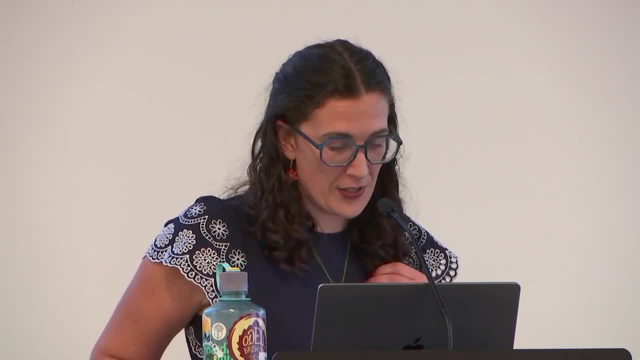 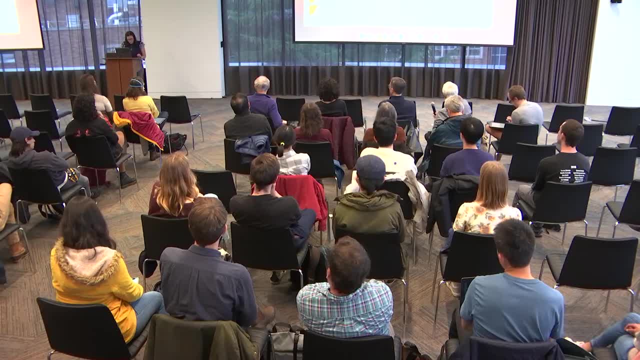 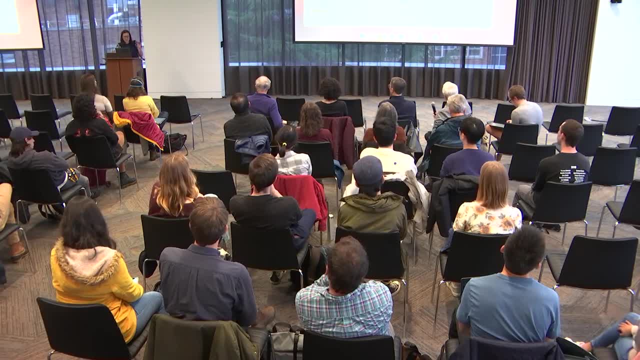 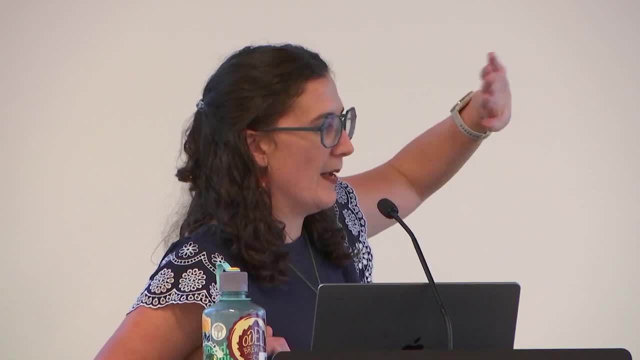 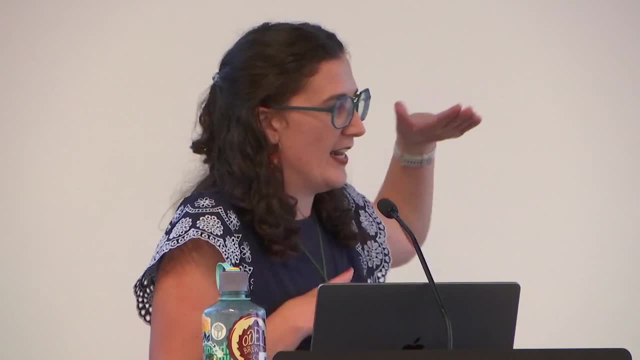 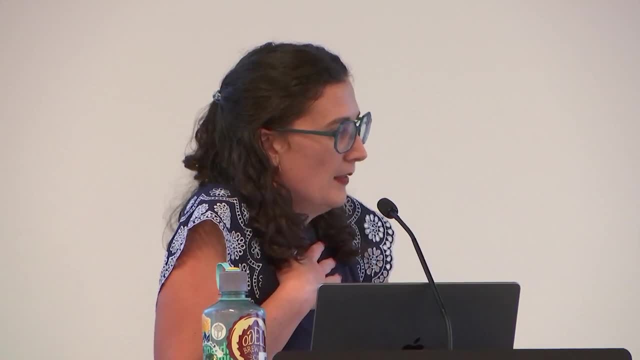 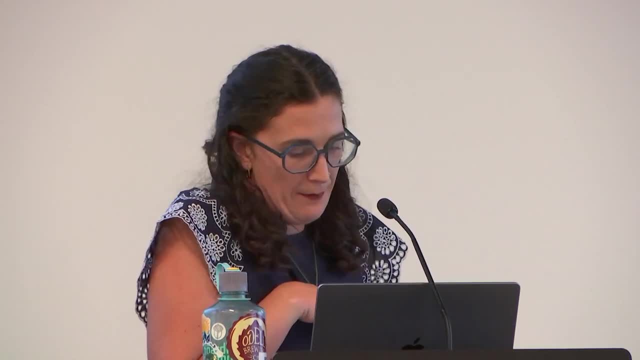 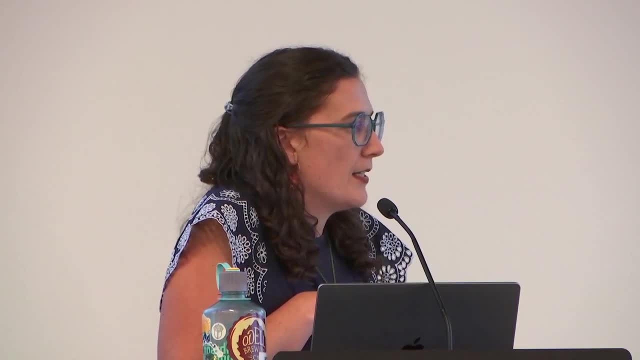 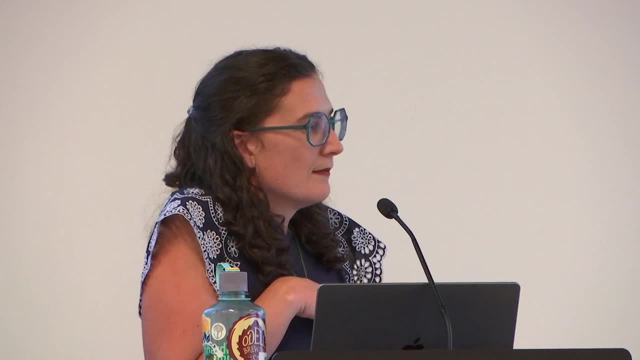 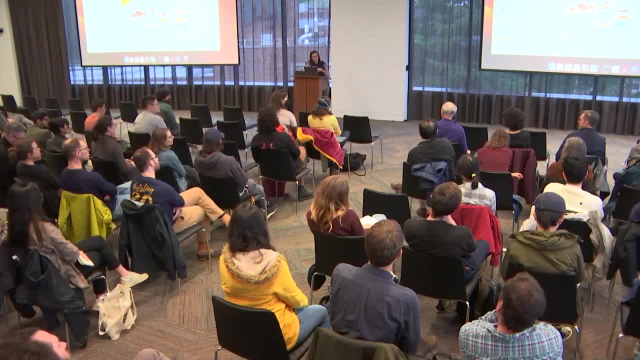 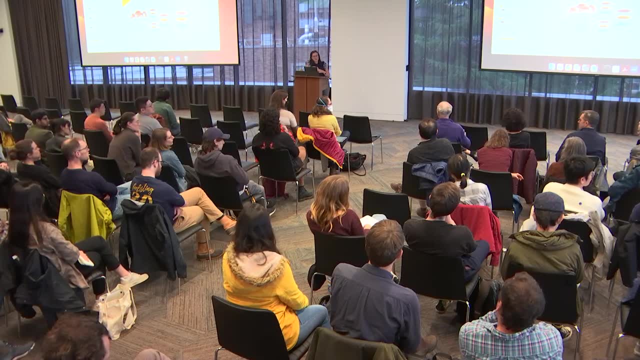 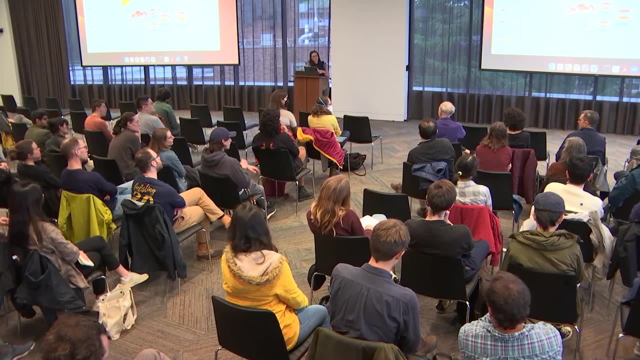 to do with decadal variability. One of them is the cause of the AMO and how important that anthropogenic aerosols might be. And then the other one is, say, the specific variability, and to what extent is it an internal variability that's driving us into a particular phase, and to what extent is it, say, teleconnections? 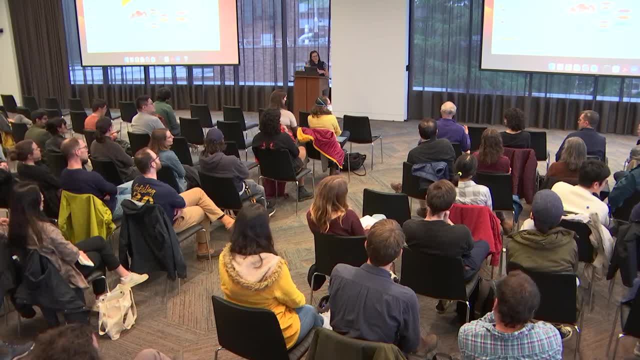 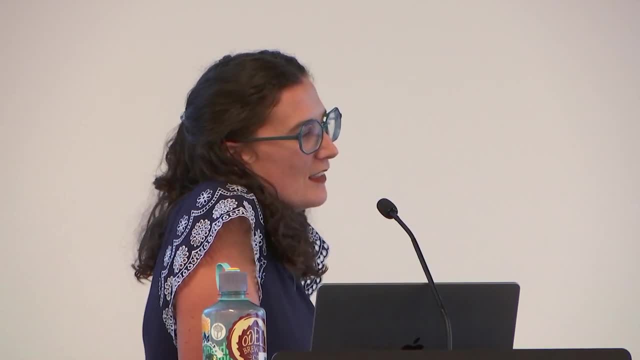 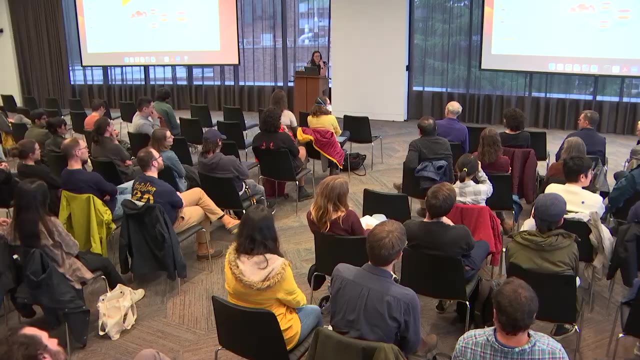 with Antarctica, et cetera. Does machine learning help us with any of these questions? I mean, there are lots of interpretability metrics, but I guess I'm wondering interpretability in the classical science sense of mechanism? how can you make that connection? 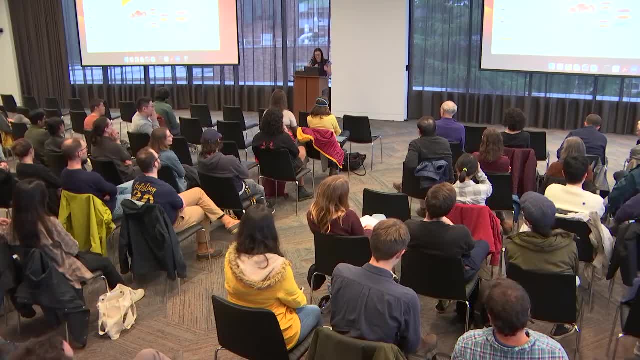 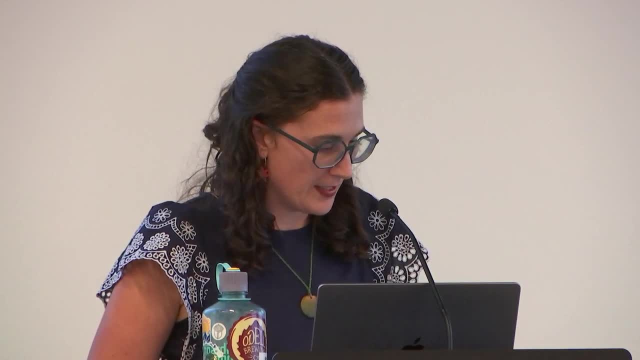 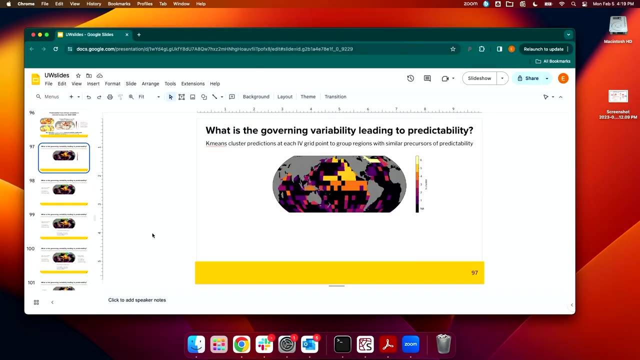 Yeah. so in terms of my own research, I can only guess. I can only point to this clustering I did, where the variability leading to predictability in the North Pacific was distinct from the variability in the El Nino region, suggesting that they are different, so suggesting that it's not just ENSO driving North Pacific variability. 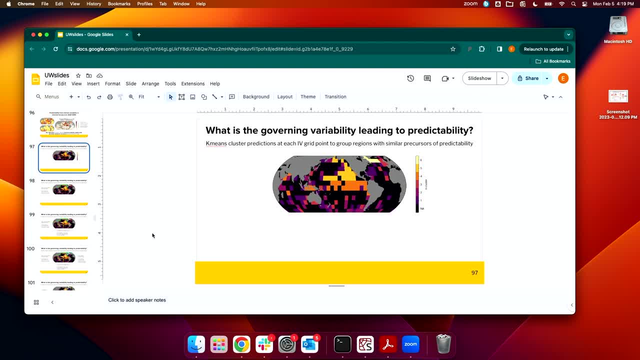 And that there is a difference in the variability that is the same in the north Pacific region. So it's not just about the variability leading to a different type of characteristic. It's about pulling out the governing modes of variability for the governing variability for AMV. 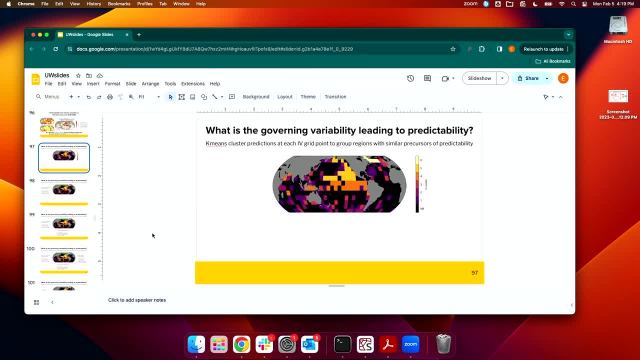 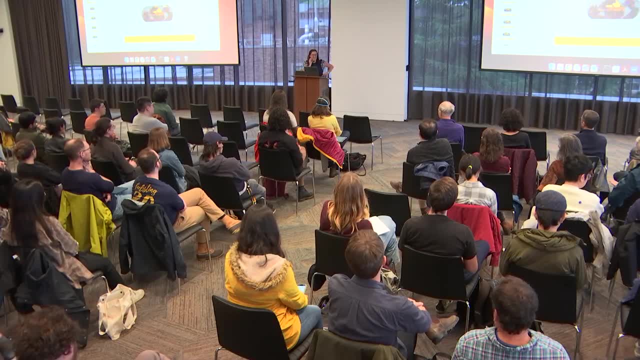 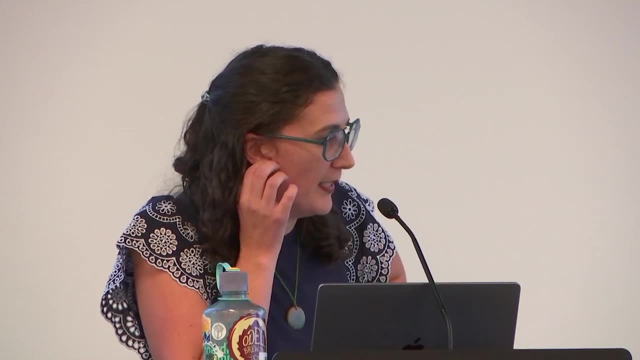 I haven't thought a lot about that. I've been thinking mostly so, using these pre-industrial runs so that we sort of don't have to worry about this problem with the forcing. And from this I sort of take the opinion that there is internal variability internally. 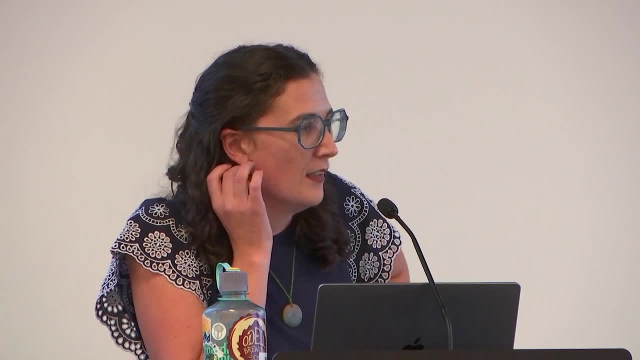 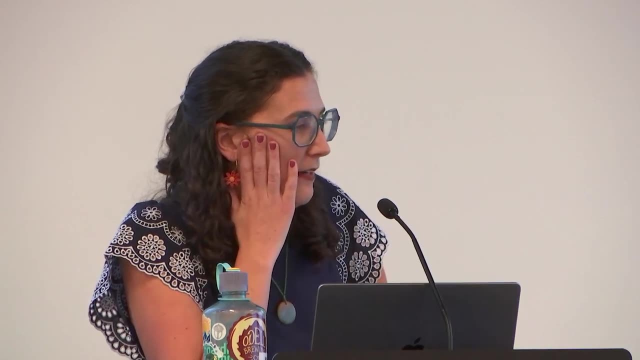 generated variability in the North Atlantic Ocean, But to what extent does it impact the environmental? I can't get to that yet. Has it just been sort of swamped out by changes in anthropogenic forcing is a question I don't know the answer to. 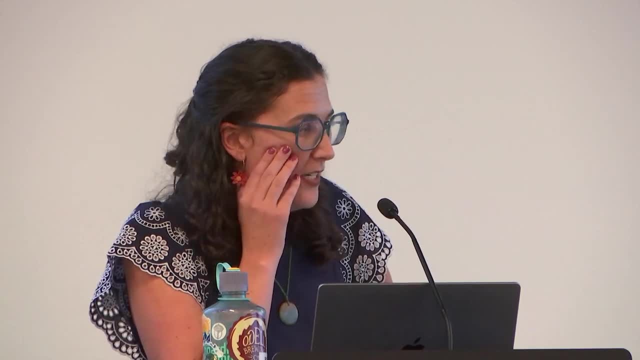 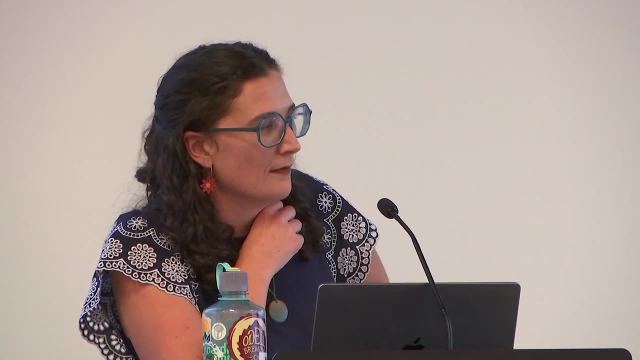 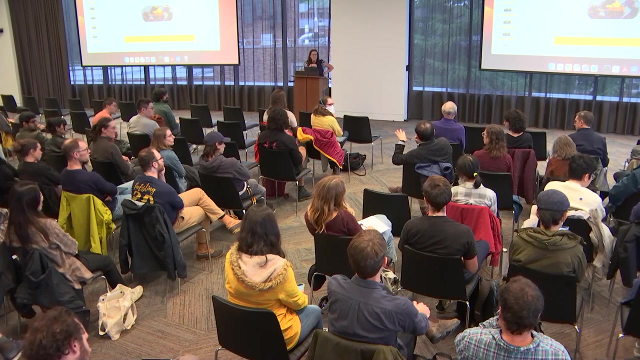 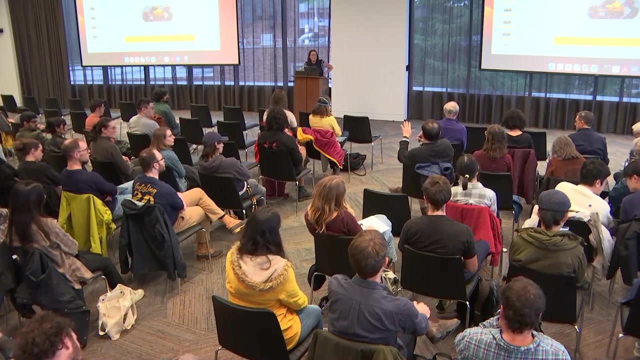 And I'm interested in thinking about ways that we can use existing data and data-driven methods to tease out those mechanisms. Yeah, thanks. So in your prediction model, is your initial state? is that given time- or at many times, I would guess- in order to predict what's happened in the next 10 years, if you use all 40 years? 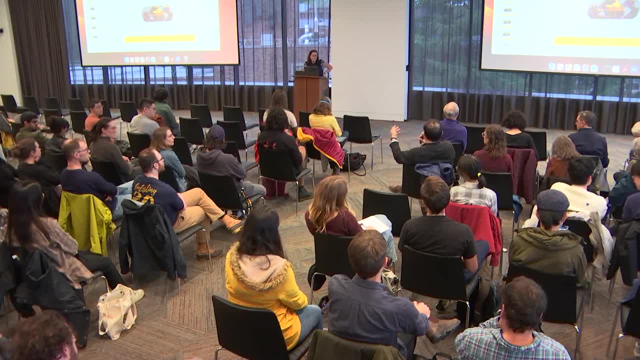 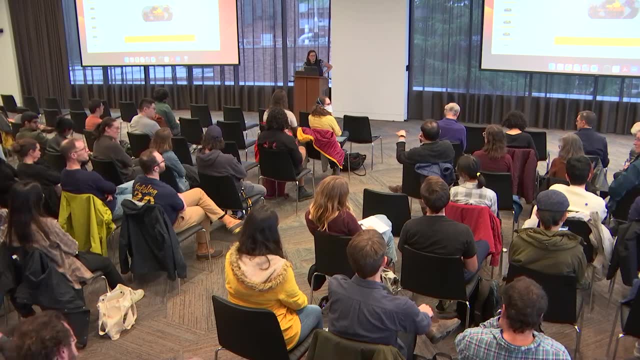 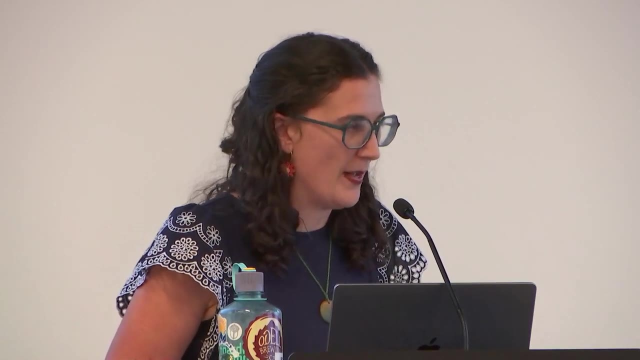 data before. from satellite we would expect better predictability And my question, if so, how sensitive to the different time of initial days you use? Thanks, Yeah, So in each of my studies I used slightly different models. I used different amounts of information. 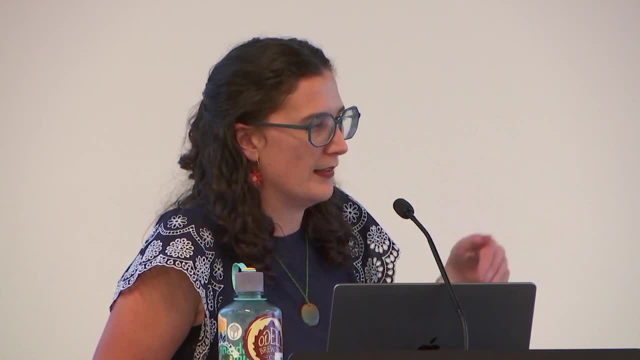 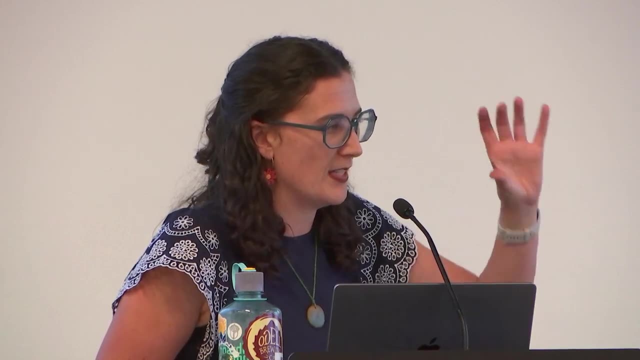 So the first one- I think I had three maps with like four-month lead times- And the second one: instead of using different lead times, I looked at different depths of ocean, heat content, anomaly, But at the same time, because the deeper you go in the ocean, the sort of longer you're. 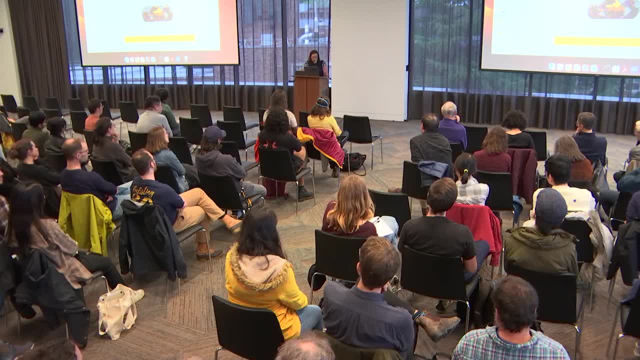 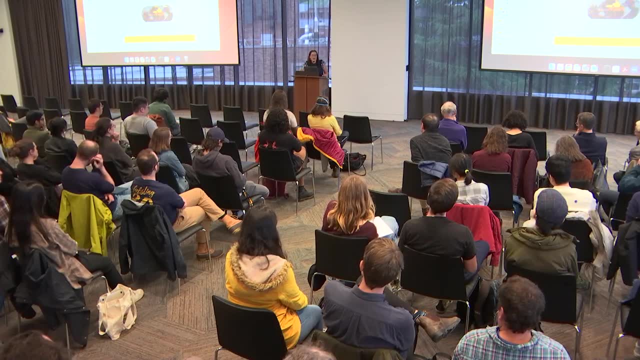 looking back in time And then, with this final study, I looked at giving it to the neural network to overlapping 10-year periods of sea surface temperatures. In some places this did improve the neural network scale and in some places it didn't. 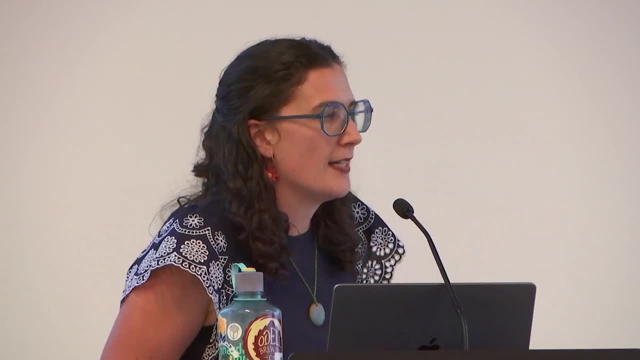 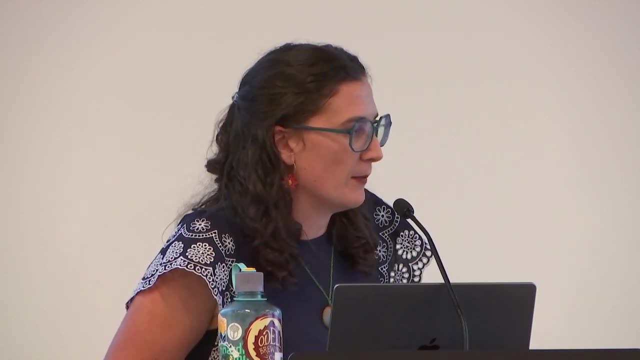 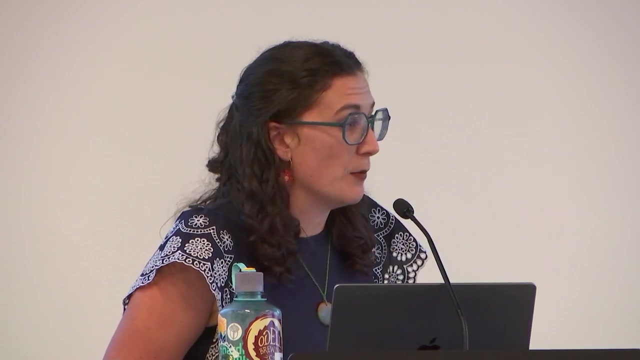 So, looking on, In the case of like training over all grid points, I think the models that I'm using are relatively simple, So I think I'm almost reaching the amount of skill you can get from a neural network of this complexity, But I like to think that there have been some pretty valuable insights from examining the 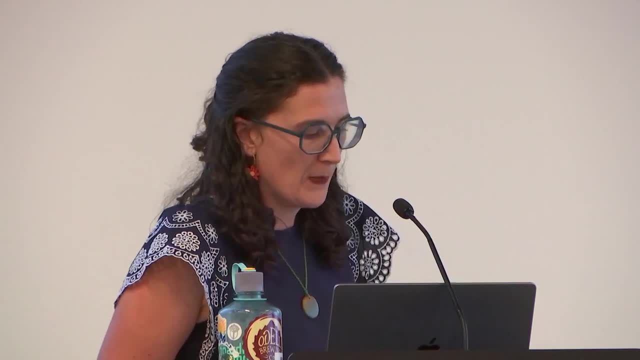 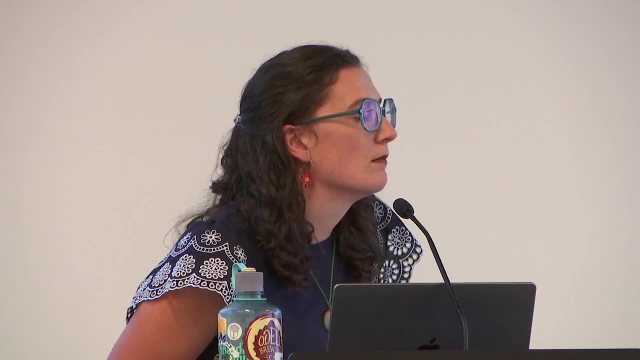 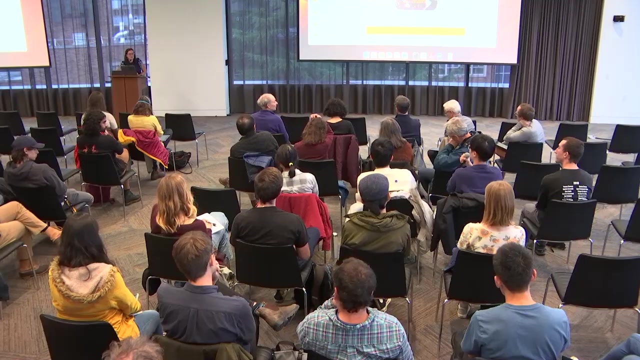 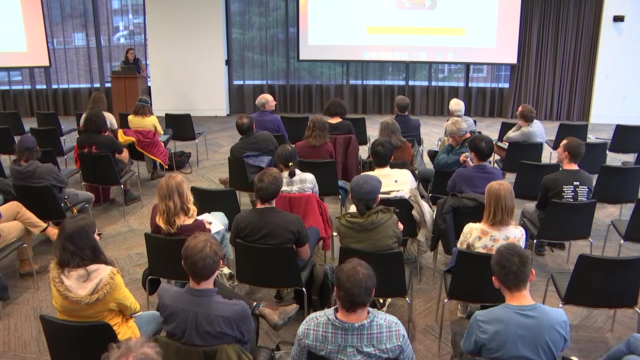 problem in a very simple way. I have some questions about how your experiment result, sensitivity to your model structure. I mean the, For most of your research uses fully connected network for prediction. So if you change to another, like self-tension network, how your model, how your result improved? 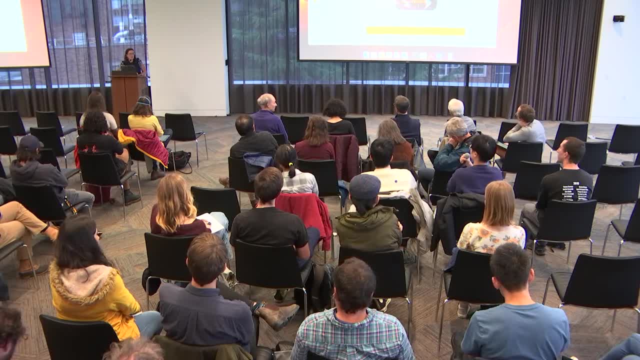 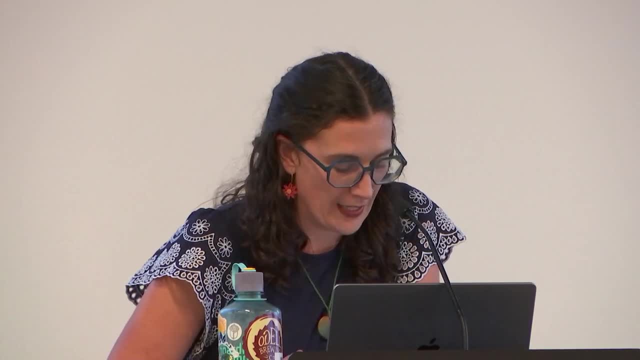 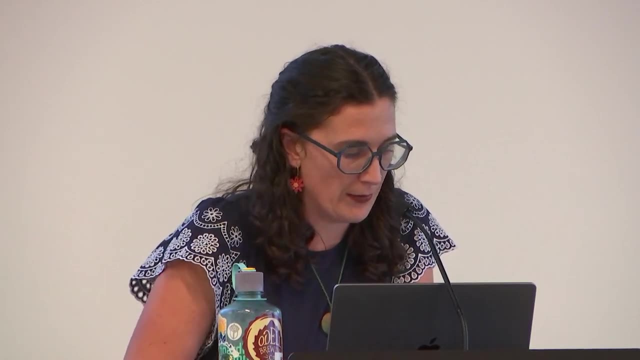 and how your signals maybe differs with this fully connected model? Yeah, so, like I think, similar to the previous question, I wanted to keep this as simple as possible. So, artificial neural- Well, using the fully connected artificial neural network as a way of doing this. 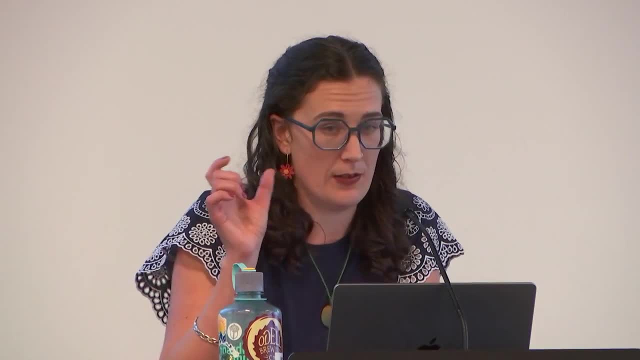 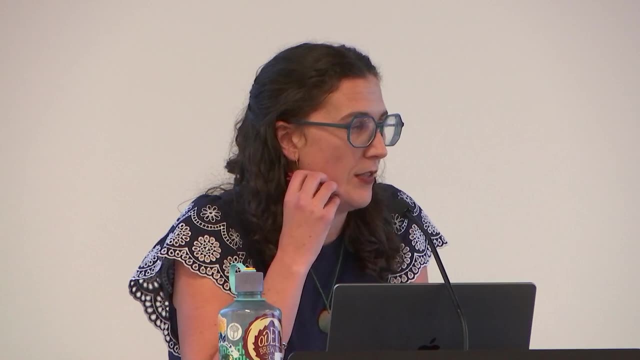 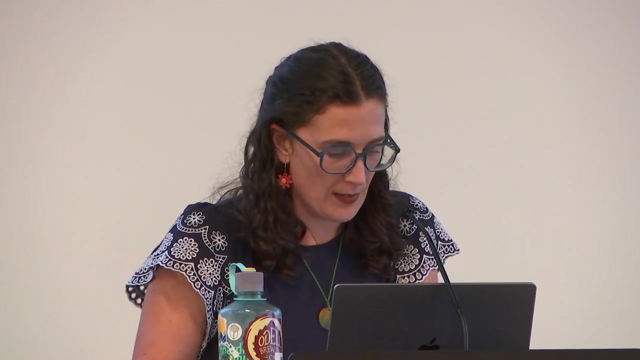 We found we didn't need to go into convolutional neural networks. So looking at sort of image-based- because using only one climate model, as I did here, you don't expect the sort of where the patterns are to change, So we don't need to like scan an image to find the patterns, for example. 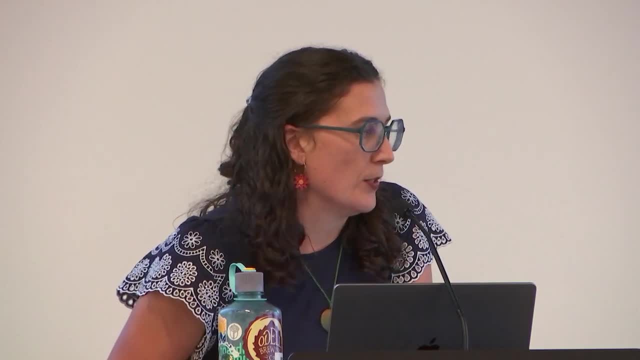 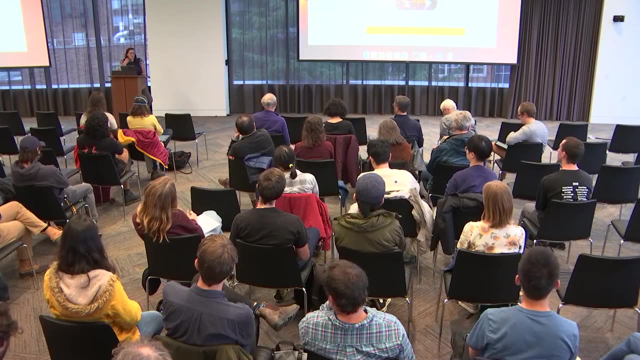 I'm interested now In moving away from using a single model, using multiple models, to learn sort of from each of the models. what can we learn about your system predictability? And I think that's when convolutional. I'm using those now because I think you need the ability to further the transformation. 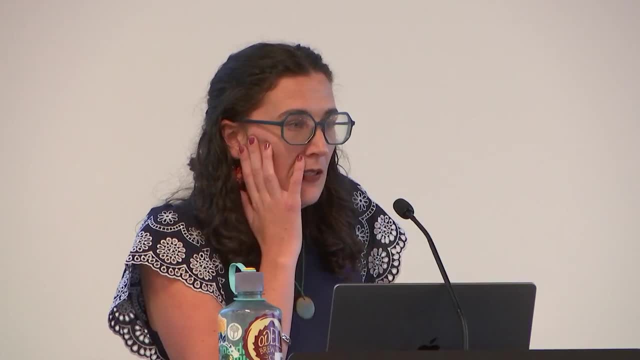 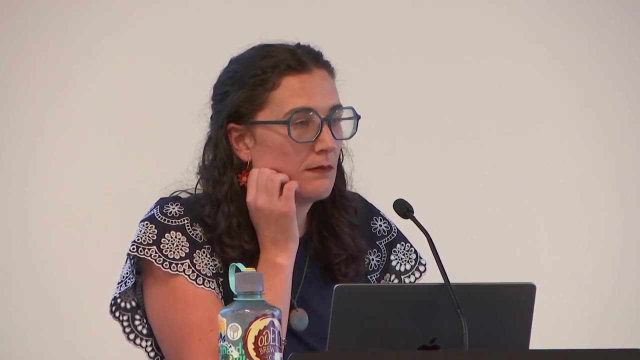 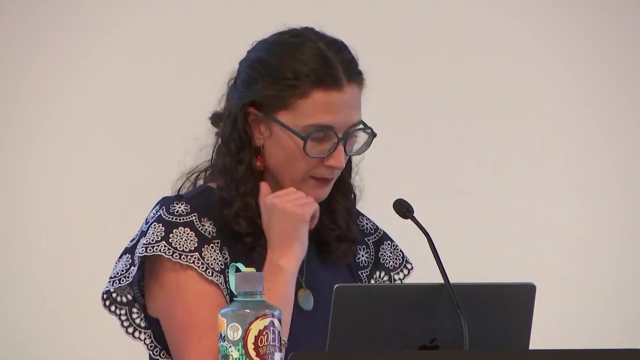 or translation. Thanks for the talk. I was curious about the method that you used early on to find the sort of important regions. As someone that doesn't really know anything about, I was just curious if you could explain sort of how that works to get sort of like the 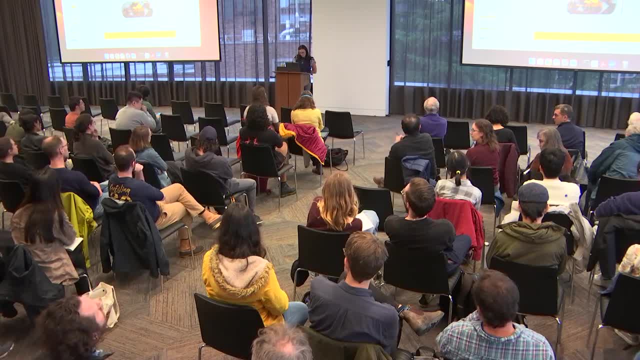 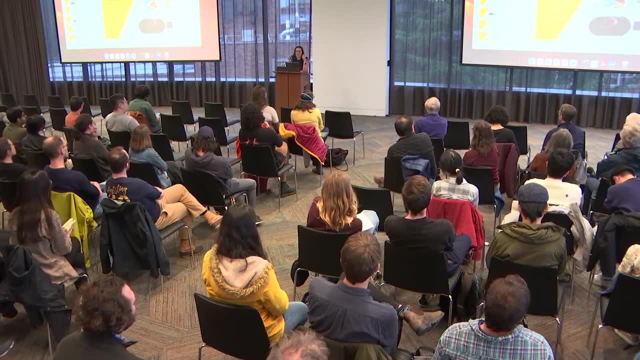 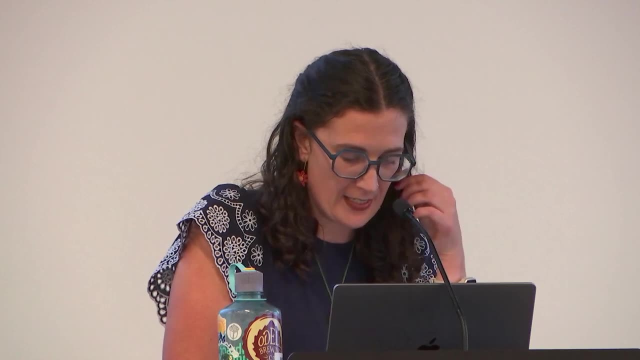 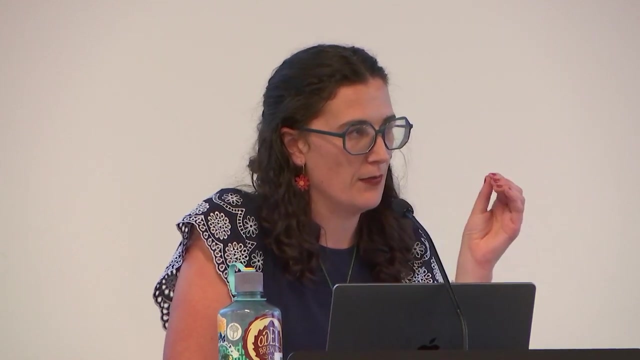 image with Horsham in the North Pacific. Yeah, So it's. This is called layer-wise relevance propagation, or LRP. In this case, it's the same as doing a method called input times gradient, which what you're doing is at each grid point you're testing the sensitivity of sort of a small perturbation. 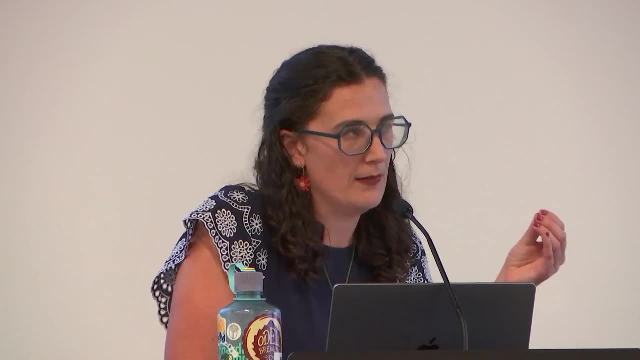 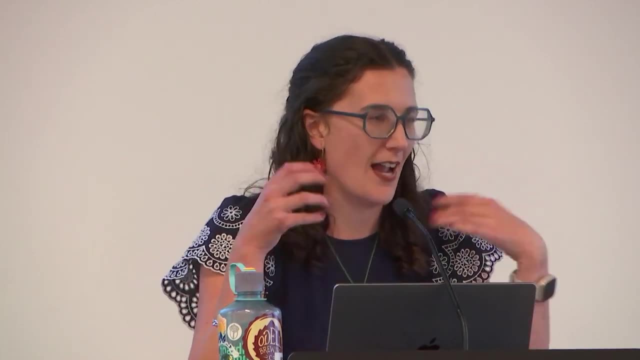 of the grid point to the output, the sensitivity of the output to small perturbations in each of the input grid points, and then you multiply it by the input mass, so you get like a. The sign sort of gets in the right place. 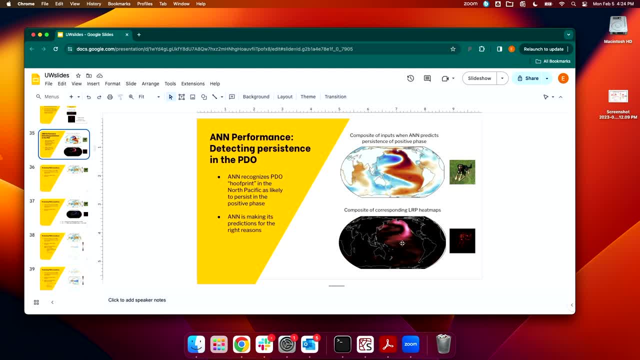 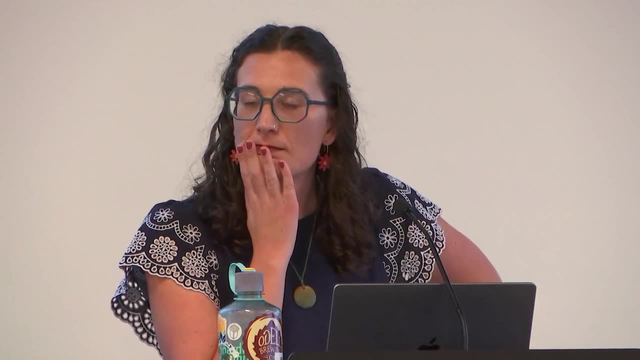 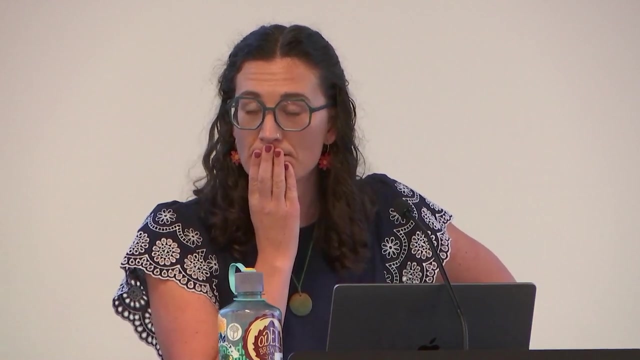 So this means that, Let me see, This means that positive perturbations in this region here result in a more positive prediction. here is sort of the way of thinking about it. Yeah, Your approach depends on using a GCM that we know has flaws, significant flaws especially. 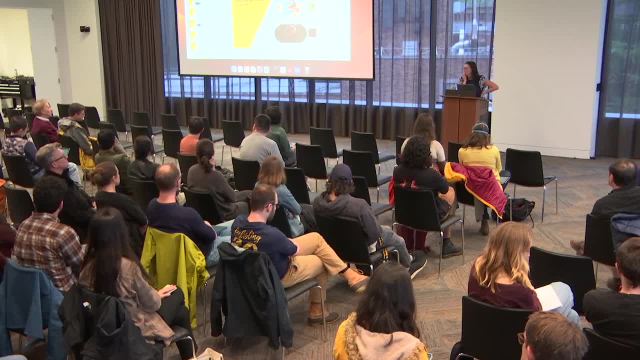 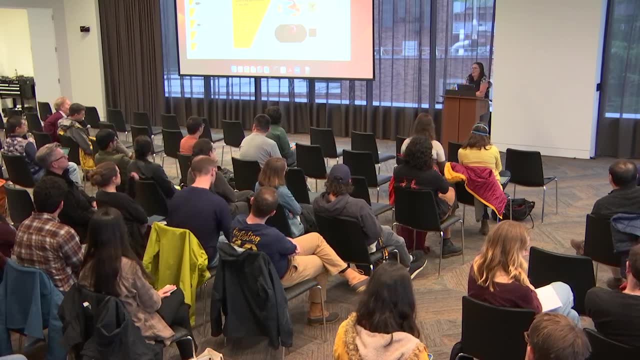 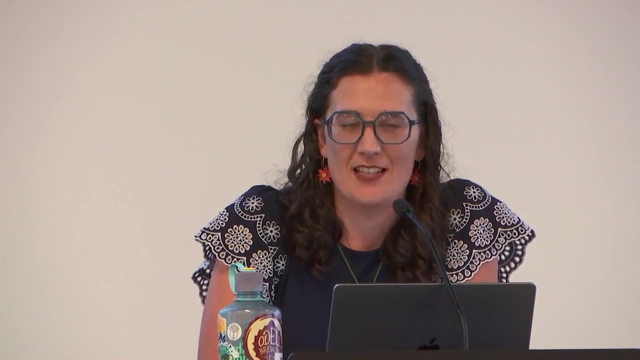 in terms of natural variability. So why do you think that you can use this approach to actually get skillful predictions in the real world? Yeah, I think that's a good question and I think it's. there's a lot of research, not my own. 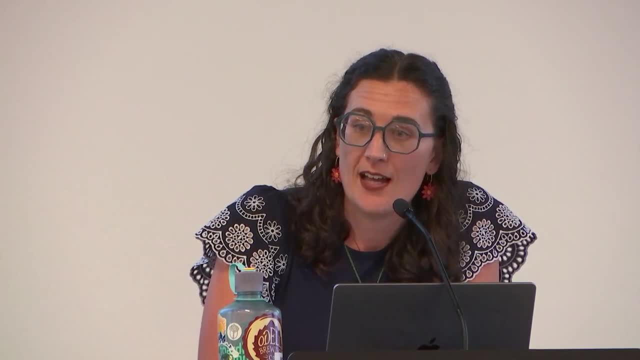 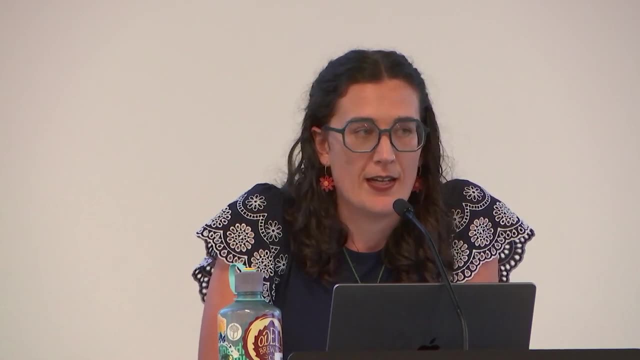 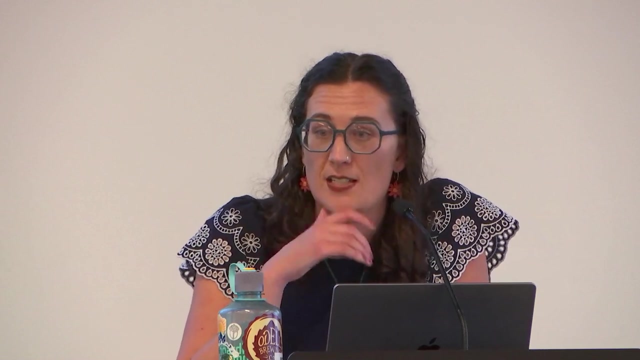 that shows, like It's just surprisingly, how good these models are at predicting the real world. and one thing I've found it actually is like training across. so I've been training across many different climate models now and then testing on observations, and we are able to get skill. 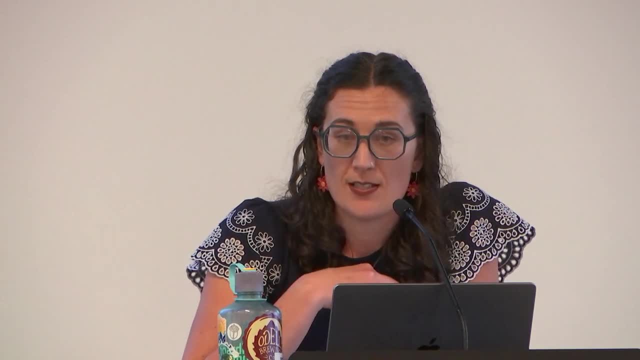 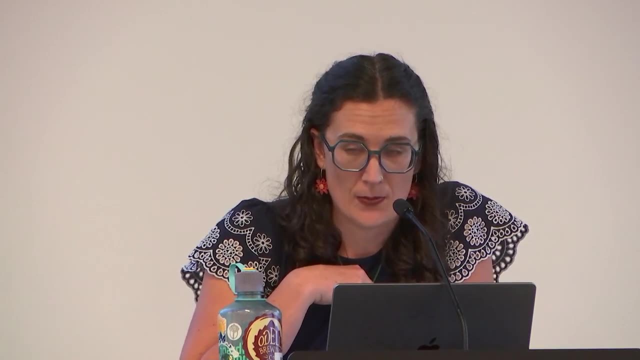 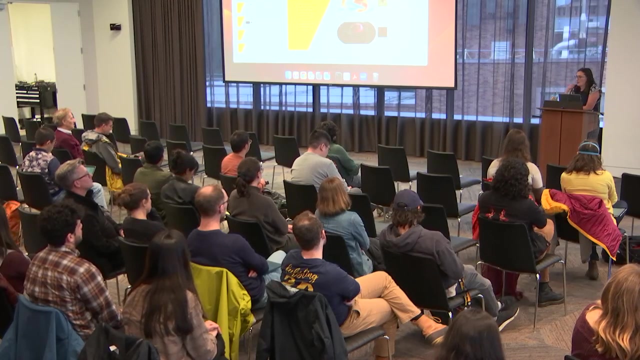 within the observational record of variability. So this is suggesting to me that I think this is a consequence of something called the signal-to-noise paradox, which is that, Yeah, observations actually have more of a signal of internal climate variability than the climate models do, and so the neural network's actually able to sort of learn enough of the 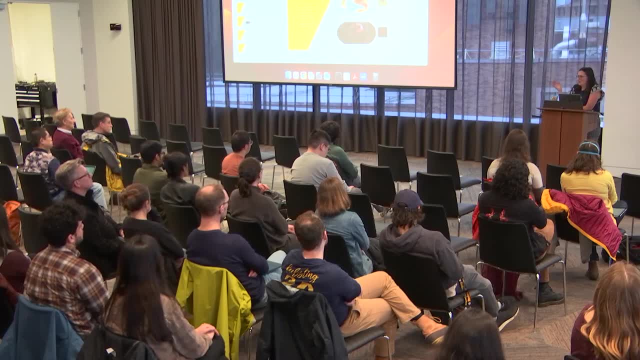 variability that when you test it on observation, it's sort of like: oh my goodness, there's actually more of a signal here to predict. All right, Let's thank the speaker one more time. Give him a hand, Thank you, Thank you. 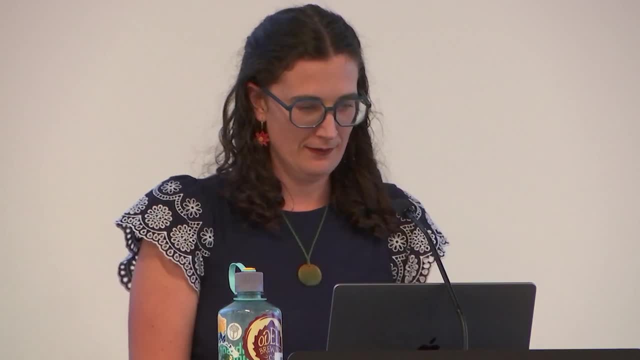 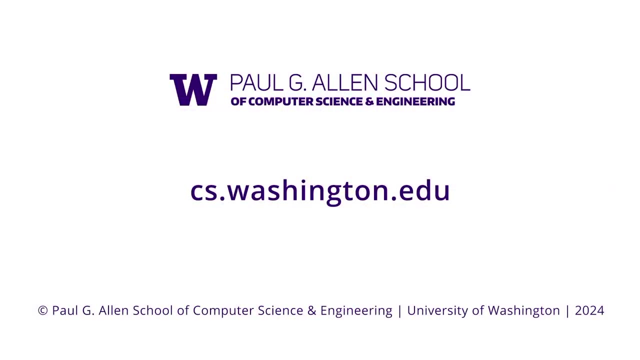